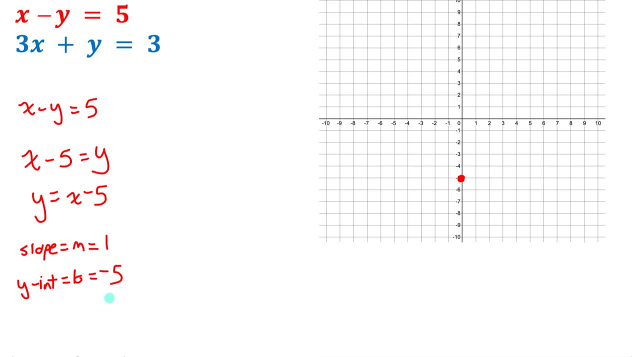 So we would plot the y intercept of negative 5, and then use the slope of 1.. Remember, slope is rise over runs. You may want to rewrite that whole number 1 as a fraction 1 over 1.. So rise 1, run 1, plot a point and keep plotting points. 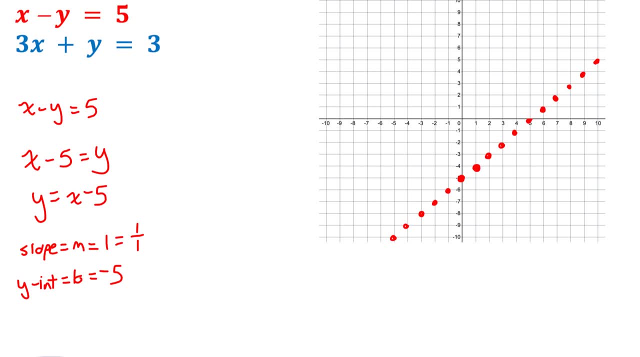 Until you fill the grid, And then we'll connect them with a straight line And we'll go through the same process for the other line. Let me isolate y. I'll just move the 3x term to the right. It becomes negative 3x. So it's clear that for 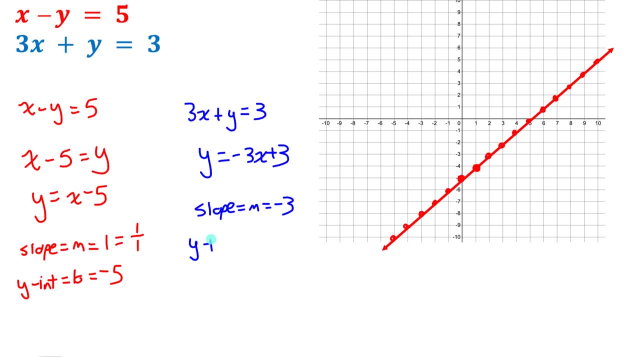 this one, the slope is negative 3. And the y intercept is 3.. Plot the y intercept And then use the slope And remember any whole number is over 1.. So you can think of this negative 3 as negative 3 over 1.. So rise negative 3, run 1.. That means down 3,, right 1. And keep plotting. 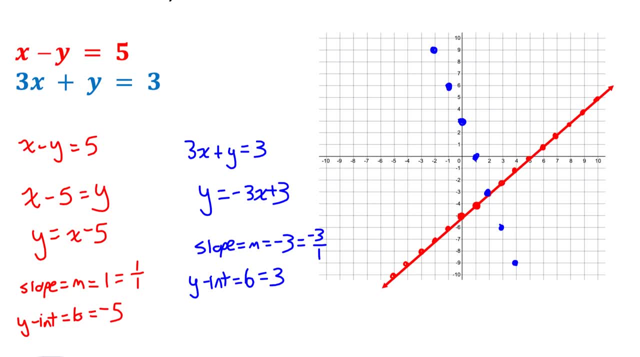 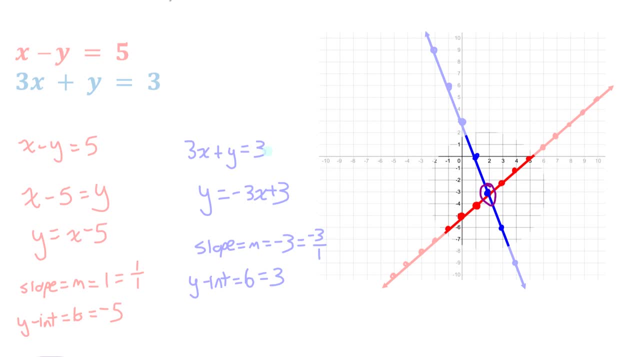 points Until you fill your grid, Connect them with a straight line And then just find where these lines intersect, And that's the solution to the system. These lines intersect right at that point. right there, the point 2, negative 3. That's our point of intersection, So we can say the solution. 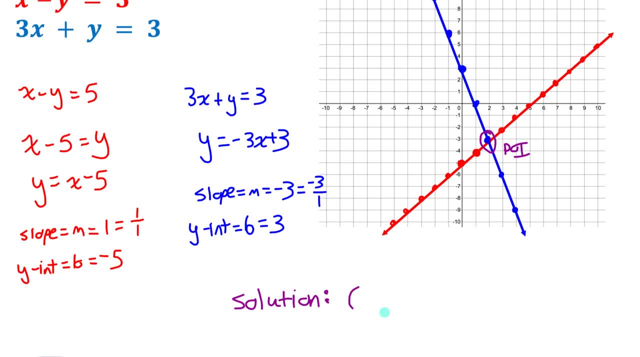 is. you could write it one of two ways. You could write it as a point: the point 2, negative 3.. Or you could write what x and y are equal to. You could write: x equals 2,, y equals negative 3.. 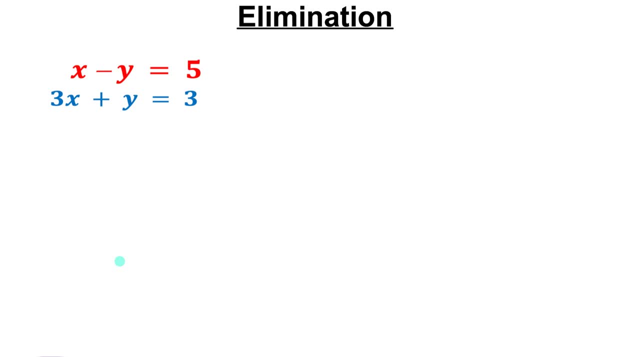 Either would be acceptable ways of writing the final answer. Let's solve that same system using elimination and substitution. Elimination first. So in doing elimination you want the equations in the format: x plus y equals the constant which both equations are already in. 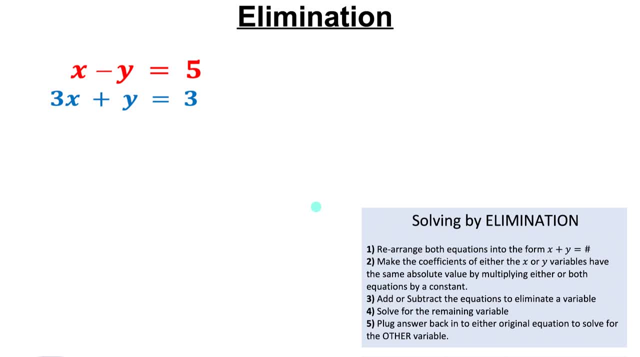 that format. Now, our goal here is to eliminate a variable, And the way we do that is by making the coefficients of either the x's or the y's have the same absolute value. Now, in this example, the coefficients of the y's already have the same absolute value. 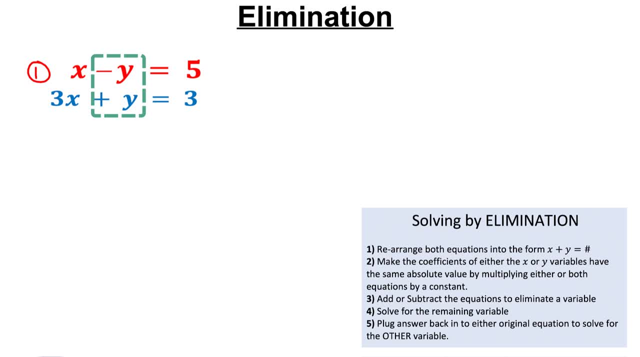 The coefficient of y in the first equation is negative 1, and the coefficient of y in the second equation is positive 1.. Those have the same absolute value But because they're opposite signs, adding the equations will make them eliminate. If they were the same sign subtracting. 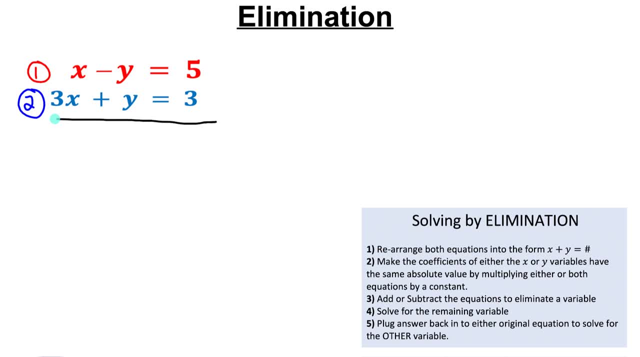 them would make them eliminate. But in this case, since they're the same absolute value, but opposite signs, if we add these two equations together, the y's will eliminate. Watch, Let's add the equations. And when we add the equations, we make sure we collect the like terms. That's why we have 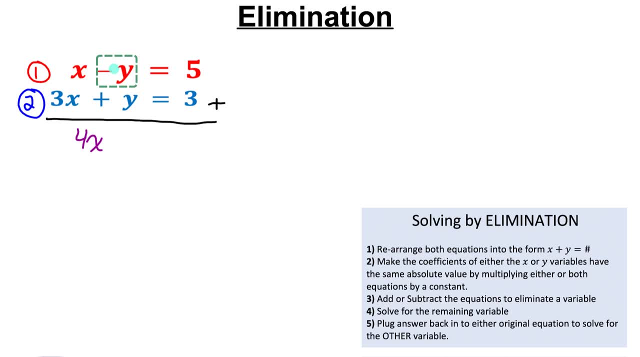 x plus 3x is 4x. Negative. y plus y is 0, that they eliminate, which is what we want, And 5 plus 3 is 8. So we have 4x equals 8. Divide both sides by 4. We get x equals 2. So we have the value of x. 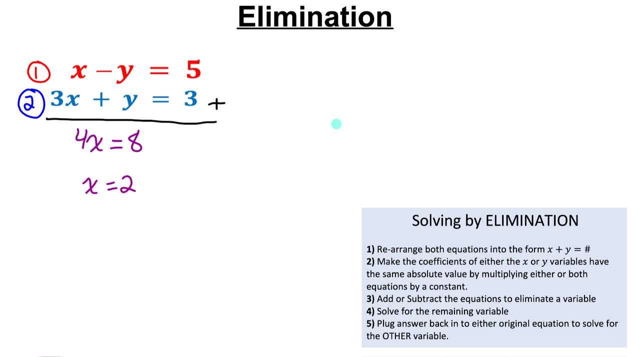 that make both equations the same. But what's the value of y? We now need to sub x equals 2 into either of the original equations. It doesn't matter which one you plug it into, because that's the value of x that makes both equations have the same value of y. So we have x equals 2, and we 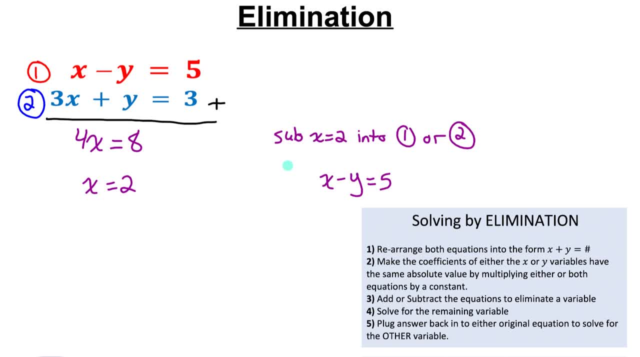 have negative y, I'll choose the first one. It looks easier. So sub 2 in for x. 2 minus y equals 5.. I'll isolate y, move the negative y to the right, move the 5 to the left. I've got 2 minus. 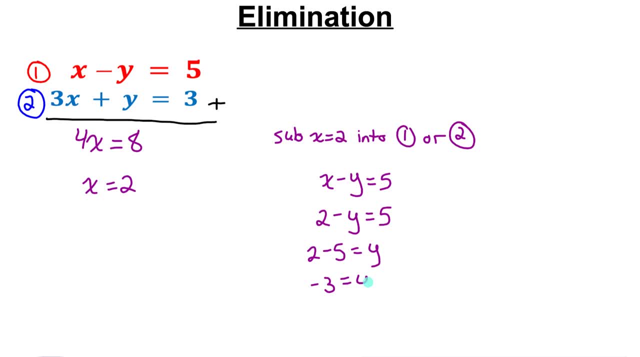 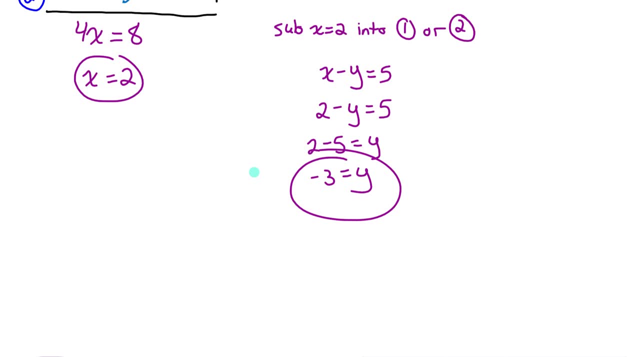 5 equals y, Negative 3 equals y. So notice my solution: x equals 2,, y equals negative 3.. That's the same thing we got by solving it graphically. Let's try it again, but using substitution. Now, when doing substitution, I often like to line them up side by side, like this: I'll. 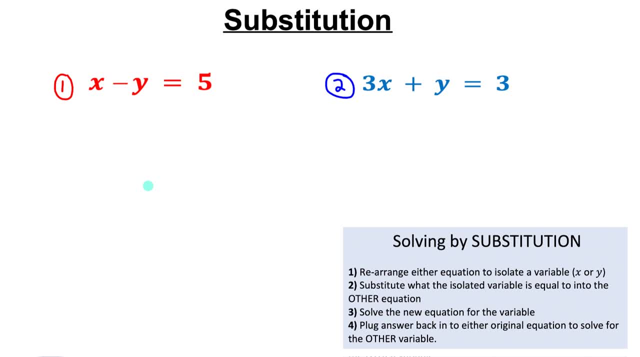 do this with two equations, equation one and equation two. When doing substitution, what you want to do is isolate one of the variables in either of the equations. Doesn't matter, I think in equation one the variable x looks like it would be easy to isolate since it already has. 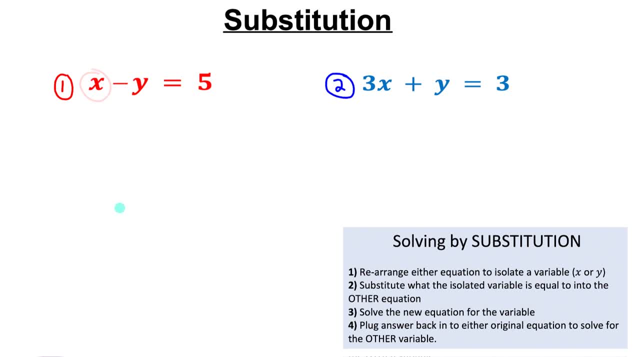 a coefficient of 1.. So I'll pick this x to be the variable that I'm going to isolate. So I'll move this negative y to the right and it becomes positive y. So I have: x equals 5 plus y. Now what? 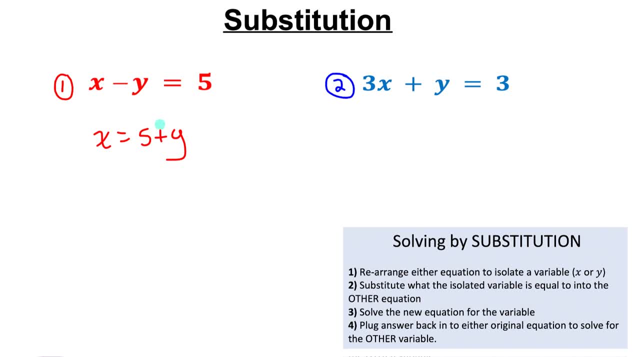 the variable you isolated is equal to. so it says x equals 5 plus y. you take that and plug it into the other equation for x, because we know x is equal to 5 plus y. So now in the other equation I have 3 times 5 plus y plus y equals 3.. Now we have an equation with only one variable, This 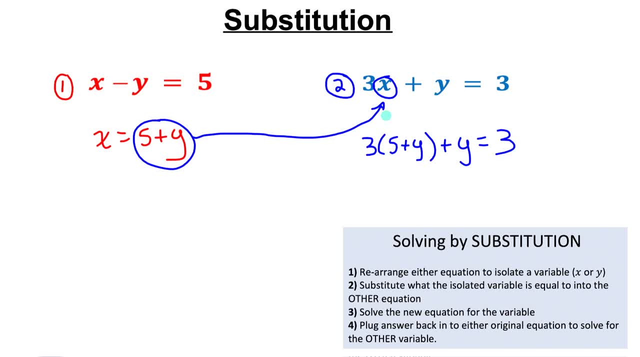 equation only has the variable y. We could solve this for y. Let me distribute the 3 into the brackets. collect my like terms. I've got 5 plus y and I've got 5 plus y. So I've got 5 plus y. 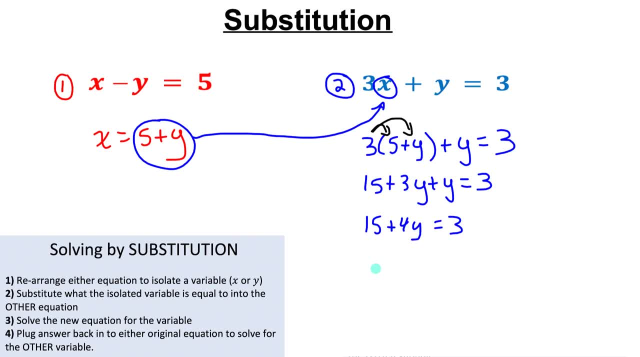 and I've got 15 plus 4y equals 3.. Now I want to isolate the y, so I'll move the 15 over. 4y equals 3 minus 15, which is negative 12. Divide both sides by 4. I get y equals negative 3. I now need 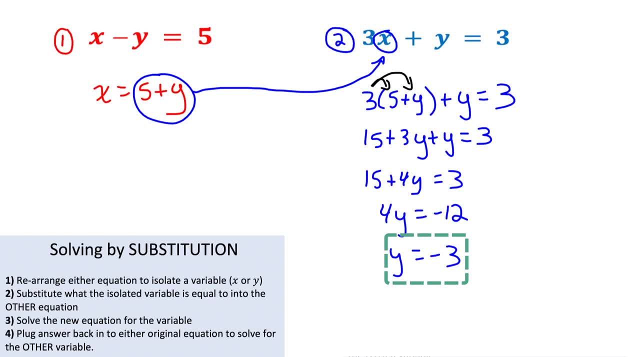 to solve for the other variable. So what we have to do is take that answer and plug it back into either of the original equations. It's always easiest if you sub it back into this rearranged version we have, because x is isolated. So you just take this answer for y, we got, plug it back. 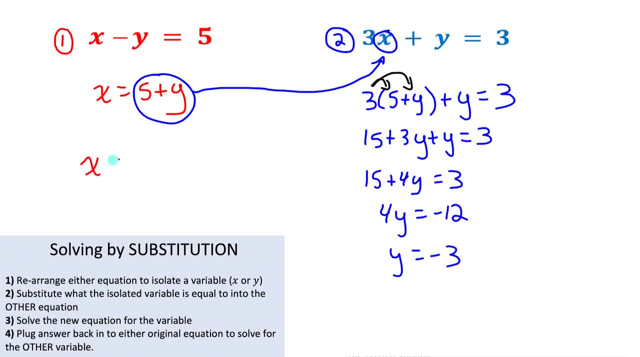 in for y there and then we get our answer For x. so I'd have x equals 5 plus y, which we know is negative 3.. So I have x equals 5 plus negative 3,, that's 5 minus 3, which is 2.. So I got x equals 2, y equals negative 3.. Same answer again. 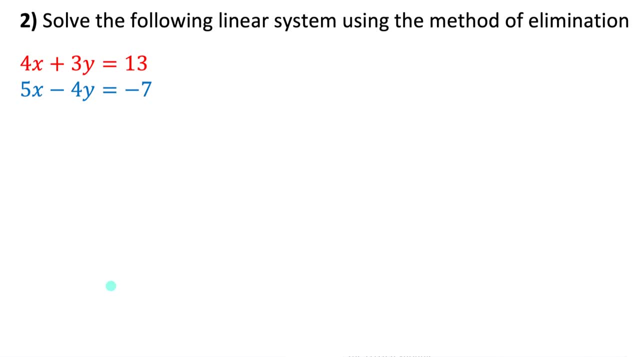 just a different method. Example 2, solve the Fong linear system using elimination. So this one's much harder than the first one. we did For this one we have two equations again, and both equations are already in the proper format, with x and y on one side of the equation and the constant on the. 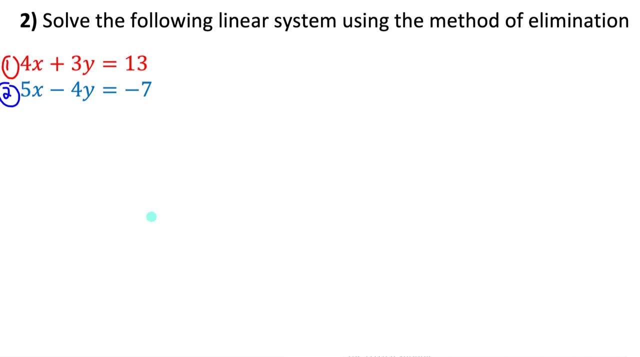 other side. But we want to eliminate the Fong linear system using elimination. So we want to eliminate the variables by adding or subtracting the equations and to do that the coefficients have to have the same absolute value. And notice the x's have different coefficients and the y's 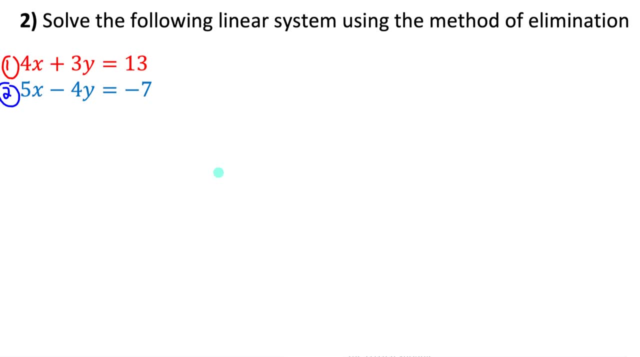 have different coefficients. So what we're going to have to do is multiply one or both of the equations by a constant to make the coefficients have the same absolute value. What sticks out to me is we can make the x's have a coefficient of 20, or we can make the y's have a coefficient of. 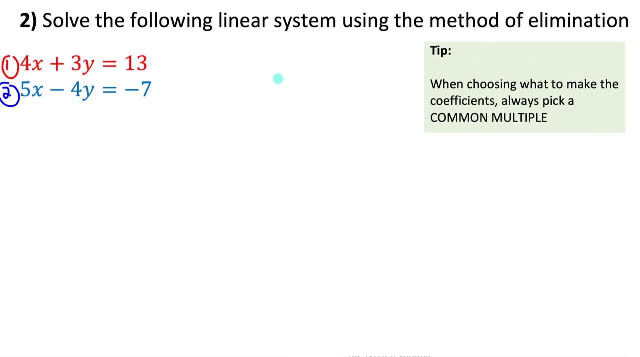 12 and negative 12.. Doesn't matter, Let's make the x's both have a coefficient of 20.. So I would have to multiply equation 1 by 2, and then I would have to make the x's have a coefficient of 20,. 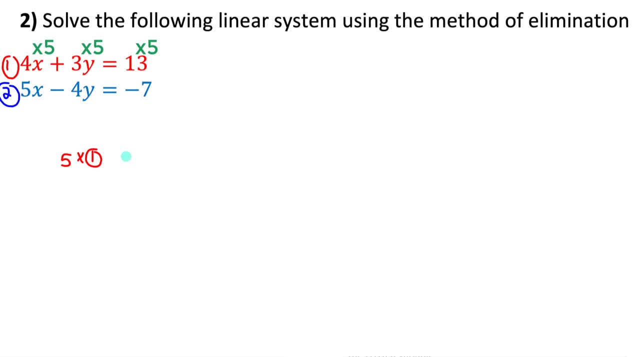 by 5.. So I'm going to do 5 times equation 1, and that would give me: so 5 times 4x is 20x, 5 times 3y is 15y and 5 times 13 is 65.. Make sure you multiply every term in the equation by the. 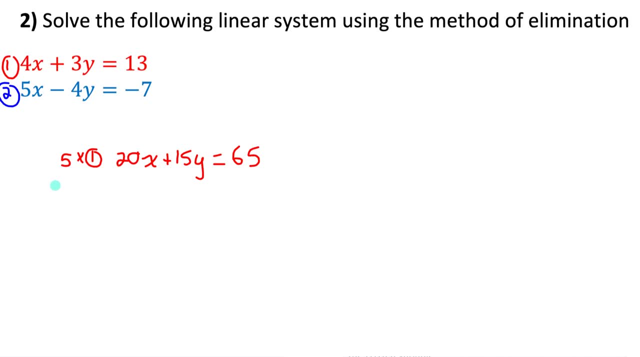 constant. And for the second equation, for the x to have a coefficient of 20, I'd have to multiply it by 4, so 4 times equation 2. And that would give me 20x, 4 times negative. 4y is negative 16y. 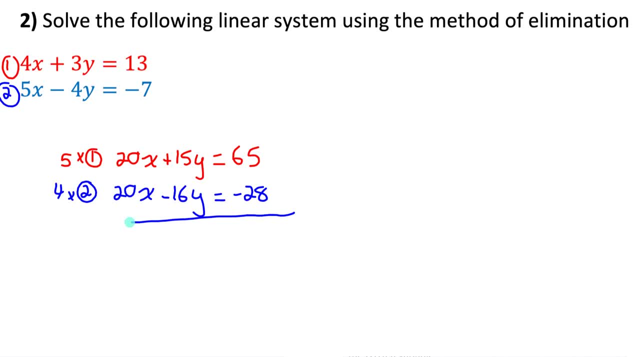 and 4 times negative. 7 is negative 28.. Now what I'm going to do is I'm going to figure out should I add or subtract these to eliminate the variable. The x's have the exact same coefficient with the exact same sign: They're both positive 20.. So subtracting will eliminate the variable x. So let's subtract. 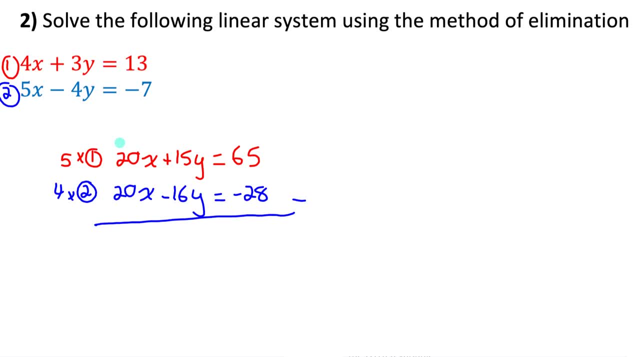 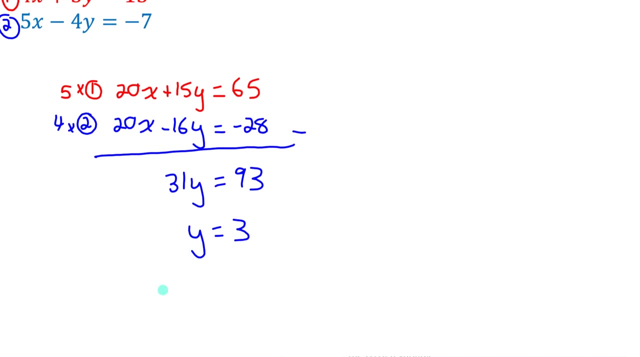 all the like terms. 20x minus 20x is 0x. so that's gone. It eliminates 15y minus negative, 16y is 31y and 65 minus negative, 28 is 93. Divide both sides by 31, and we get y equals 3.. Now we need to sub y equals 3 into either. 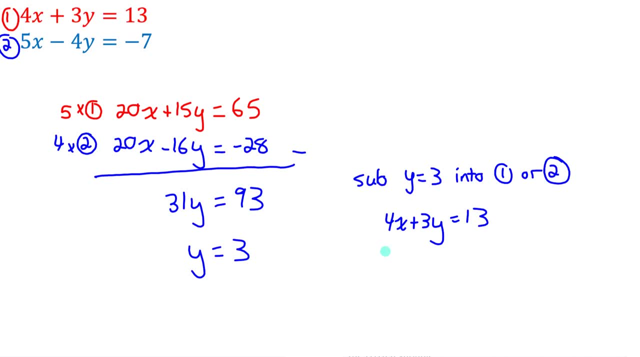 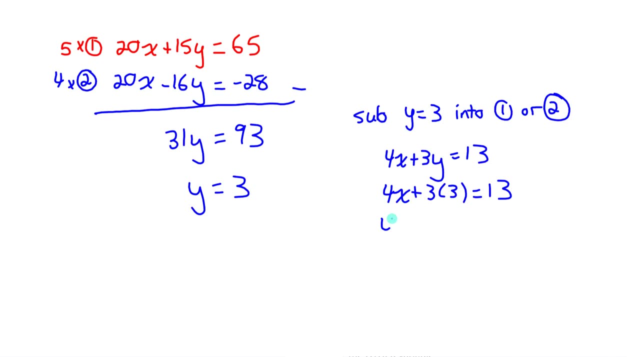 original equation, So I'll just sub it into equation 1.. Let's sub our answer for y into that equation. So 3 times 3 equals 13, and then we just solve this for x. So 4x plus 9 equals 13.. 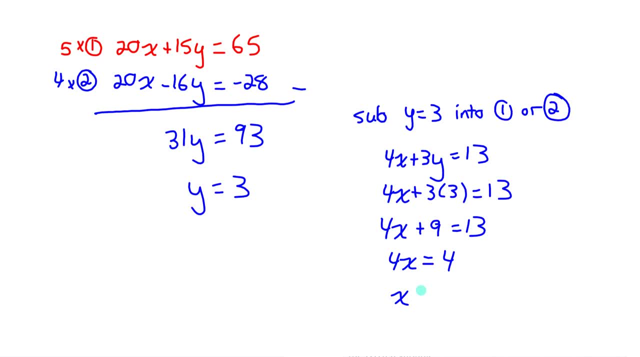 Let's subtract the 9 to the other side, I get 4x equals 4.. Therefore, x must equal 1.. So my solution to this linear system is: x equals 1, y equals 3.. If we were to graph both lines, they would intersect at the point 1, 3.. 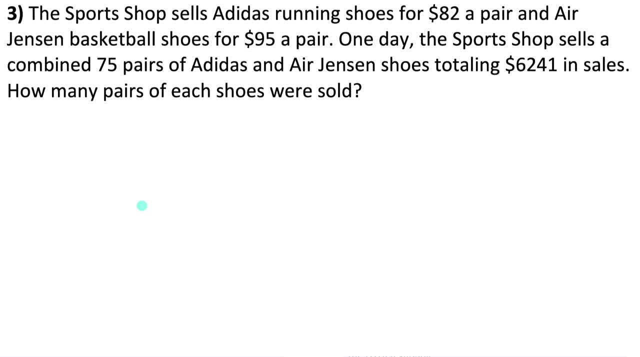 Example 3.. Here's an application of solving linear systems. A sports shop sells Adidas shoes for $82 a pair and Air Jensen basketball shoes for $95 a pair. One day, the shop sells a combined 75 pairs of shoes totaling $6,241 in sales. How many pairs of each shoes were sold? Now for these types and 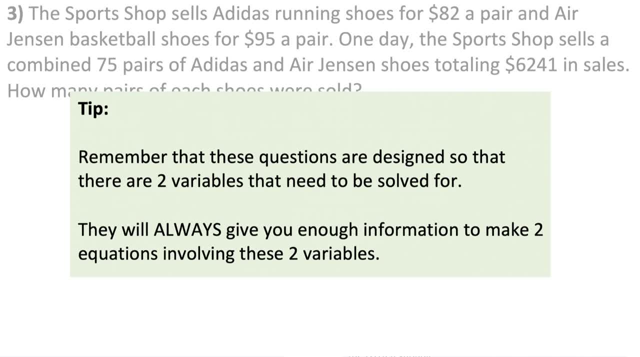 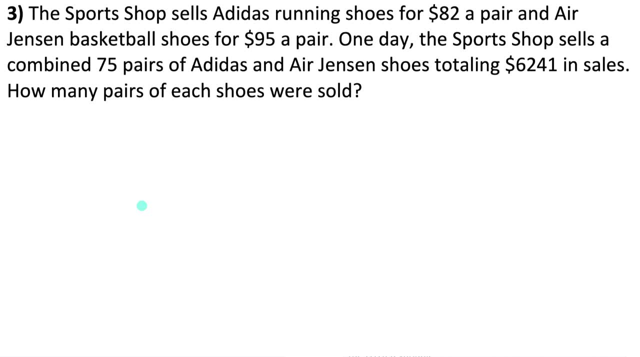 questions. they're always going to want you to solve for two variables. And in order to solve for two variables, you must be able to make two equations. So let's do that, So, let's do that. So I always like to start by figuring: okay, what variables am I going to be trying to solve for? 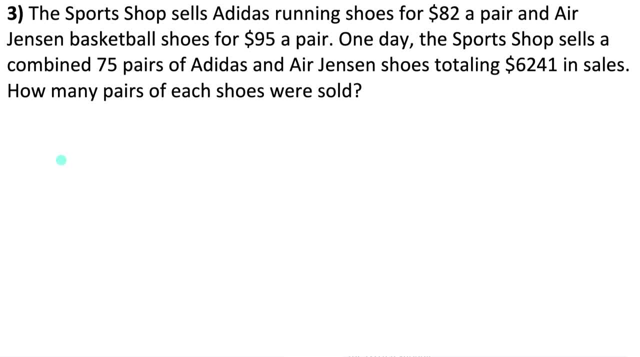 So it wants to know how many pairs of each shoe were sold. So we're trying to figure out, okay, how many Adidas shoes were sold and how many Air Jensen shoes were sold. Those are my variables. I'll say x equals number of Adidas and y equals number of Air Jensen. And in order to figure out, 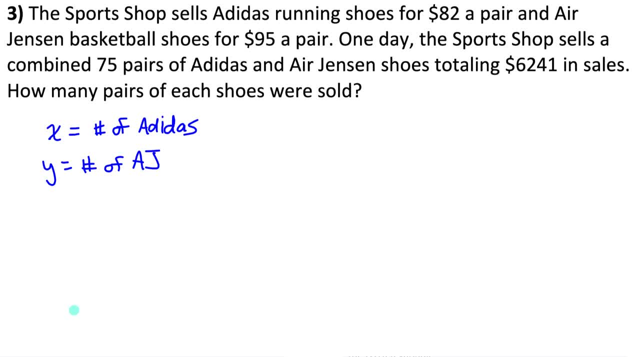 what the value of these variables are. I must be able to make two equations that involve these two variables. Well, I know they sold a combined 75 pairs of shoes. So my first equation: x plus y equals 75.. There's one equation that involves x and y In the second equation. well, I know what. 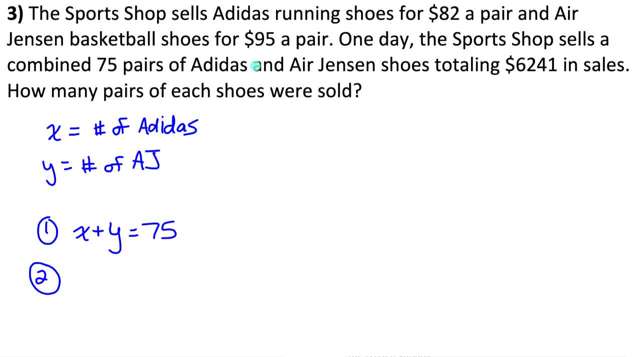 the total dollar amount in sales was- And I know how much each pair costs- Adidas shoes cost $82 a pair. So 82 times the number of Adidas sold plus Air Jensen's cost $95.. So 95 times the number of Air Jensen sold would equal that $6,241.. When you have two equations with two variables. 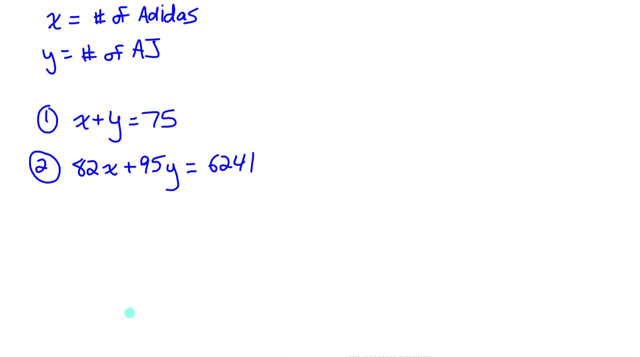 you can solve them by graphing substitution or elimination. I think I'll do elimination. for this. Let me make the coefficients of the x's be the same. So I'll multiply the first equation by 82. And that would give me 82x plus 82y, And 82 times 75 is $61.50.. 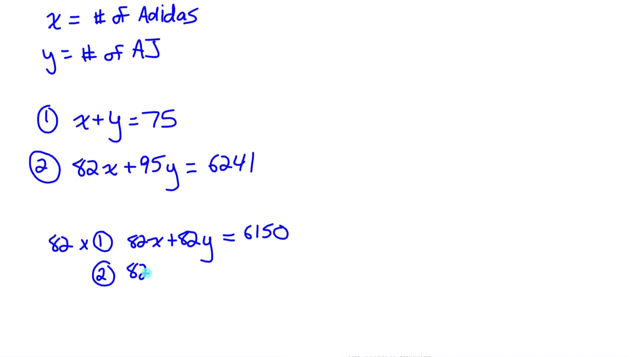 Now let me rewrite equation two, lined up with that right underneath of it, And since the coefficients of the x have the exact same sign, I know subtracting will eliminate the variable. 82x minus 82x is zero, 82y minus 95y is negative 13y, And 61.50 minus 62.41 is negative 91.. Now if I divide both sides, 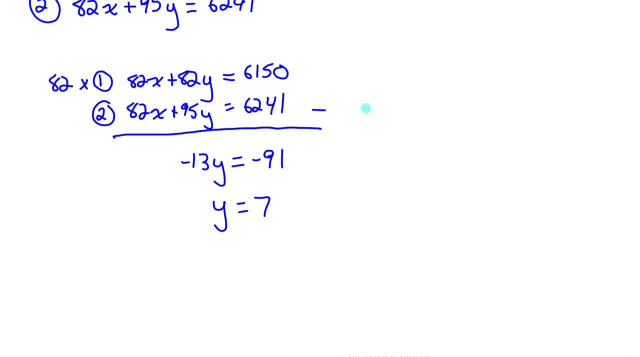 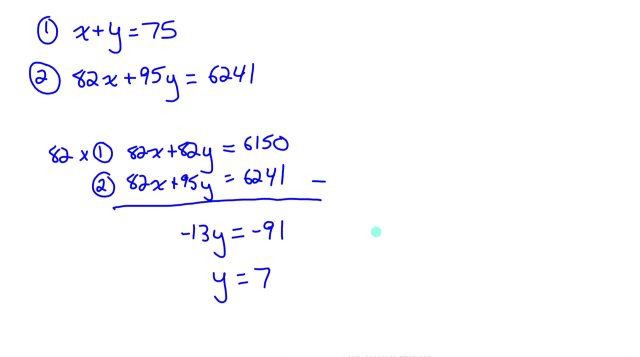 by negative 13,, I get y equals 7.. So I know that they sold seven pairs of Air Jensen shoes. Let me just sub that answer back into either of the original equations. Let me sub it back into one- That's going to be a lot easier- And then solve for x. So I'll sub 7 in for y. Therefore, 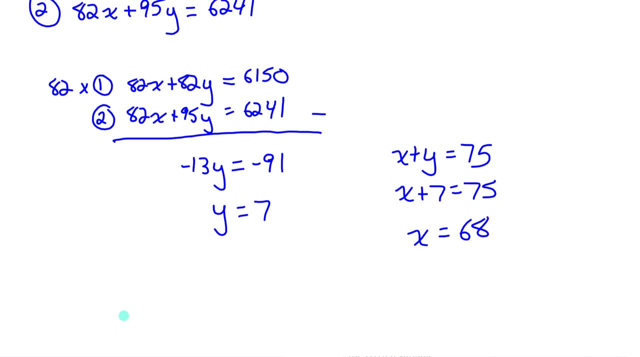 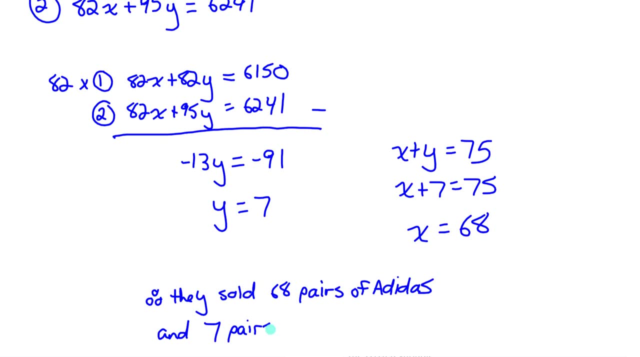 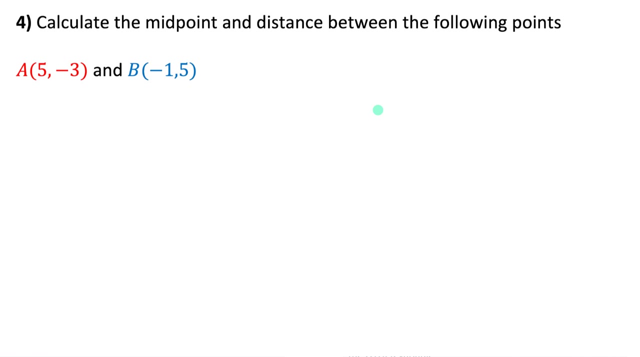 x is 68. So our final answer for this: they sold 68 pairs of Adidas and seven pairs of Air Jensen. Next, you need to know how to calculate the midpoint and distance of a line that connects two points. So I've got point A and point B. it says: calculate the midpoint and the distance. 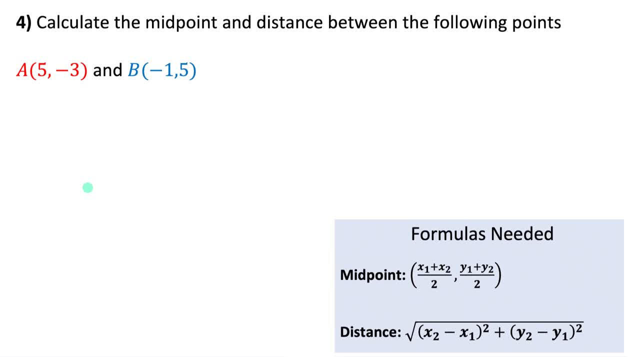 between those points. Let's start with midpoint. If you notice the formula, it says we need the x and y coordinates from our first and our second point. Now it doesn't matter which your first point is and which your second point is, but it's helpful to pick one and label it. So I'll make A. 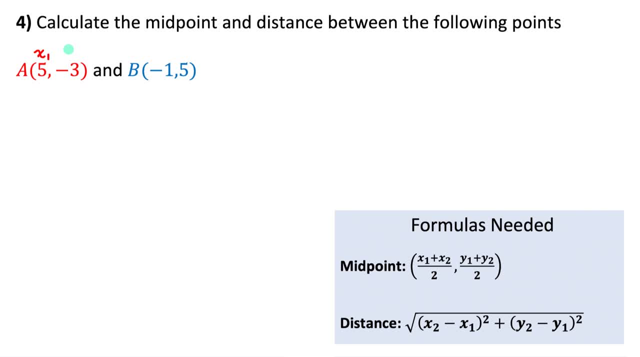 my first point, which means five is my xy, And then I'll add the second point. So I'll add the first point and negative three is my y one. It'll make B my second point, which means this is my x two and this is my y two. right, Each point has an x and a y. If I want the midpoint between these, 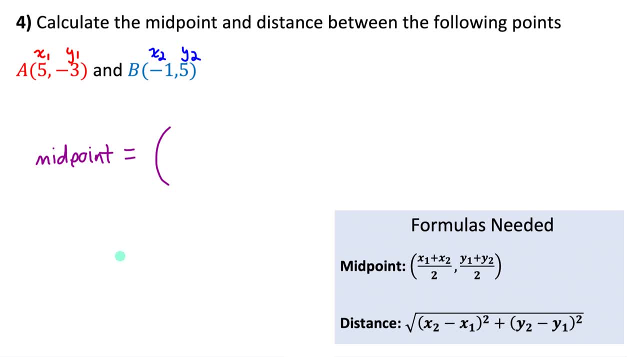 two. using the formula, it tells me that what I need to do is average the x coordinates. So I'll add x one and x two together, So I'll do five plus negative one, And then I have to divide it in two to get the average of the two of them right. the middle of the two points is going to be at the. 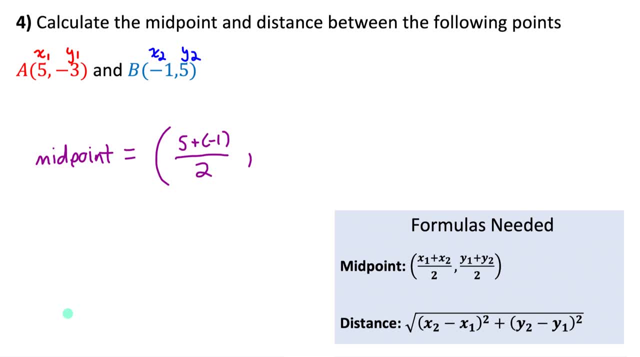 average of the x coordinates and the average of the y coordinates. So I'll do five plus negative one. So I now need to average the y coordinates by adding them and dividing by two. So negative three plus five divided by two and the midpoint. if I simplify this, the x coordinate: five plus negative. 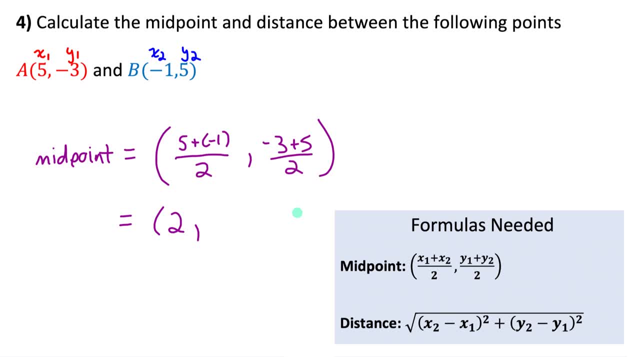 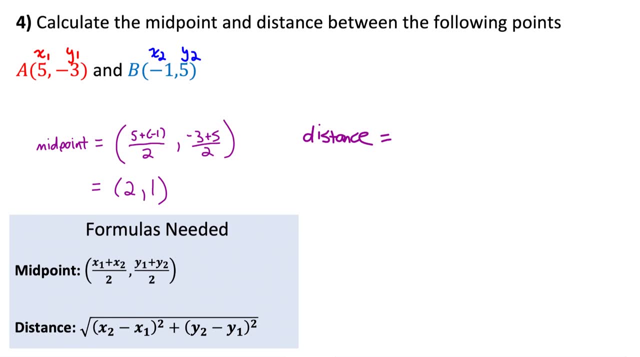 one over two, that's four over two, which is two, and the y coordinate negative. three plus five is two. divided by two is one. Let's now find the distance between point A and B. The distance formula comes from Pythagorean theorem. To find the distance, I do the square root of the difference. 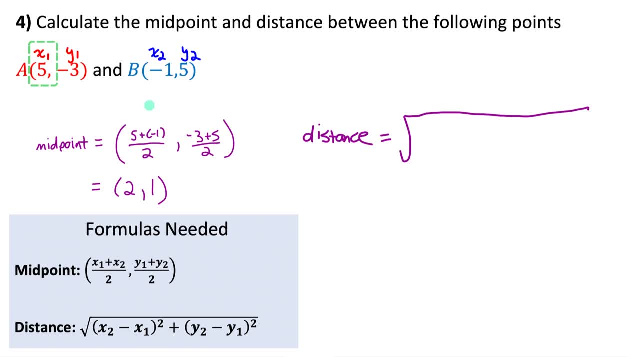 in the x coordinates. So the formula tells me to do x two minus x one and then square it. So negative one minus five squared plus the difference in the y coordinates. So now I have to do y two minus y one, so five minus negative three, and then square. 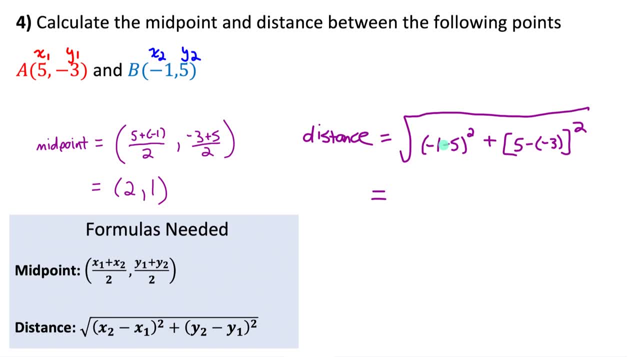 that difference And I just have to simplify this. So negative one minus five is negative six square it, and I get 36.. Five minus negative three is eight square it, and I get 64.. So I need the square root of 36 plus 64.. That's the. 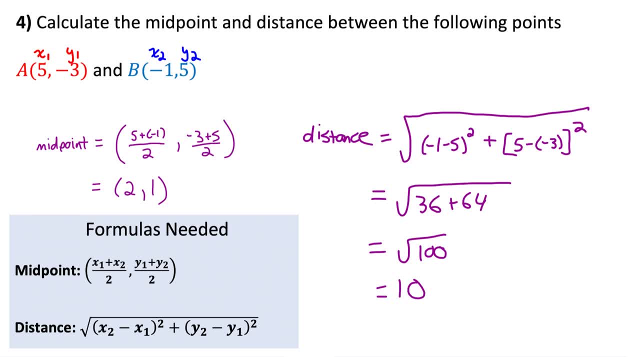 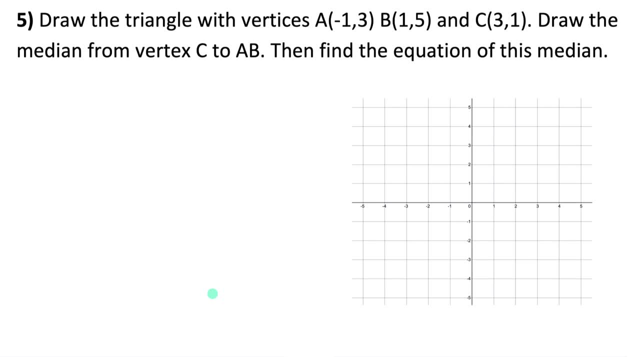 square root of 100, which is 10.. So the distance between the two points is 10 units. I don't know what the units are, but that's the distance between the two points. Example five says: draw the triangle with these vertices. So let me start by plotting those vertices. So there's my triangle. it says: 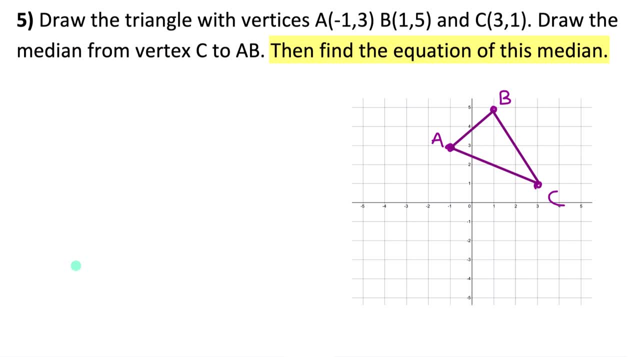 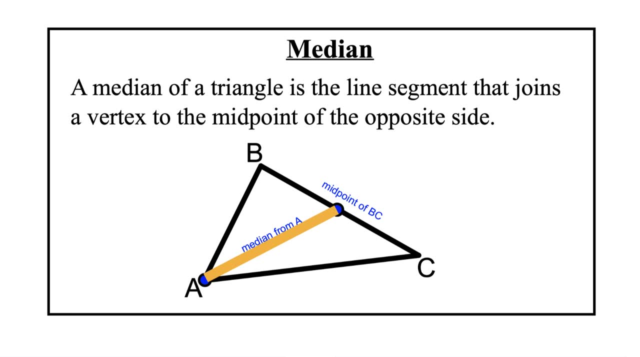 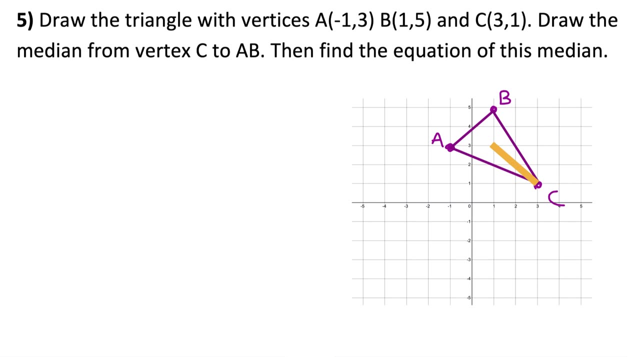 draw the median from C to AB, then find the equation of this median. Remember, a median of a triangle is the line segment that joins a vertex to the midpoint of the opposite side. So the median from C to AB would be the line that goes from C to the middle of AB. So let me just estimate. 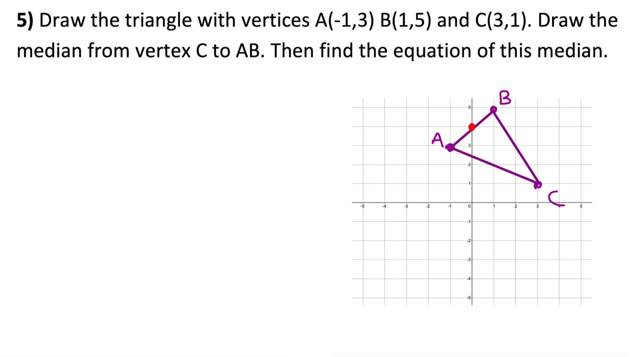 where that is right. here it looks like it's going to be about there. That's the middle of AB. So the median would go from C to that point. So what I've drawn in red is the median. Let's find the equation of that line in the form: y equals MX plus B. So I'm going to need to know its slope and y. 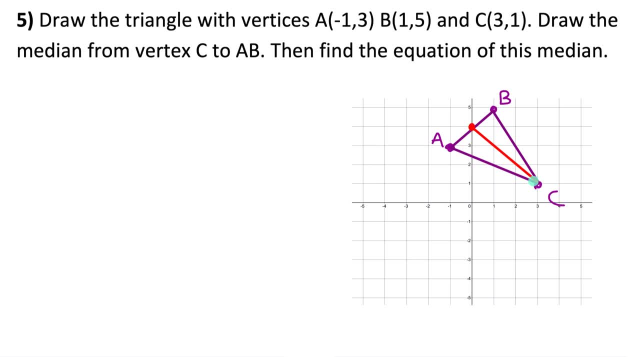 intercept. Let's start by figuring out its slope. And to figure out its slope, I would need to know its point C, And it's also at the midpoint of AB. Okay, so I'm going to need to know the midpoint of AB. Let's find the midpoint. So, the midpoint of AB. I'm going to need to average the x coordinates. 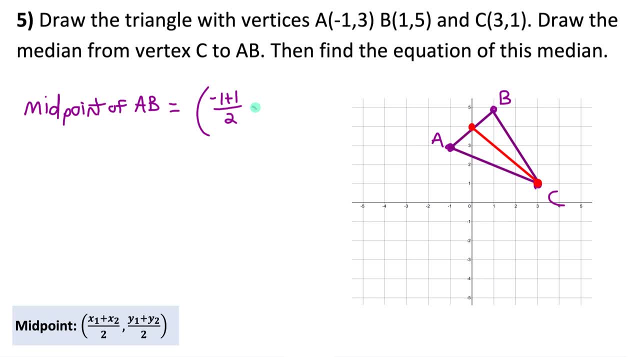 So negative. one plus one, divided by two and average the y coordinates three plus five over two, So the midpoint is going to be negative. one plus one is zero, So zero over two is zero, And eight over two is four, So my midpoint is zero four. 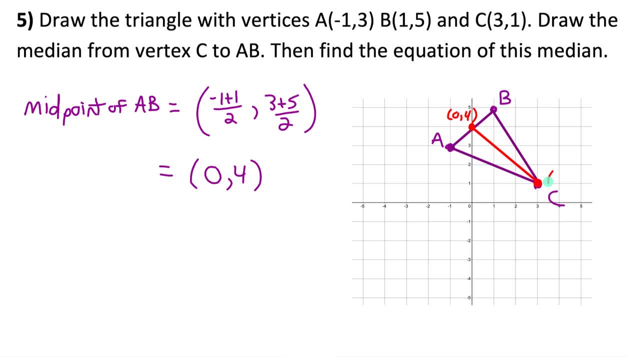 And I know point C is on the median as well, which the question tells us is the point three one. I could use those two points to find the slope of that median. I'll call the slope M and remember to calculate slope. you just do change in y over, change in x, y, two minus y, one over x, two minus x. 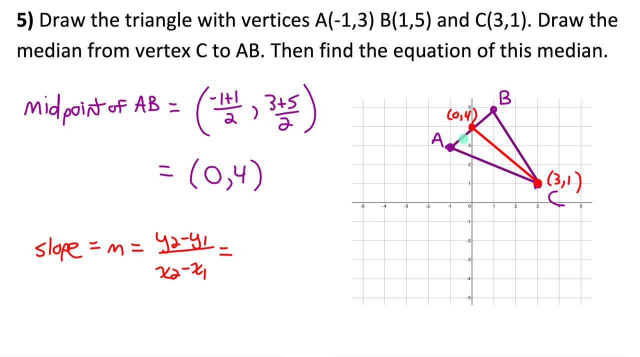 one. So I'll make C my second point and the midpoint of AB my first point. So one minus four over three minus zero And that gives me negative three over three, which is negative one. So the slope of my median is negative one. If I want the y intercept of the 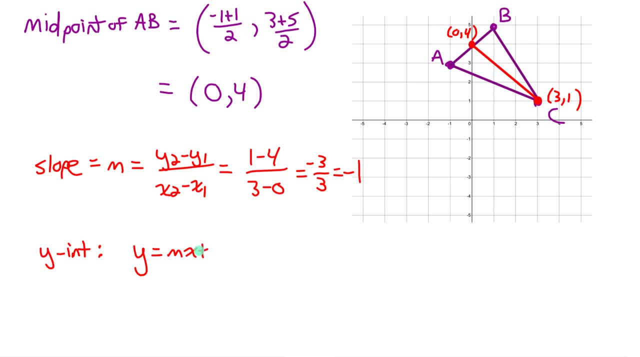 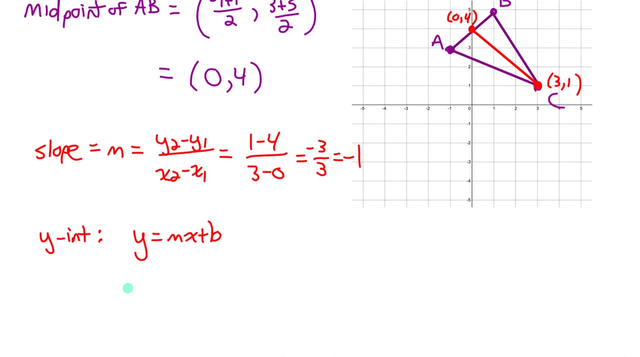 median. I'm going to have to into the equation: y equals MX plus B. I'm going to have to sub in the slope, I know, and a point on the line, doesn't matter which point, I can pick: the point zero, four, And actually that's already the y intercept. I know the y intercept is four, But let me just show. 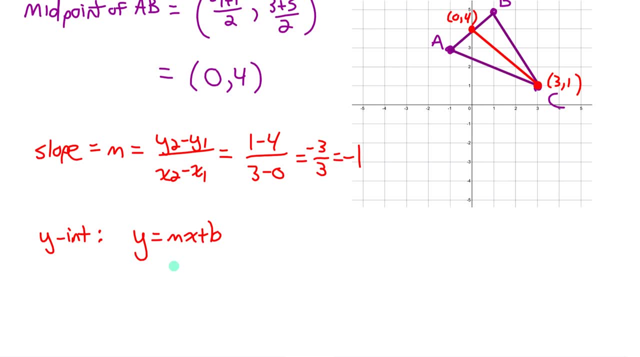 you algebraically how we would get it. So we would plug in the point zero four for x and y, the y coordinates, for the x coordinate is zero and we know M is negative one. And we solve for B. four equals zero plus B, So B is four. 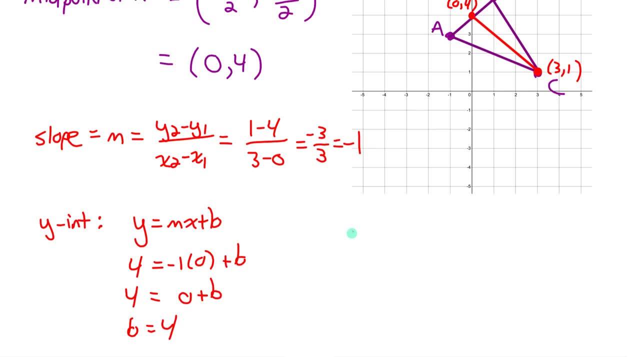 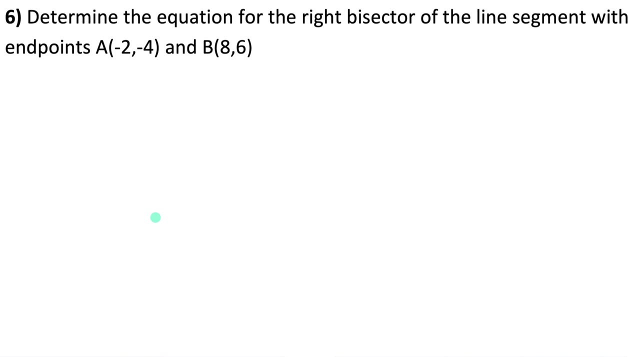 So now that I have the slope and the y intercept of the median, I could write the equation: y equals we sub in for M and B, so negative one x plus four, which you would just write as negative x plus four. So that's my final answer. That's the equation of that red line. Example six: determine: 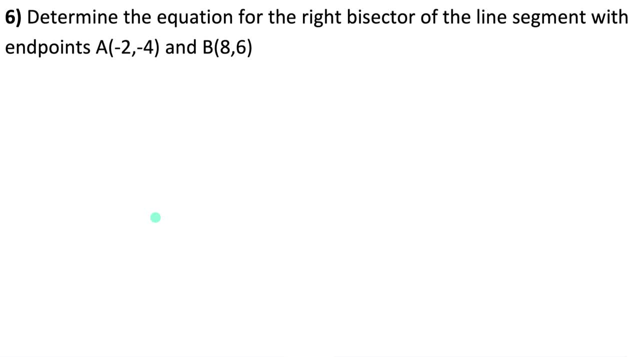 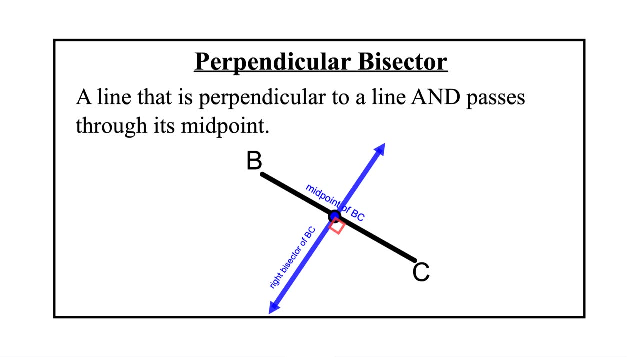 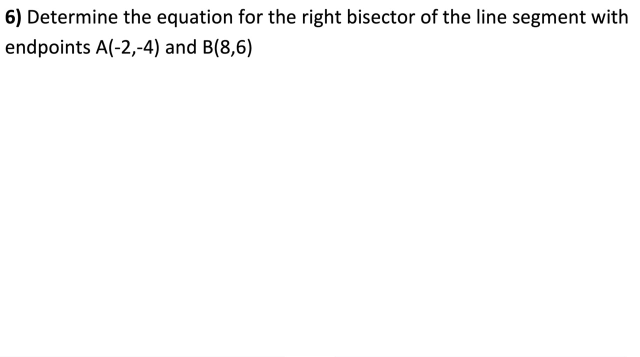 the equation for the right bisector of the line segment with the endpoints A and B. Let's remember what a right bisector is. The right bisector, often called the perpendicular bisector, is a line that is perpendicular to a line and passes through its midpoint. So I know my perpendicular bisector is going to be perpendicular. 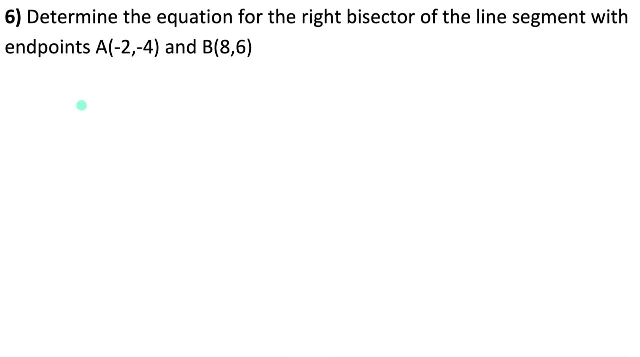 to the line connecting A and B. So I'm going to need to know the slope of A and B, which I know I get by doing change in y over change in x. So y two minus y, one, six minus negative four over x two. 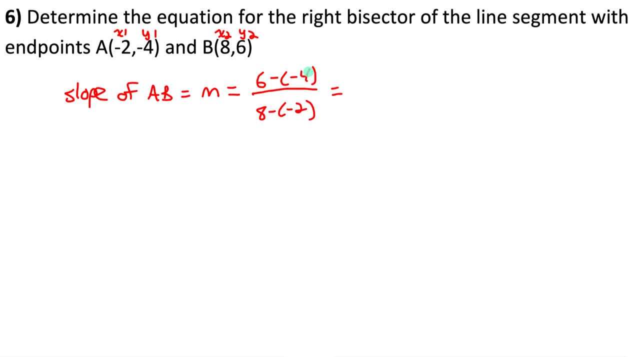 x one, eight minus negative two. So that gives me 10 over 10, which is one. And I know my right bisector is going to be perpendicular to this line, So it's going to have a slope perpendicular to one. perpendicular slopes are what are called negative reciprocals of each other, So I would have to take 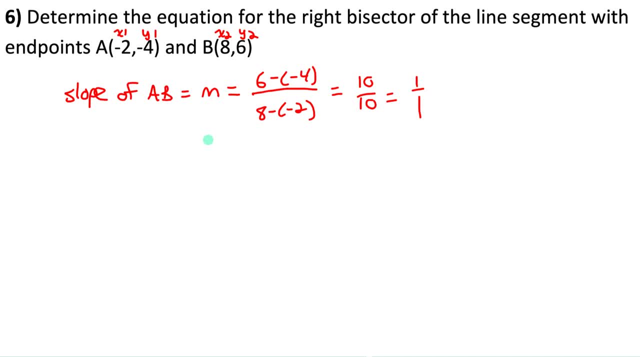 this one, which you could rewrite as one over one, flip it and change its sign. Well, the reciprocal of one over one. if we flip that, it's still one over one, but we do have to change its sign, So it becomes negative. 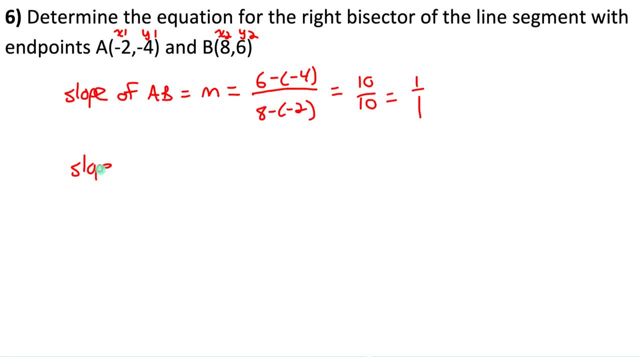 One over one, so negative one. So our slope of our right bisector- I'll call that the perpendicular slope- That equals the negative reciprocal of one over one which is negative, one over one which is just negative one. If I want the equation of the right bisector, not only do I need its. 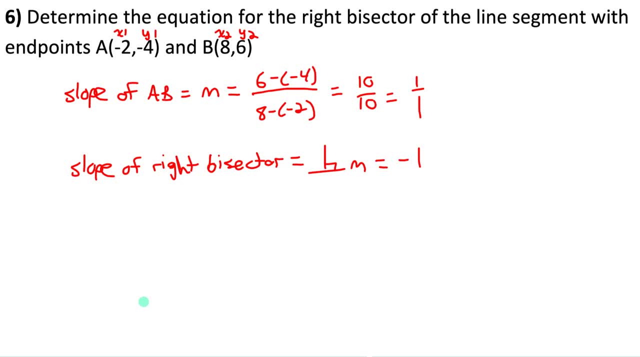 slope. but I need its y intercept And to find that I'm going to need to know a point on the right bisector. Well, I know the right bisector goes through the midpoint of A- B, So I'm going to need to know the midpoint of A- B. So I'll average the x coordinates negative two plus eight. 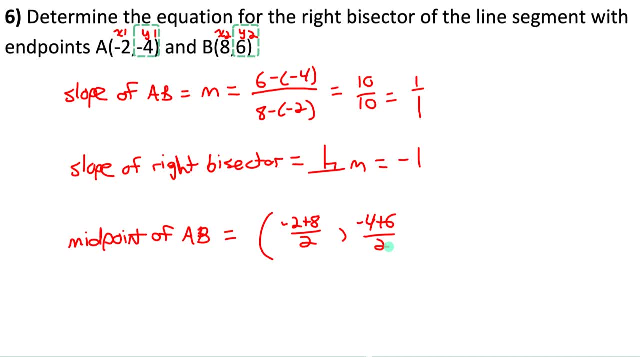 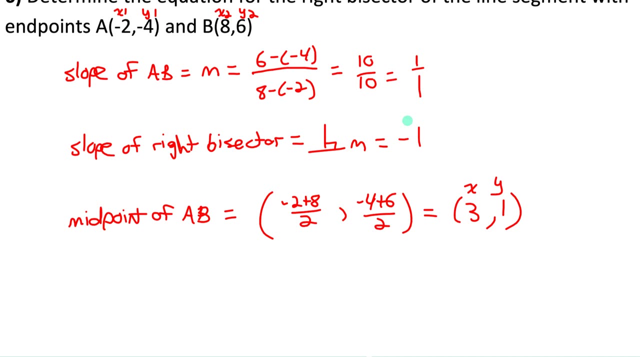 and average the y coordinates negative. four plus six over two. So my midpoint the x coordinate is six over two, which is three. The y coordinate would be two over two, which is one. So my midpoint is three, one which is an x and a y coordinate. I now take that x and y and the slope of my right. 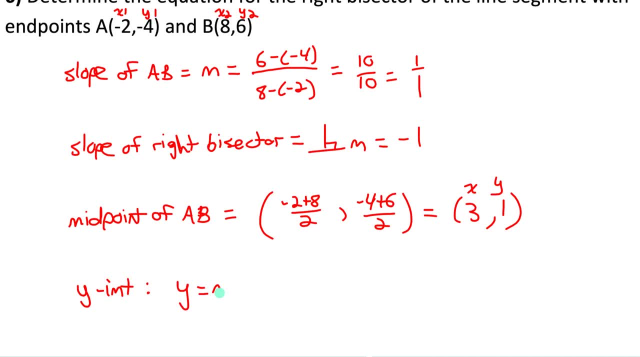 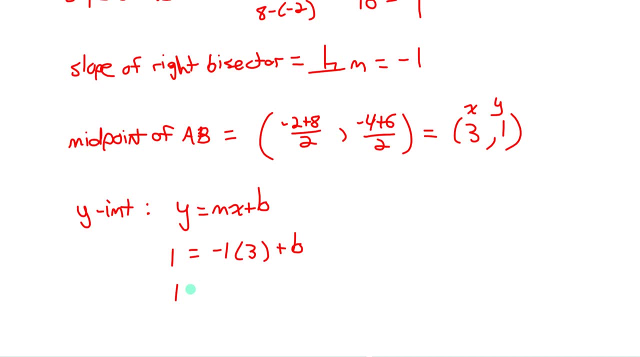 bisector and I can solve for B the y intercept. So I'll sub in my point for x and y and negative one for my slope, And if I solve this for B, I get B equals four. So I can now write my final equation by subbing in my m and my B values into: 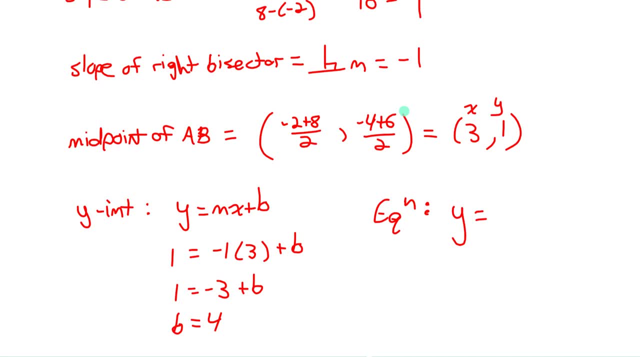 y equals mx plus B. So y equals- and make sure you use your perpendicular slope because we're doing the right bisector equation. So negative x plus the B value four. So there's my final answer. Example seven: classify the triangle with these vertices as either scalene isosceles or. 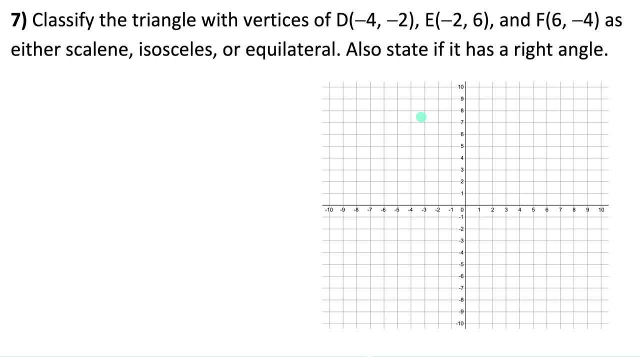 equilateral and also state if it has a right angle. Let me start by just drawing it quickly for you All. right, there we go. It looks like it's probably scalene Angle D looks like it might be close to 90 degrees. We'll have to do some calculations to know for sure. So if I want to 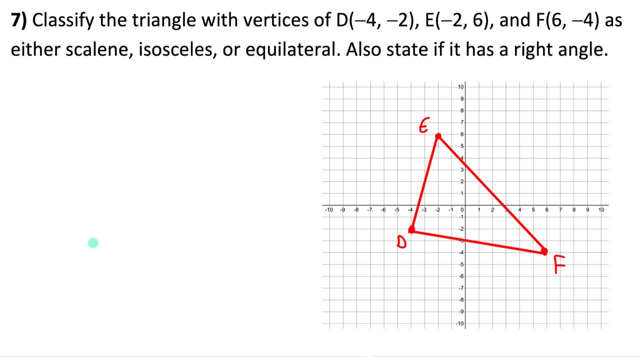 classify the triangle and give proof as to what shape it is, I'm going to need to know the length of each line which we can use our distance formula for. So let's find the distance of all three side lengths. So let me start with side DE. Now you can do DE or ED, doesn't matter, I'll do DE. 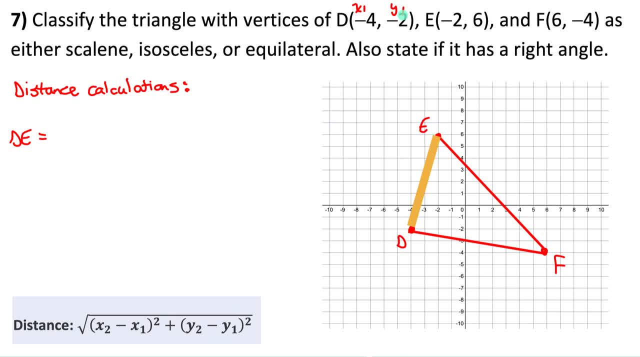 I'll make D- my first point, x1, y1, and E my second point, x2, y2.. Plug that into my distance formula and get the length of side DE, So I would have the square root of difference in the x's. 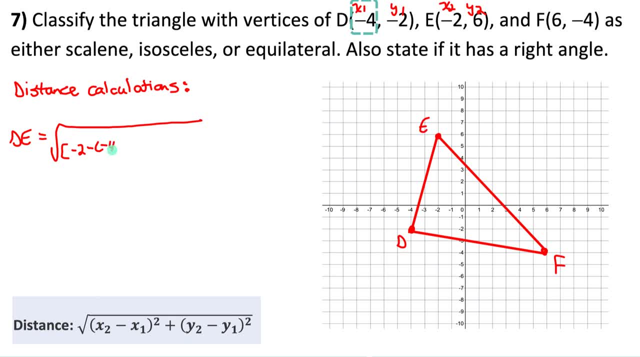 squared, so negative two minus negative four squared plus the difference in the y's squared six minus negative two squared. If I simplify, underneath the square root I'd have two squared eight squared, which is 64.. So four plus 64 is 68. So this would be root 68.. We would do the 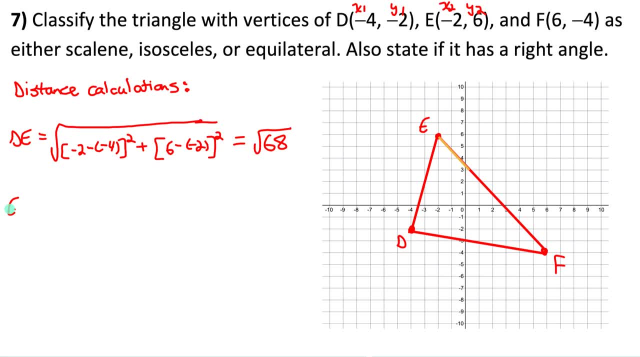 same thing for the other two sides, So for side EF and DF, and then we'll have all three side lengths. For time's sake of this video, I'm just going to fast forward through me solving for these side lengths. Okay, I have all three side lengths. Notice, all three sides are. 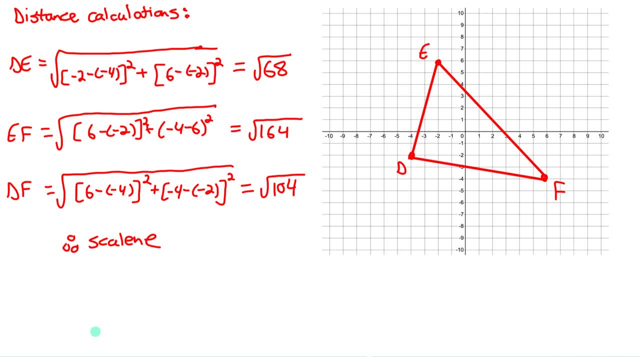 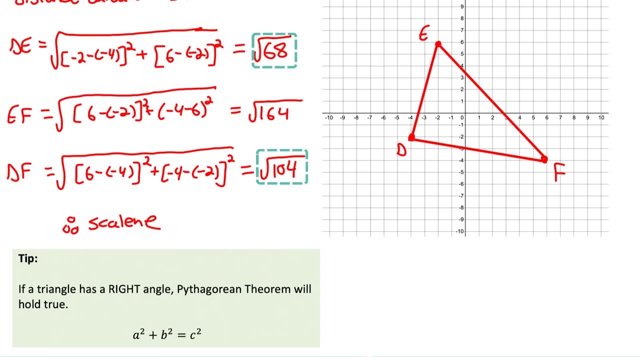 different lengths. Therefore, this is a scalene triangle. But does it have a right angle? Well, I know that right angle triangles, Pythagorean theorem is true: The sums of the squares of the shorter two sides is equal to the square of the longer side. So let's check: Is the square root? 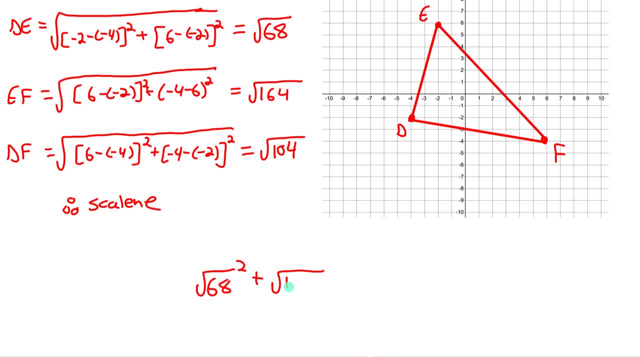 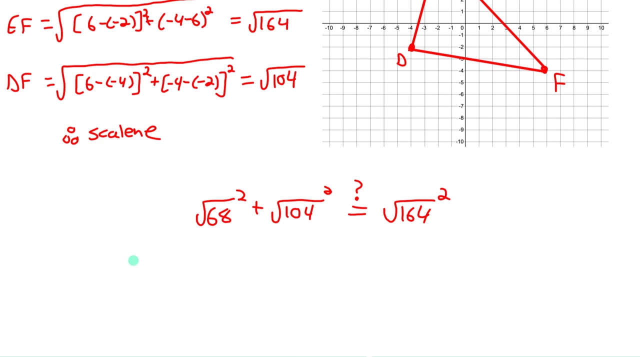 of 68 squared, plus the square root of 104 squared, is that equal to the square of the longest side. So root: 164 squared. If this is true, then there's a right angle. If it's not true, then there's no right angle. 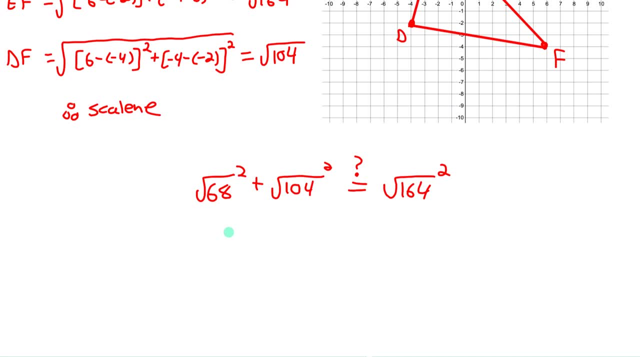 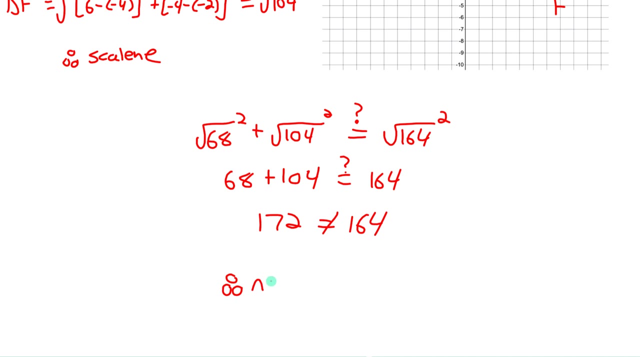 Square rooting and squaring are inverse operations. They cancel each other out. So really, what we have here is 68 plus 104.. Is that equal to 164? It's not. 172 does not equal 164.. Therefore, there's no right angle, Therefore not a right triangle. Example eight: This: 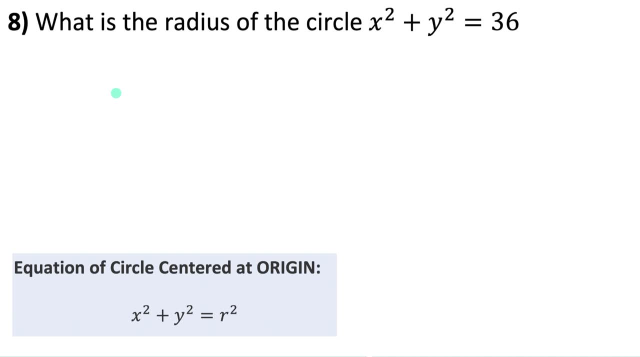 is a really quick one. What's the radius of a circle? Remember the equation of a circle is: squared plus y squared equals r squared. In this case, r squared is 36.. So the radius squared is equal to 36, which means the radius would be equal to the square root of that And the square 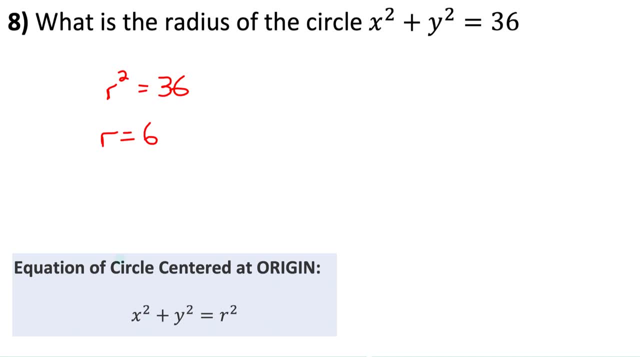 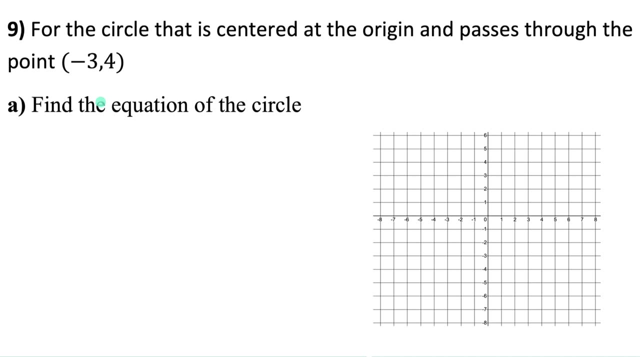 root of 36 is six. We don't have to consider the negative square root of it because radius lengths can't be negative. We only look at the positive. So the radius is six units Nine for the circle that's centered at the origin and passes through the point negative three, four. So center at the. 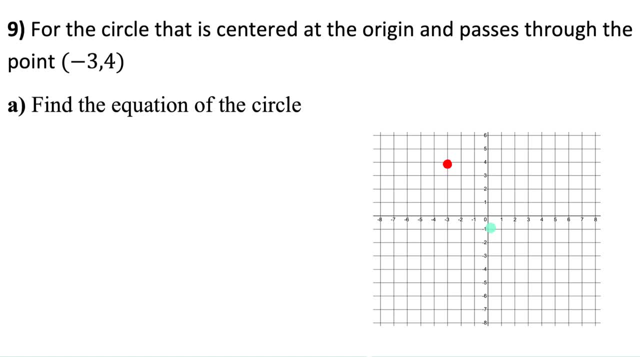 origin passes through this point. negative three, four. Let me just draw a circle that does that quickly for you. That circle, we want to find the equation of this circle. And part B asks us to check if this point five, two lies on the circle, inside of it or outside of it. And we'll do this. 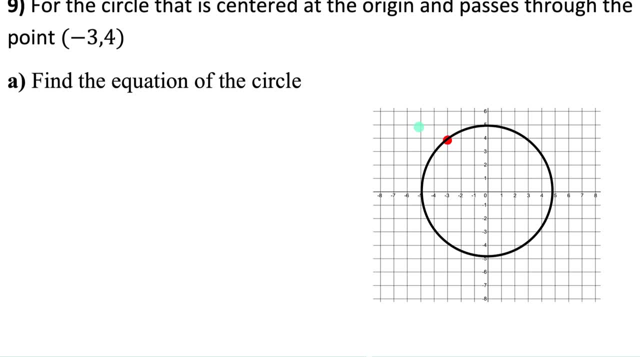 algebraically. So if I want the equation of this circle, well, I know one point on the circle, this point right here: negative three, four, that's an x- y point. the equation of a circle is of the form: x squared plus y squared equals r squared. So I need to know what's the radius. 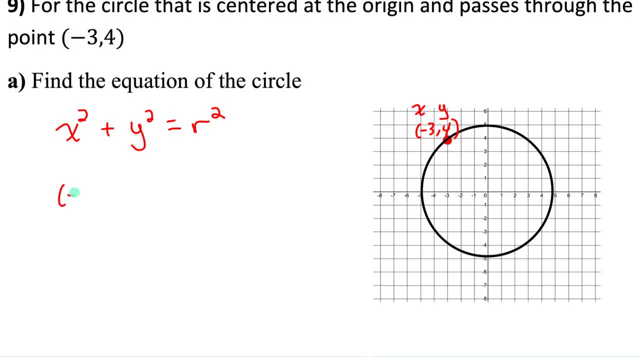 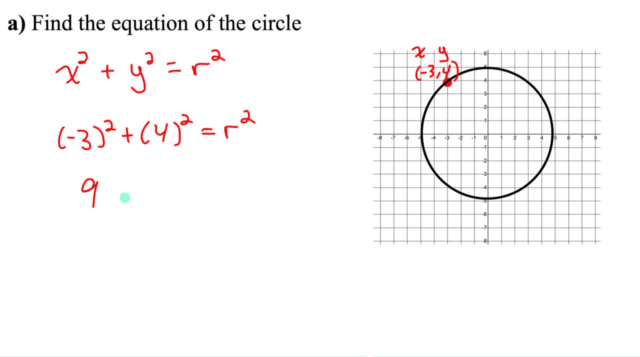 squared. to figure that out, Just plug in your x and y into the equation. So negative. three squared plus four squared is equal to the radius squared. I have, nine plus 16 equals r squared. So r squared is 25, which means the 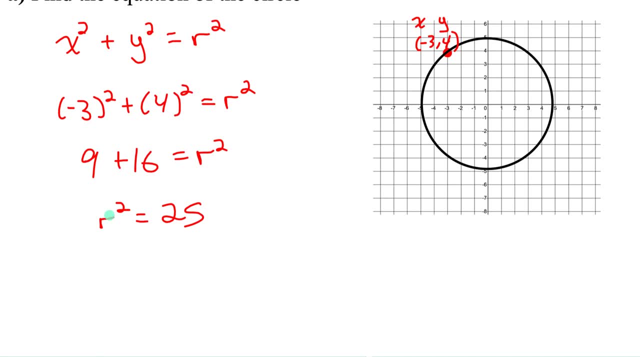 radius is five. but I don't need the radius in this question. I just need the radius squared so that I can write the equation. because the equation is: x squared plus y squared equals r squared, which is 25.. So my final equation would be: x squared plus y squared. 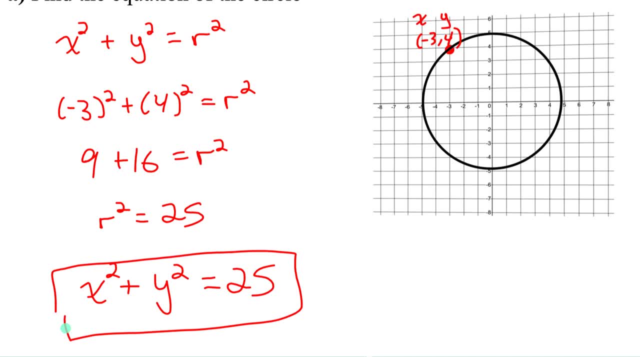 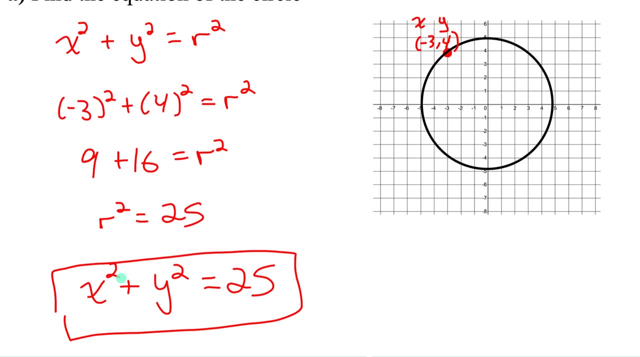 equals 25.. That's the equation of this circle. Now if we want to check if this point lies inside the circle, outside of it or on the circle, we just plug five, two into the equation of the circle and see if we get a number that's less than 25, equal to 25, or greater than 25.. That'll tell. 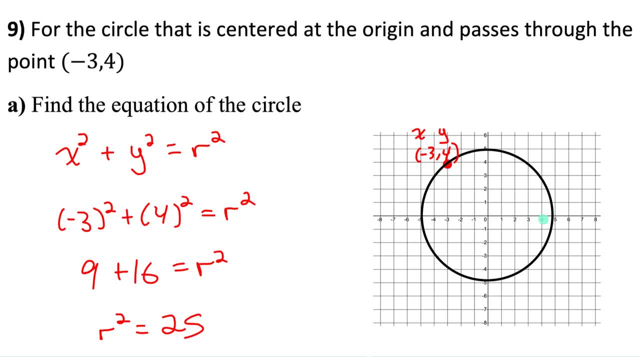 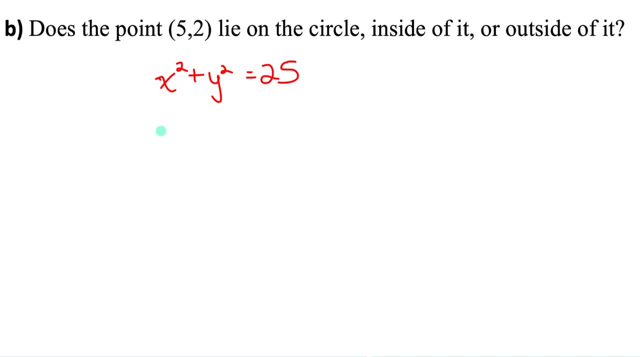 of our circle and we see what happens when we plug this value in. So if we plug five and two in for x and y, well, five squared plus two squared, that's actually going to give me a value that's bigger than 25, right, 25 plus four is 2929, is bigger than 25.. That tells me that the point. 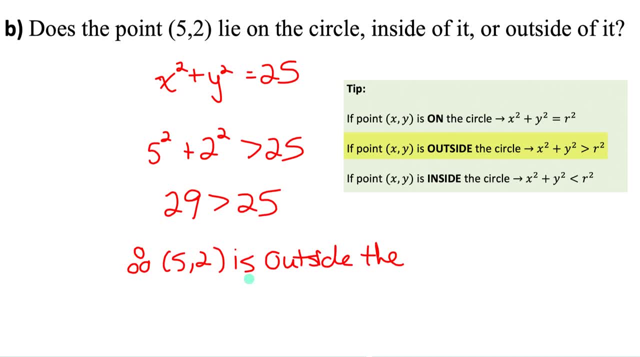 must be outside the circle If we got 25 equals 25 would be on the circle If we got something less than 25,. like we got 25, we would be outside the circle If we got something less than 25,. 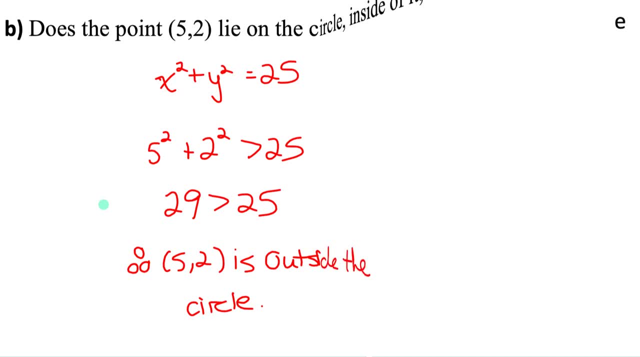 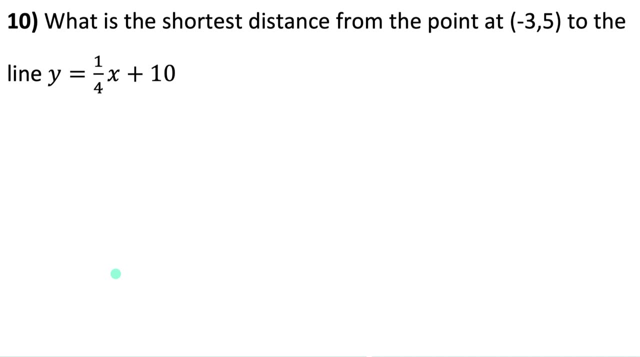 like we got 21 less than 25, I mean inside the circle. Example 10 says what's the shortest distance from point negative three five to this. line y equals a quarter x plus 10.. This question is going to involve pretty much everything from this unit. So we've got the line y equals a quarter. 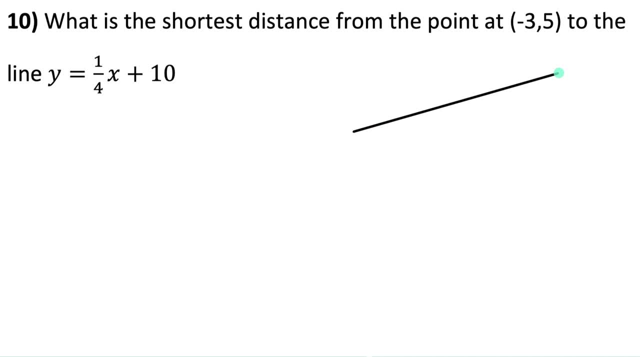 x plus 10.. I'll just draw an approximation of that line there for you there, just to visualize what's happening here. And we have the point negative three, five. I don't have a Cartesian grid, but let me just put it right here. Here's the point negative three. 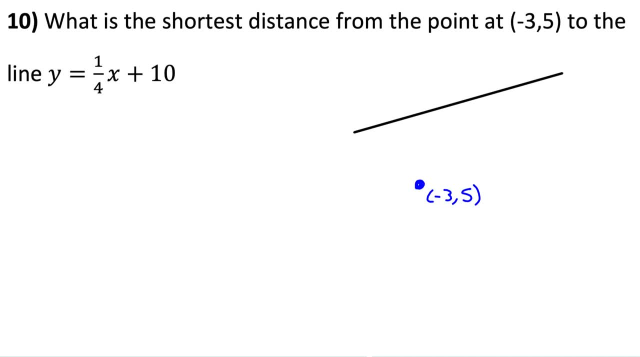 five, I'm looking for the shortest distance from that point to that line. the shortest distance from the point to this line isn't going to be something like that or like that. it's going to be along a line that's perpendicular to the original line. So it's going to be along that line. 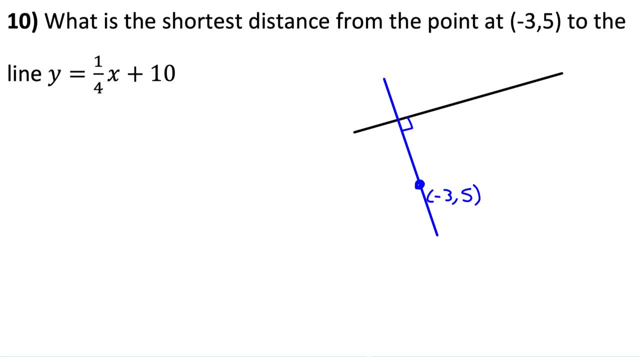 right there which forms a 90 degree angle with the original line: y equals a quarter x plus 10,. right, this black line is: y equals a quarter x plus 10.. And I want to figure out the shortest distance. So basically, the distance is going to be the shortest distance from that point to that. 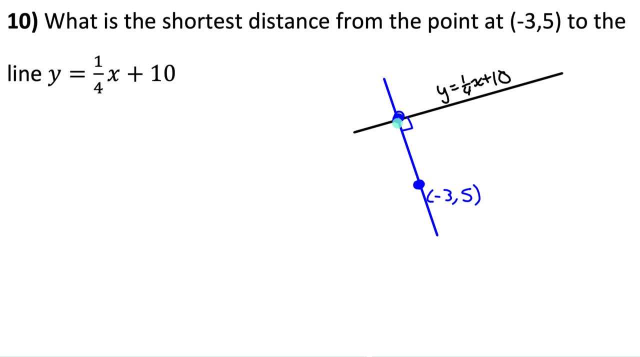 distance from this point to whatever this point is here. I don't have that point, but I'm definitely going to need it to find that point. Well, that's where the blue line intersects the black line. So if I have the equation of the blue line, I could figure out where they intersect. So to find the 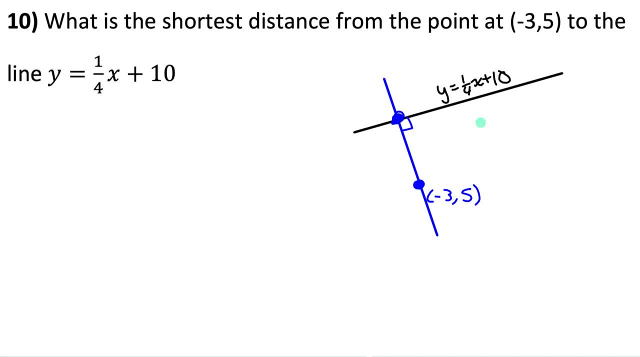 equation of the blue line- well I need it slope and y intercept. Well I know it's perpendicular to y equals a quarter x plus 10.. So I know its slope is going to be the negative reciprocal of a quarter. So the perpendicular slope would equal the negative reciprocal of a quarter which. 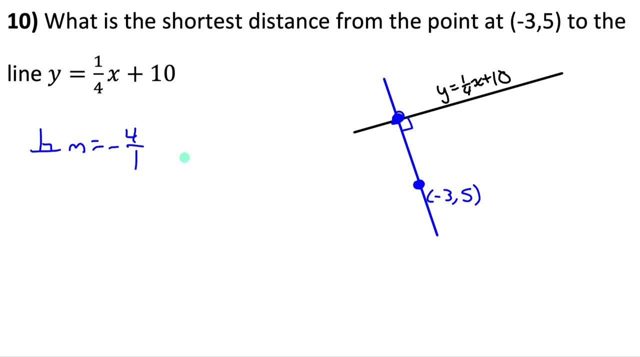 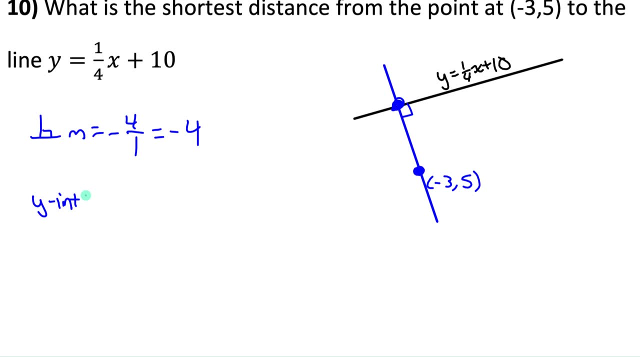 means flip it and change the sign, So it's negative four over one, which is just negative four. To write the equation of that blue line, I also need the y intercept, the b value. to get that into y equals m x plus b. I have to plug in a point on the line and the slope. Well, I know a. 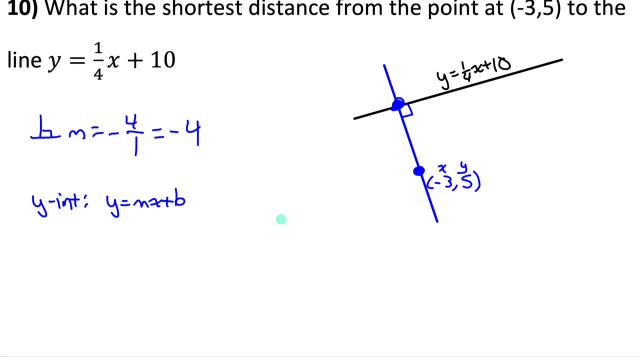 point: negative three, five. it has an x and a y. So sub that in five. for y, I know the slope of the blue line is negative four. I know x is negative three. if I solve this equation for B, negative four times negative three is 12, subtracted over five minus 12 is negative seven. So my b value is: 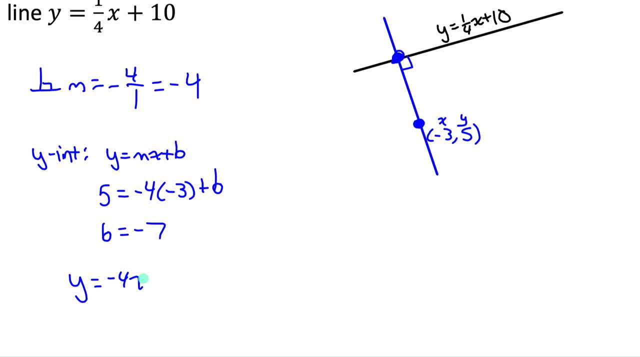 negative seven. So the equation of that blue line is: y equals negative four x minus seven. So this blue line, y equals negative four x minus seven. Now let's figure out where does that blue line intersect, the black line? I've got two equations I can solve using substitution or elimination. 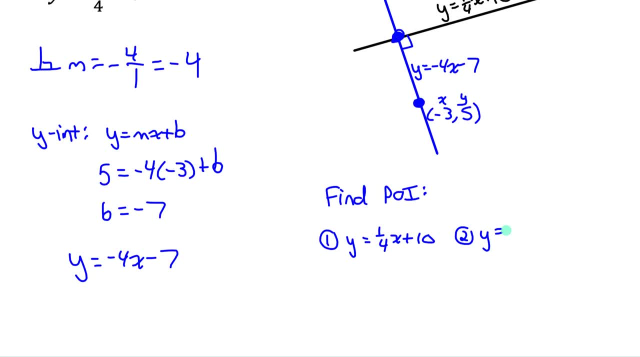 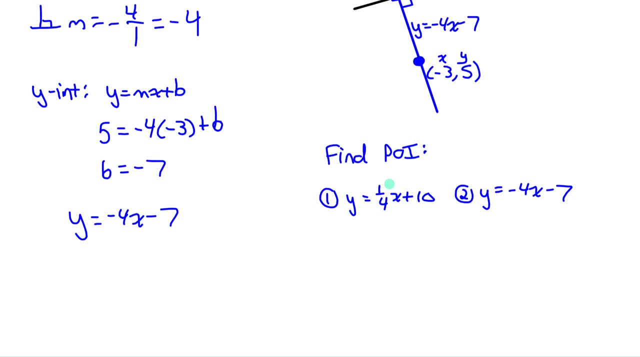 Let me rewrite the two equations, And I think, since y is already isolated in both equations, I think substitution is the easiest method. So really all we do is we take what y is equal to from one equation and replace the y and the other equation with that. So replace the y and second. 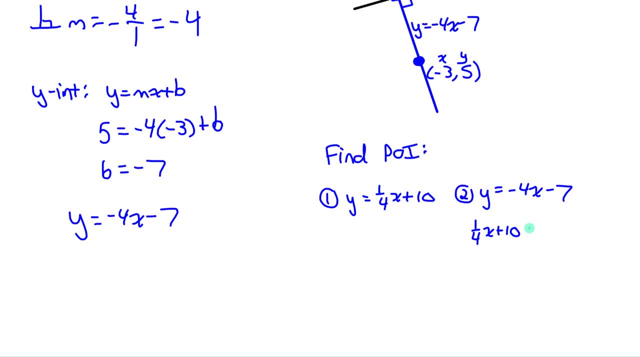 equation with a quarter x plus 10.. And now let me solve this equation. I don't really like this fraction here, So what I'm going to do is I'm going to get rid of the fraction by multiplying both sides of the equation by its denominator. So I'll multiply both sides by four. Now give me x. 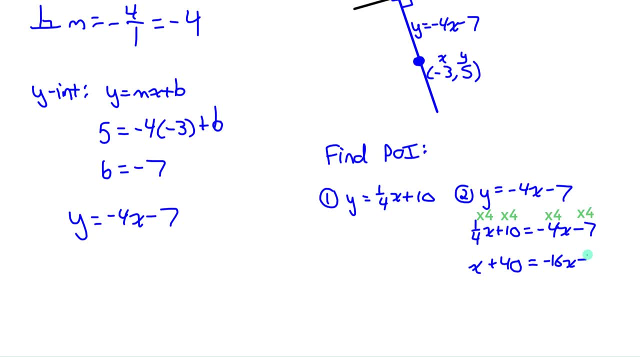 plus 40 equals negative 16 x minus 20.. Now I'll collect my like terms onto the same sides of the equation. I've got 17 x equals negative 68. So I've got x equals negative four. I now need to figure out what y equals. So let me just sub x equals negative four into either. 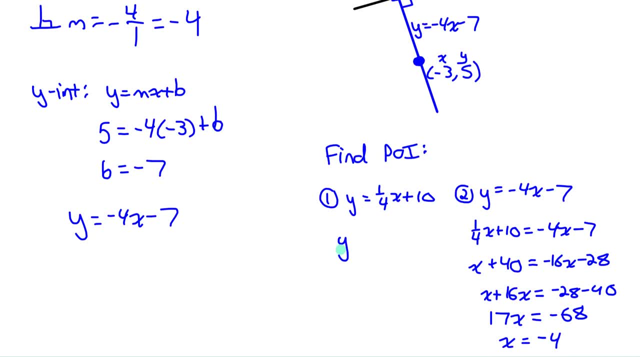 original. I'll just plug it into the first one because I have room underneath of there, So I'll plug negative four in for x A quarter times negative four is negative one, So I've got negative one plus 10, which is nine. 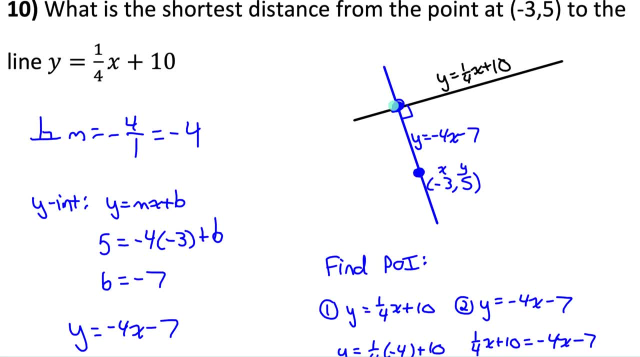 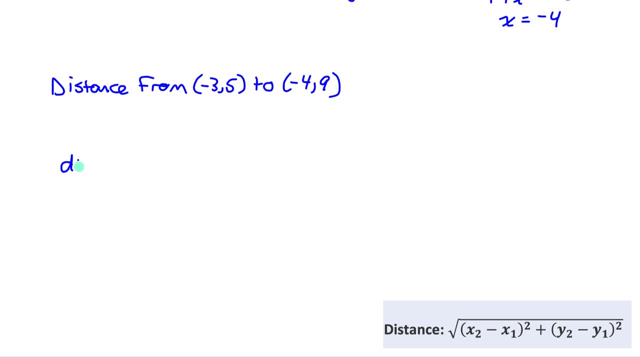 So my point of intersection is the point negative four nine. So I know this point right. here is the point negative four nine. The shortest distance is going to be the distance between negative three five and negative four nine. So if I use the distance formula, I'll have my final answer. 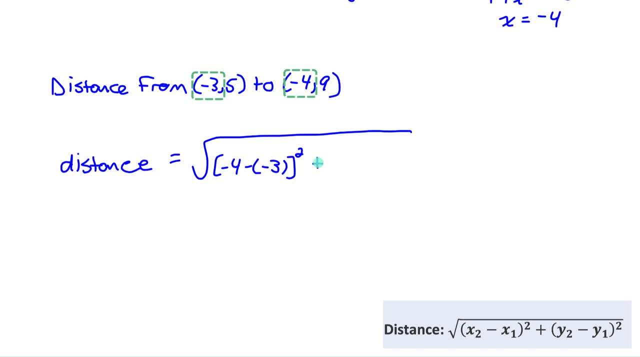 So I'll do the difference in the x coordinates squared plus the difference in the y coordinates squared, So this gives me one Plus 16.. So I have root 17 units. So that's the shortest distance from the point to the line. 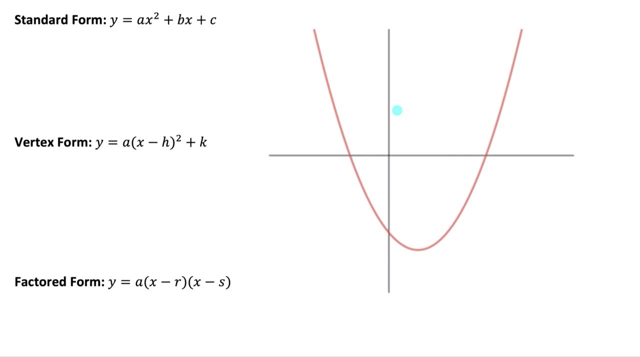 In this unit you look at the three versions of equations. a quadratic function can be given to you in standard, vertex and factored form. you learn the usefulness of all three versions and how to transition between the three versions. Now, quadratics are. 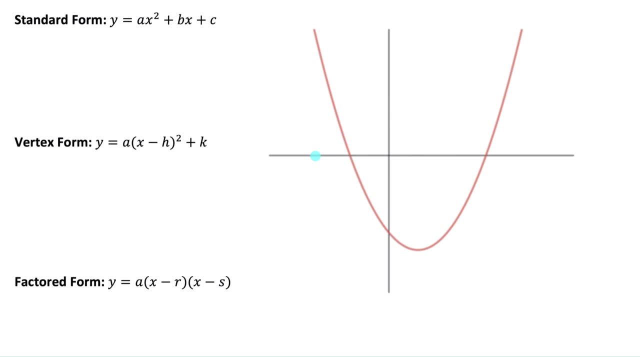 equations where the highest degree exponent on x is a, two, And the shape of those equations is always this u type shape which we call parabola. Now a standard form equation is most useful for determining the y intercept. So the y intercept we can tell from the equation because it's the c value. So this point right here. 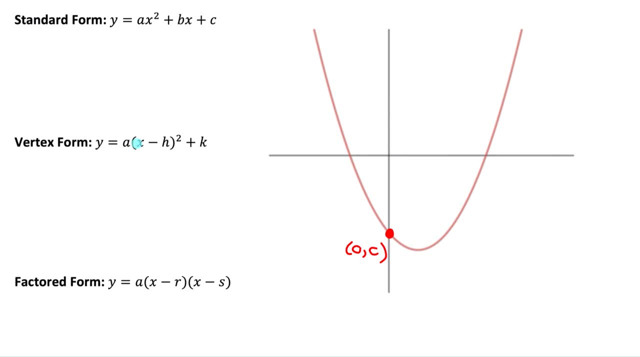 would be the point zero, And then whatever the C value is in the standard form equation. Another useful thing about standard form is that the a value tells you the direction of opening. If a is positive, the parabola opens up, like the one we have here. If a is negative, 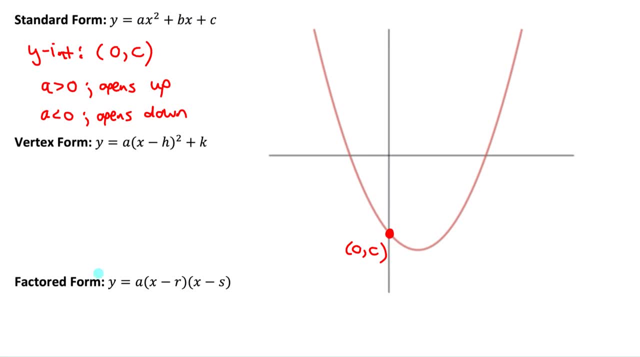 it opens down. Now a quadratic function could also be written in vertex form or factored form, and those have different uses. Now the a value in all three versions of the equation all tell you the same thing. they all tell you direction of opening. So let's just talk about what the 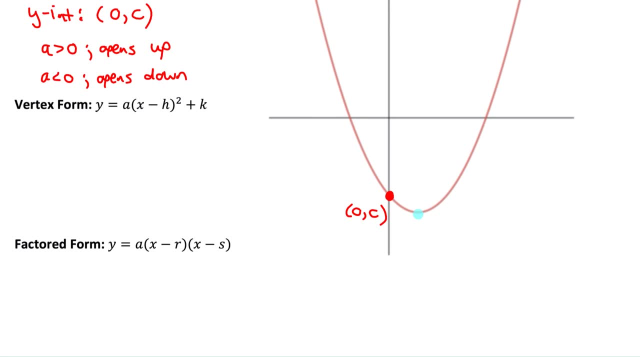 other variables tell you So in vertex form. well, it's obviously most useful for telling you what the coordinates of the vertex are. So, if it's in vertex form, y equals a times x minus h, squared plus k, the vertex is at hk. And notice, since the general format is x minus h, this h value is 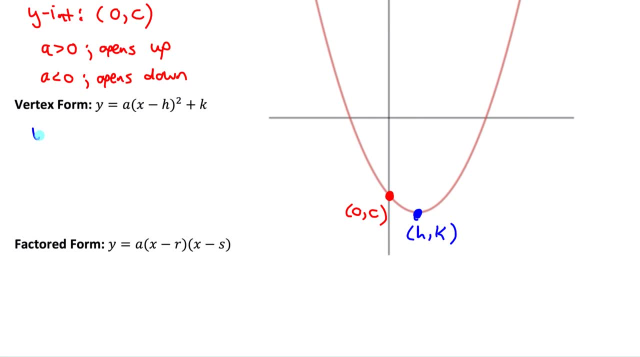 always going to be the opposite sign of what you see in the equation. So our vertex is at hk. that's what vertex form is useful for, And factored form is useful for the x-intercepts. So these points right here you could figure those out by if we have it in factored form. 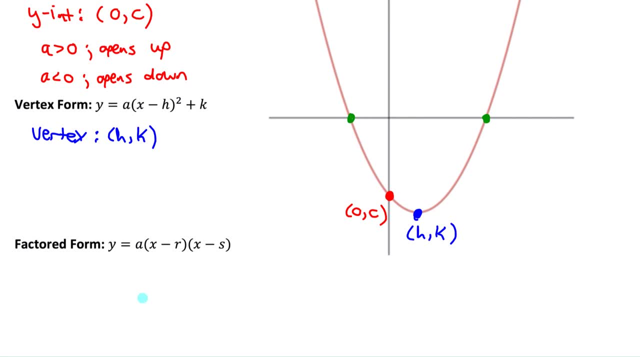 the form y equals a times x minus or times x minus s. we could find the x-intercepts by looking at the r and s values. This x-intercept, I could say, is at r0, and this one is at s0.. So the x-intercepts are at r and s. Let's look at how we can work with the three versions. 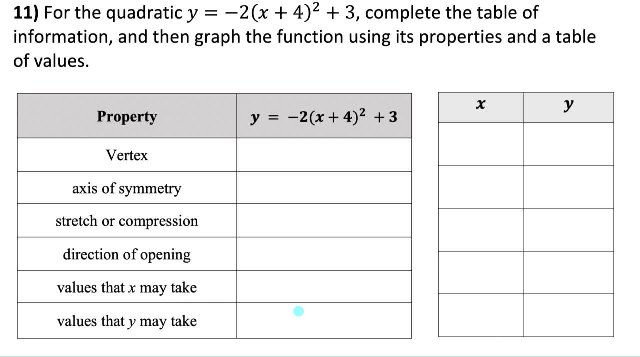 of a quadratic and how to transition between the three. Question 11,. this quadratic is in vertex form. Complete the table of information. So the vertex is going to be at negative, 4,, 3, right, because the general format is x minus hk. 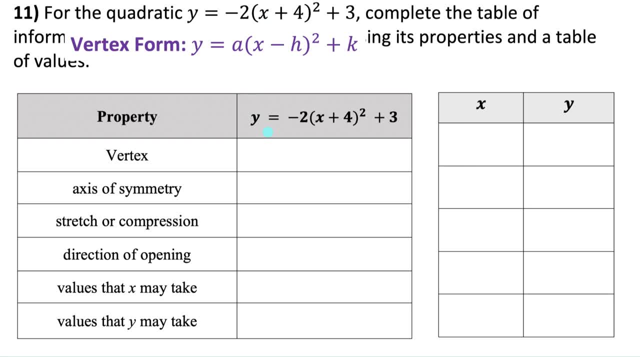 So it must be x minus negative 4 in order for it to look like x plus 4, which means h is actually negative 4.. So my vertex is at negative 4, 3.. x-coordinate is always opposite sign of what you. 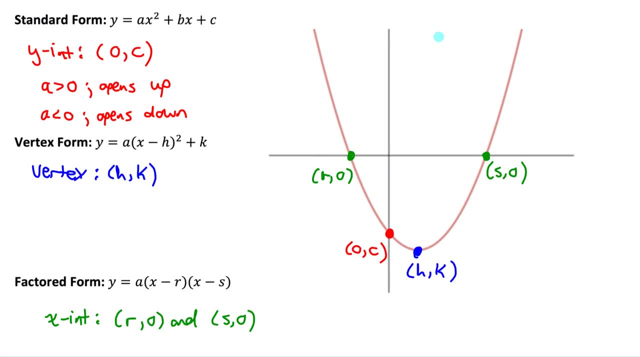 see there, The axis of symmetry is the vertical line that would divide the parabola in half. And that vertical line, notice, it passes right through the vertex. So the equation of the axis of symmetry is: x equals whatever the x-coordinate of the vertex is. So x equals h. So in this case, 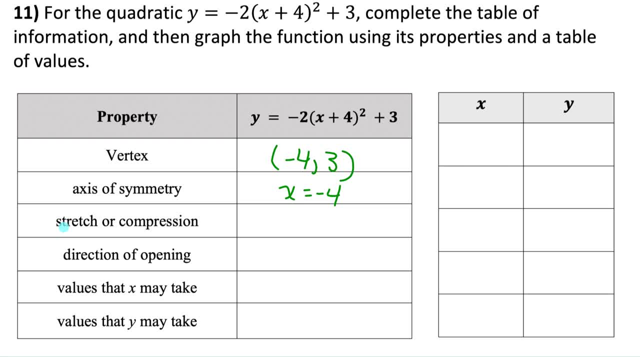 x equals negative 4.. Stretch or compression: we get that by looking at the absolute value of a. So the absolute value of negative 2 is 2.. So if the absolute value of a is bigger than 1, it causes a vertical stretch. So vertical stretch we say by a factor of the absolute value of a. So the 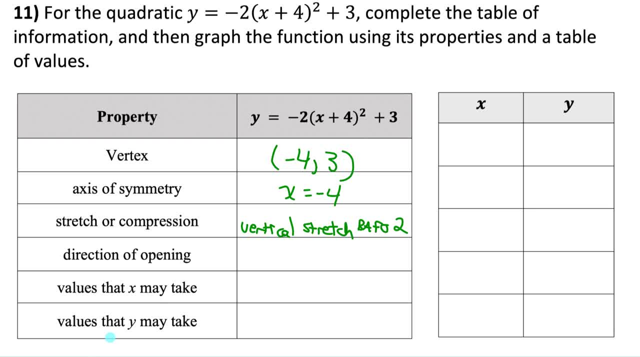 absolute value of negative 2 is 2.. Always use the absolute value when describing the stretch factor. The direction of opening is affected by the sign. Since the a value is actually negative, that tells us the quadratic is going to open down Values that x may take, also called the domain of the 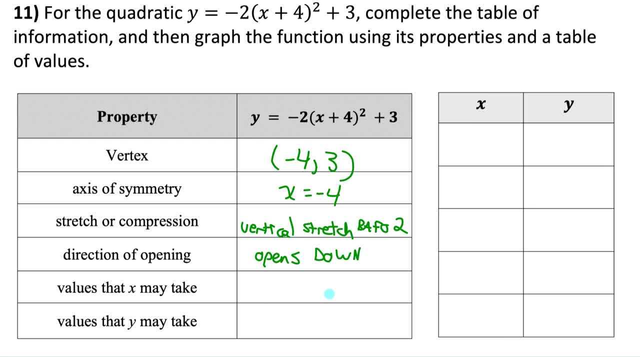 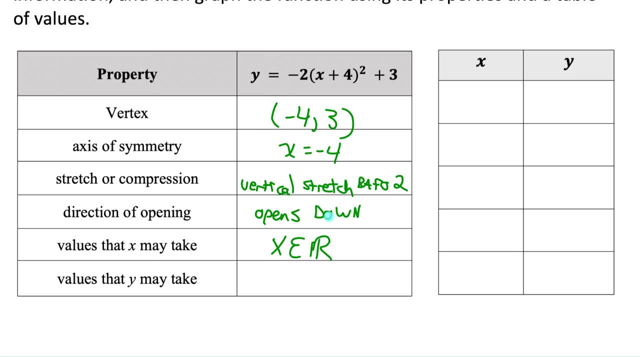 function. the answer for quadratics is always the same. There's no restrictions on the domain. We just say x can be any real number Values that y may take. well, since the parabola opens down, we know that the vertex is going to be at the very top of the parabola, right. The parabola is going. 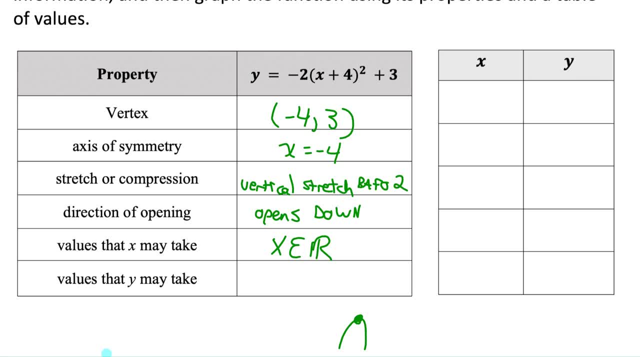 to look like this: The vertex is at the top, So we know the y values are always going to be at or below the y coordinate of the vertex. So the y values are always going to be less than or equal to the y coordinate of the vertex, which is 3.. If I'm going to graph this function, I'm going to 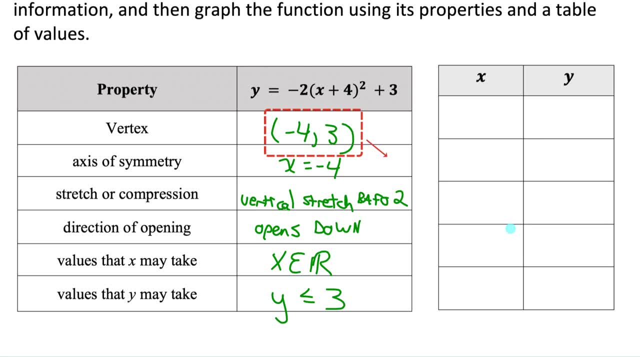 want to make a table of values, And in the table of values you always want to put the vertex in the center. So I'm going to put negative 4, 3 in the center. And now I want to pick points on either. 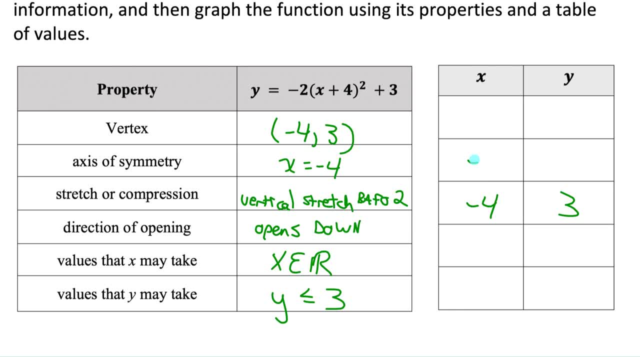 side of the vertex. So to the left of negative 4, I'm going to choose x values, negative 5 and negative 6.. And then to the right of negative 4,, I'll choose x values, negative 3 and negative 2.. 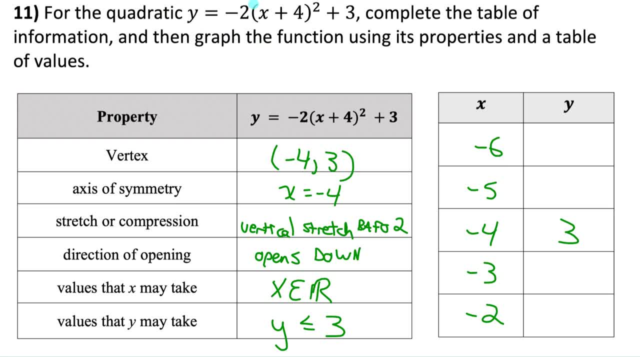 And now I just have to plug those in To my equation for x and calculate the y's. So if I plug negative 6 in for x, I would have y equals negative 2 times negative 6 plus 4 squared plus 3.. If I evaluate this, negative, 2 squared is: 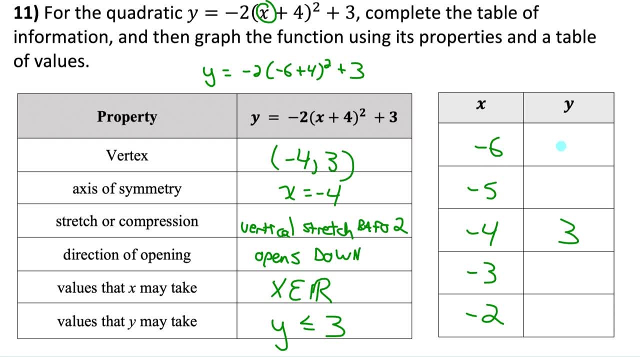 4 times negative. 2 is negative. 8 plus 3 is negative 5.. So this would be negative 5.. And since I know parabolas are symmetrical, if 2 to the left of the vertex, the y coordinate, is negative 5,. 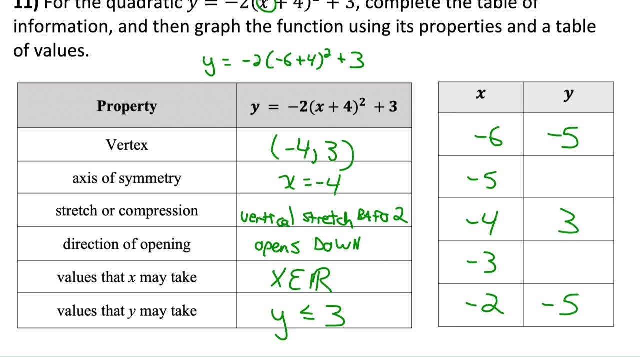 2 to the right, it's going to be at the same spot. Let me plug negative 5 in for x and see what I would get. Negative 5 plus 4 is negative. 1 squared is 1 times negative. 2 is negative. 2 plus 3 is 1.. So I know those are both 1.. So using those points, 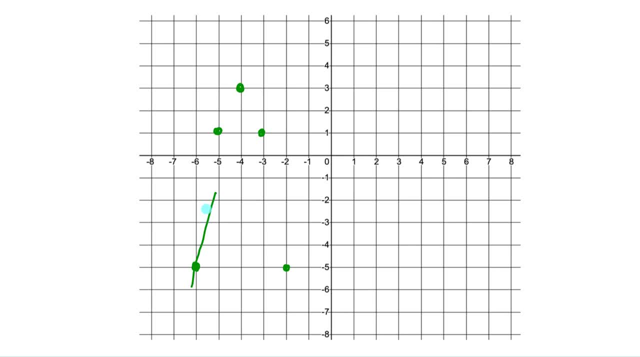 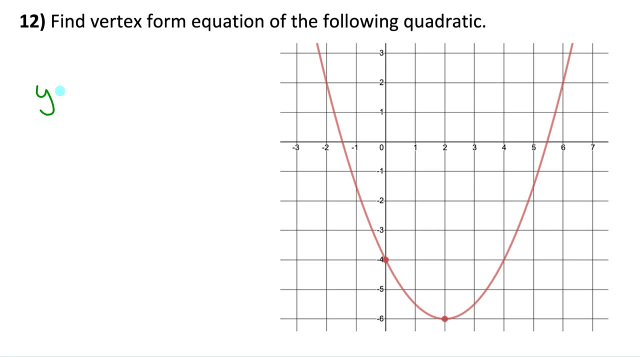 I could graph the quadratic And there's a rough sketch of the parabola. Let's go the other way. Here's the graph. Let's find the vertex form equation. So remember, vertex form looks like this: a times x minus h squared, don't forget the squared plus k. 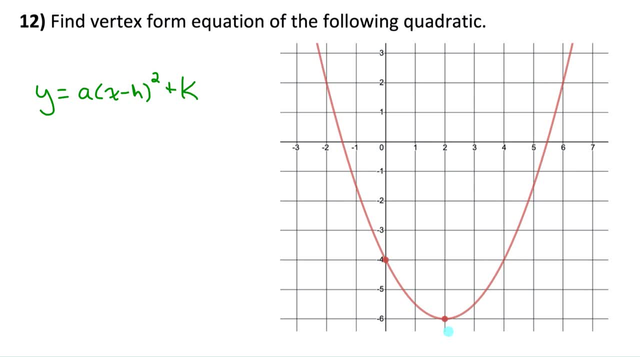 So I'm just going to write the equation. well, I just need to know the vertex. plug that in for h and k. but I also need to know a, the stretch or compression factor, And we'll solve for that by plugging in the vertex and a point xy. So I've got the vertex here. it's at 2 negative 6.. 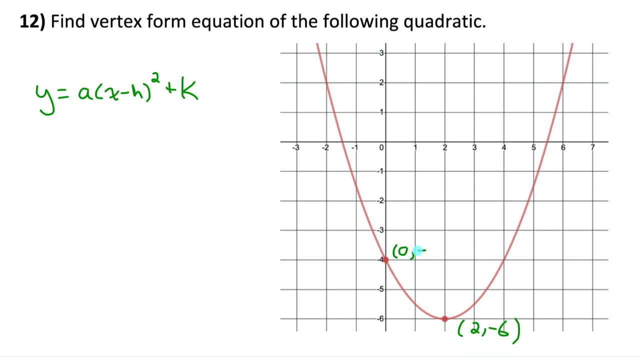 And it gives me another point here. it labels the y intercept that's at 0 negative 4.. I've got my xy, my hk, sub all that in and solve for a. I've got y value of negative 4,. 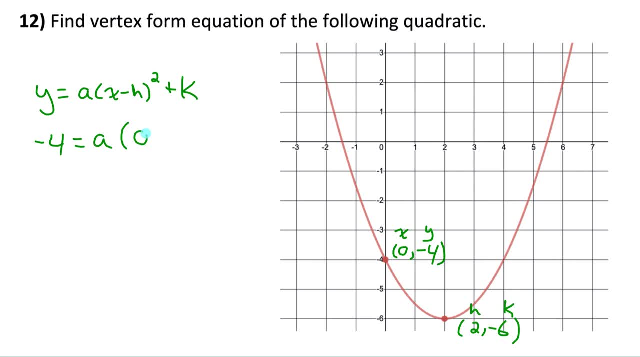 I don't know a. that's what we're solving for. x is 0, h is 2 squared plus my k value of negative 6. so plus negative 6, i'll just write minus 6. let's solve this for a. so in the brackets i'll do first: 0 minus 2 is negative 2 square. that i get. 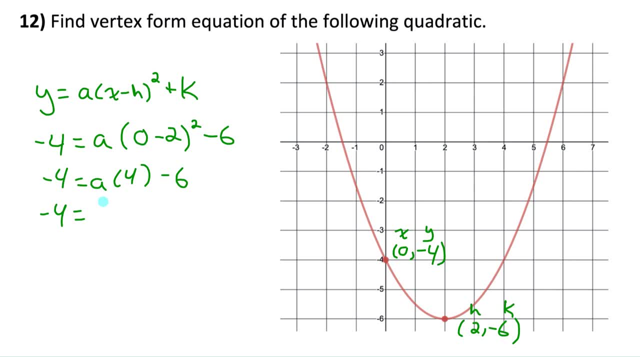 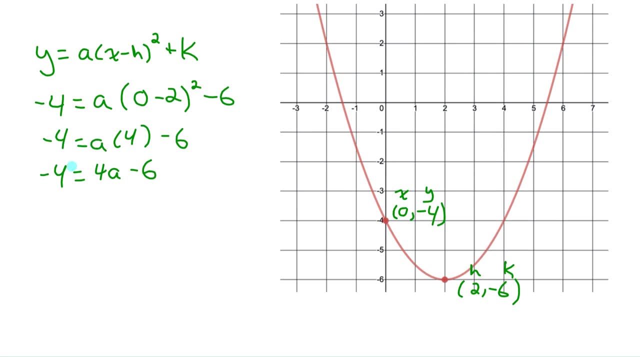 4. now it often helps, instead of writing a times 4, usually people write that as 4a. if we write it like that, you'll avoid mistakes. let me now add the 6 over negative. 4 plus 6 is 2, so i have 2. 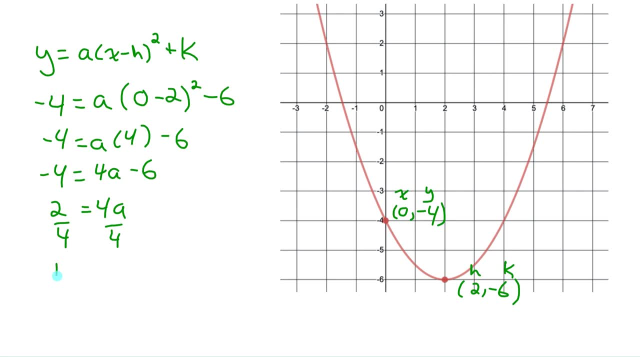 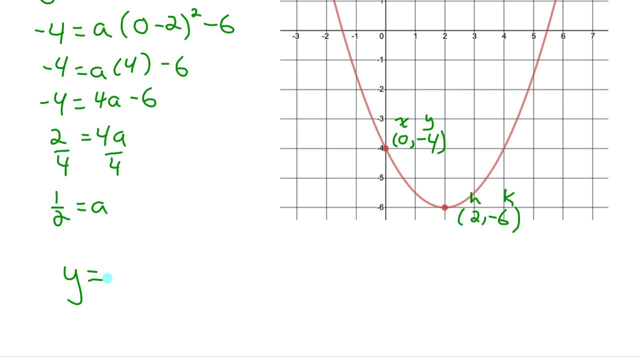 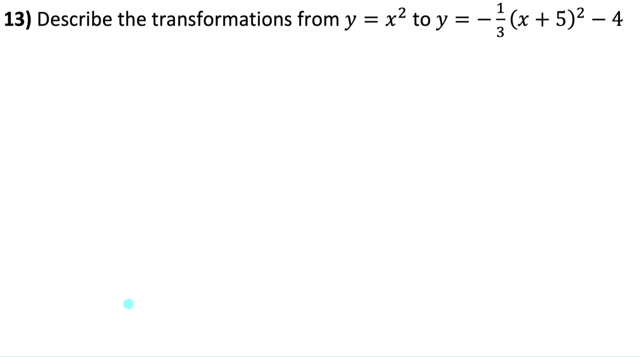 equals 4a. divide both sides by 4, i get a half equals my a value. so my final answer would have a h and k plugged into the vertex form. so a half x minus 2 squared minus 6, there's the vertex form. equation 13 just asked me to describe transformations in words, so we can describe the left and right. 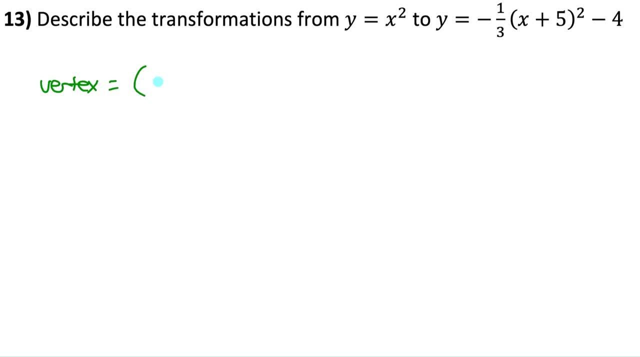 shift based on where the vertex is. so my vertex is at negative, 5, negative, 4. i get that from the h and k. remember h is always the opposite sign of what we see there. the vertex of x squared is at 0, 0, but now the vertex of this function is at negative, 5, negative. 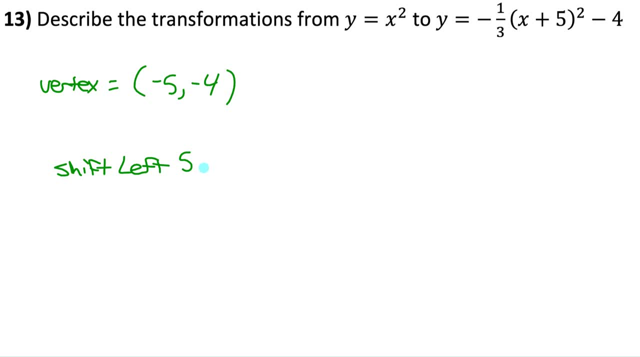 4. so for that to happen it must have shifted left 5 units and shifted down 4 units. now if i look at the absolute value of a, that will tell me the vertical stretch or compression factor. the absolute value of a is a third. if the absolute value is between 0 and 1, that's going to vertically. 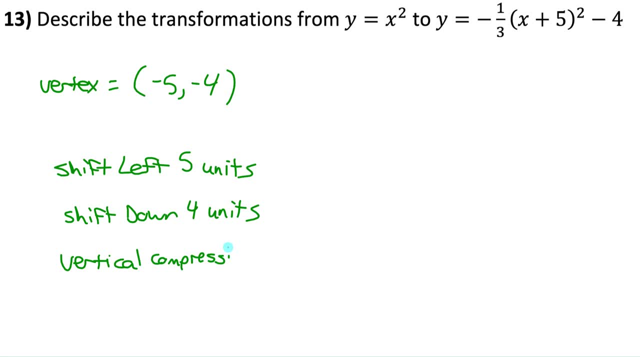 compress it. so i'm going to compress it vertically and i'm going to compress it vertically and i'm going to compress it vertically. so i would say vertical compression by a factor of the absolute value of a. so by a factor of a third. but the fact that it's negative means it's also going to be. 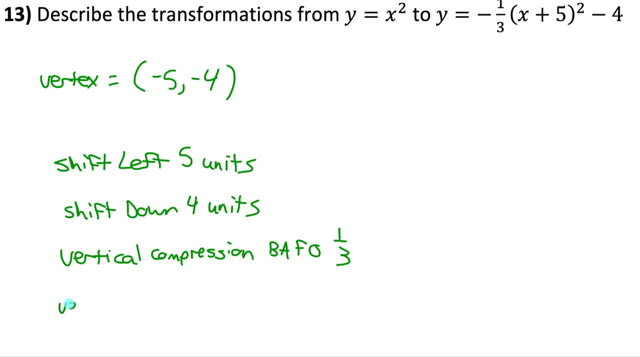 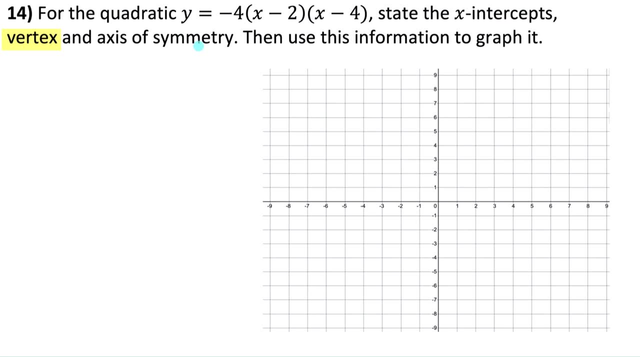 opening down, which means it's been vertically reflected. so we would say vertical reflection. example 14 for this quadratic, that's in factored form, we want to state the x intercepts, the vertex and the axis of symmetry and use the information to graph it well to find the x intercepts, if it's. 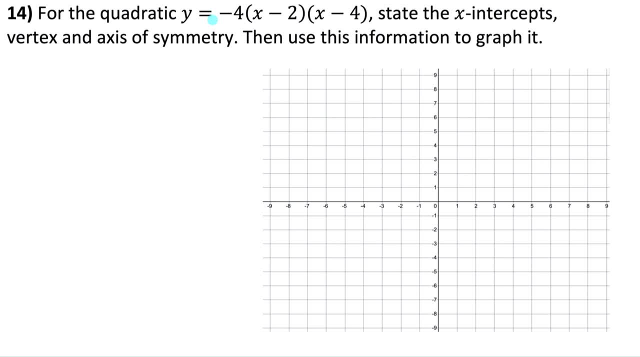 in factored form. that's easy. we're just looking to see what value of x would make any of the factors be zero. what would make x minus 2 be 0 would be if x was 2. so 2 is an x intercept. so we have an x intercept at 2: 0, and what value of x would make this factor be 0? well, 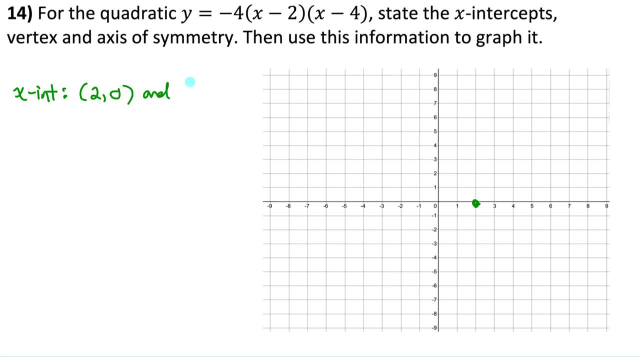 4 would make it be 0.. so there's another x intercept at 4: 0.. right, if we can make one of the factors be 0, we make the whole product be 0, which makes the y coordinate become 0.. so 2 and 4 are both x values that have a y value of 0, meaning they're x intercepts, and that's easy. 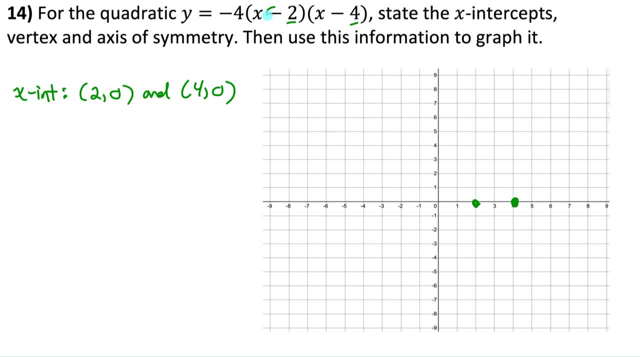 out from factored form. right, it's just these numbers here, remember, opposite sign of what you see there. now, where's the vertex? well, i know parabolas are symmetrical, so the vertex is going to be halfway between those. so a shortcut to find the x coordinate of the vertex would be to just 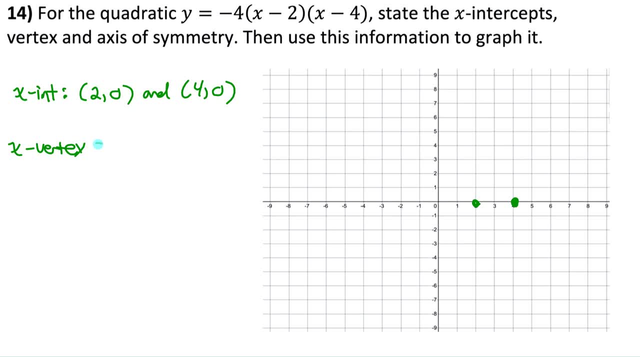 find the average of the x intercepts. so the x coordinate of the vertex would be equal to the average of 2 and 4.. and you average numbers by adding them, dividing by 2.. so the x coordinate of the vertex is 3.. but where's the y coordinate? to find the y coordinate of the vertex we have to 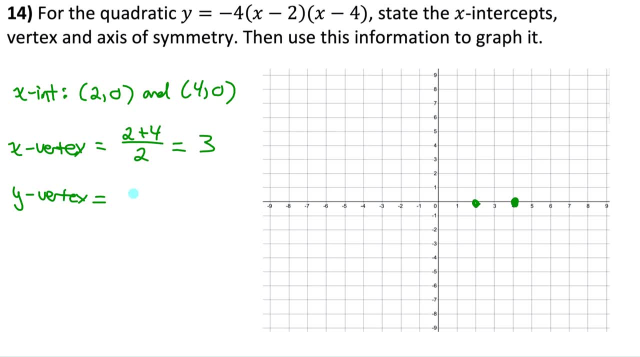 find the x coordinate and plug it into the original equation. so i would have negative 4 times 3 minus 2 times 3 minus 4, which is negative, 4 times 1 times negative 1, which is 4.. so my vertex is at the point 3, 4.. and the axis of symmetry is the vertical line that goes through. 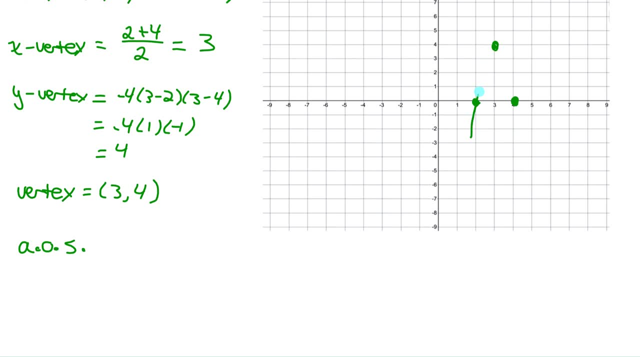 the middle of the parabola. so the parabola looks. let's do a rough sketch now. the parabola looks like this and we know that the axis of symmetry is the vertical line and it's going to go right through the vertex. the equation of that line would be: x equals the x coordinate of the vertex, so x. 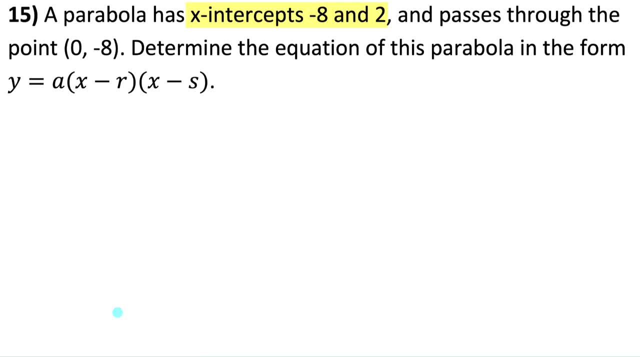 equals. 3 is the equation of the axis of symmetry 15. a problem has x intercepts of negative 8 and 2 and passes through the point 0. negative 8 determine the equation of this problem in the form here, this factored form. okay, well, the x intercepts are our r and our s, and we know a point x, y to. 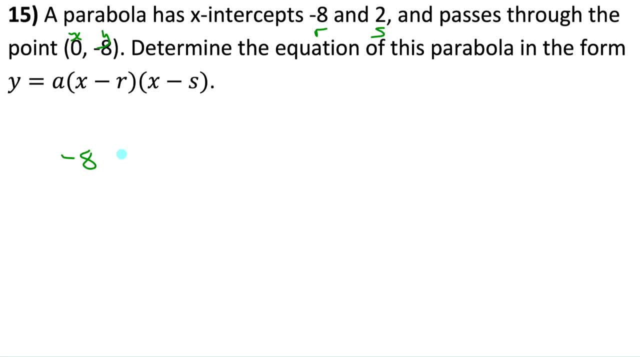 solve for a. so let's sub in what we know: y is negative 8. i don't know a, but my x value is 0, so i do 0 minus r. so minus negative 8 times 0 minus s, and s is 2.. now let's solve this for a negative. 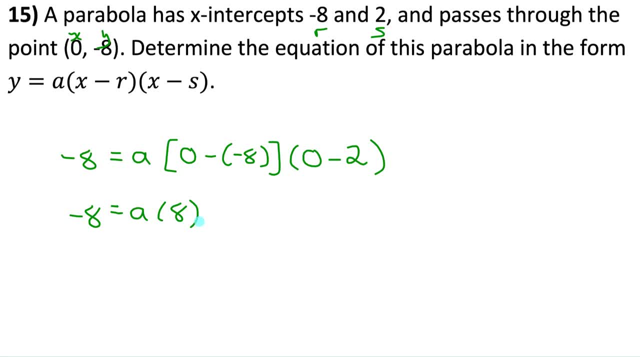 8 equals a: 0 minus negative 8 is 8, and 0 minus 2 is negative 2.. so negative 8 equals a times 8 times negative 2.. i'll write that as negative 16. a divide both sides of the equation and you. 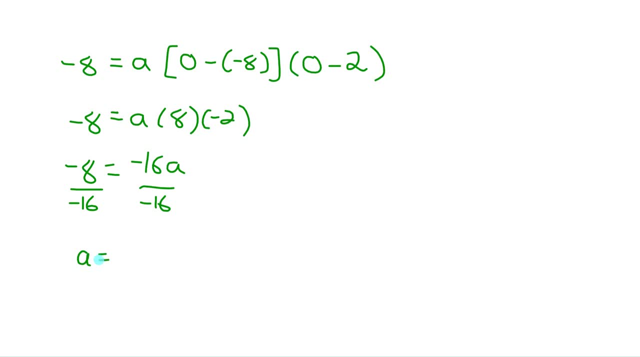 find negative 16 to isolate a, and i get a equals a half. so i could write my final equation: y equals a half and then sub in for r and s, but leave x and y, so x minus negative 8, which we would write as plus 8 and x minus 2.. there we have it. question 16: factor each of the following: 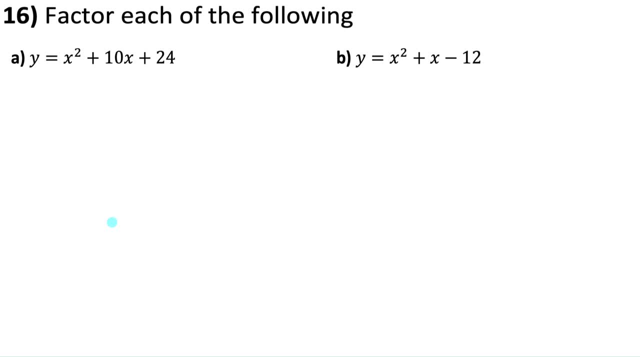 part a. i have a three term quadratic. the coefficient of that x squared term is 1, which means i can do product and sum factoring the short way. so i just have to find numbers who have a product of the c value 24 and a sum of the b value 10.. the numbers that 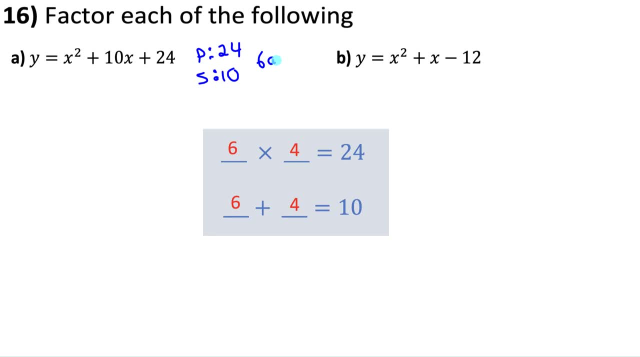 multiply to 24 and add to 10 are 6 and 4.. since the coefficient of the x square is 1, i can go right to my factored form equation by just adding 6 and 4 to x in both of those factors. so x plus 6 and x plus 4 are my factors. part b is very similar. 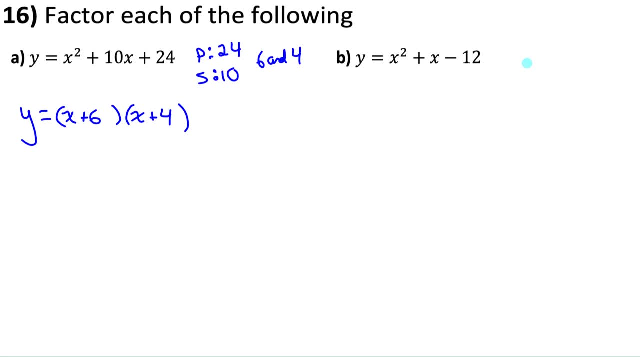 three term quadratic coefficient of x squared is 1.. so i just need to find numbers that have a product of the c value negative 12 and a sum of the b value, which is 1.. and the numbers that satisfy that product and sum are 4 and negative 3.. so once again, what i do is i can go right to. 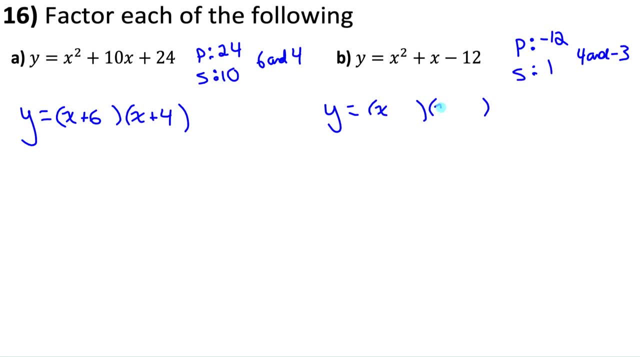 my factored form equation by adding those two numbers to the x-axis. and i can go right to my, to the x's in each of these factors, so x plus 4 and x plus negative 3, which we would just write as x minus 3.. part c, three, term quadratic, but the leading coefficient, the coefficient of the, 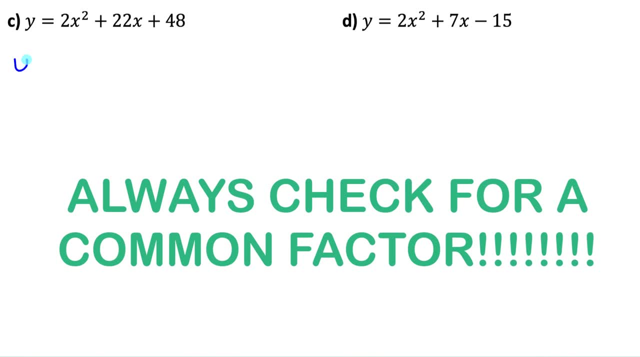 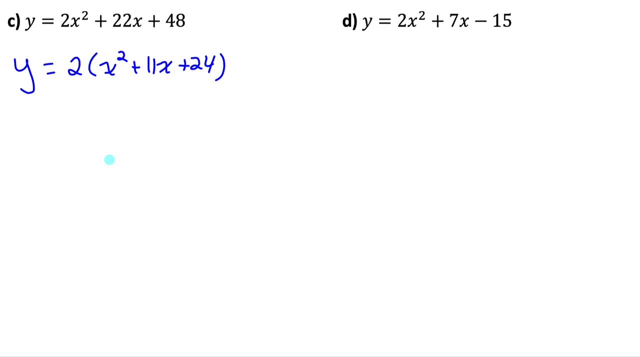 x squared is not 1.. so what we should do is we should check if it can common factor out, and it can in this case. 2 divides evenly into 22 and 48. so let's common factor out the 2 by dividing all three terms by 2 and putting it out front. so x squared plus 11, x plus 24 is my second factor. 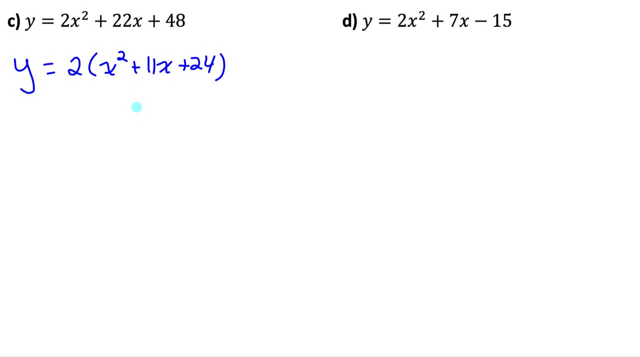 now we're just going to look inside the brackets here at this quadratic and we're going to try and factor that the coefficient of the x squared is now 1.. so we're just looking for numbers that have a product of the c value 24 and a sum of the b value 11.. the numbers that work are 8 and 3.. 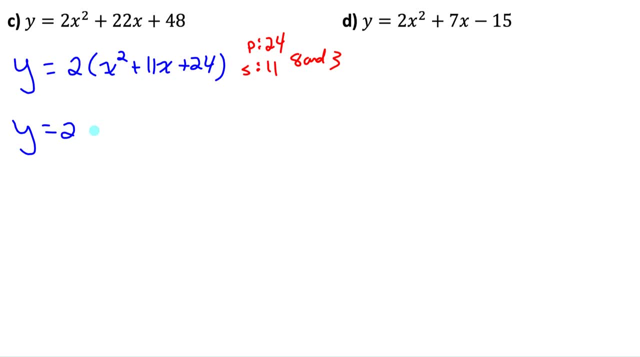 so we can factor what's in the brackets to x plus 8 times x plus 3.. just don't lose that 2 that was out front at the beginning. so don't lose that 2 that was out front at the beginning of the equation. 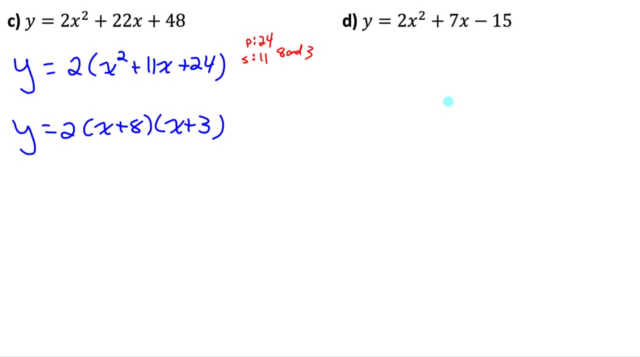 Part D, a three term quadratic that we want to factor. the coefficient of the x squared is not 1, it's 2, but this time we can't common factor out a 2,. 2 doesn't divide evenly into 7 and negative 15, so we can't common factor it out, so we have to factor this the long. 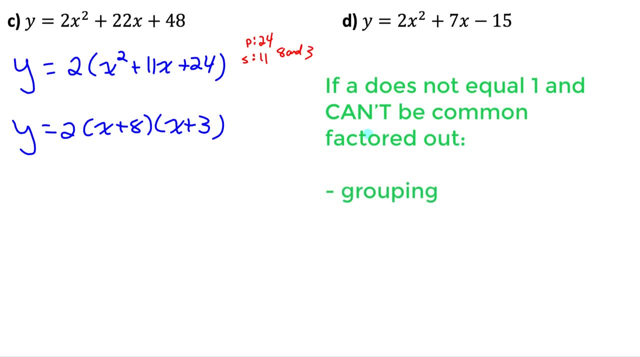 way. Some teachers may call it by grouping, some by decomposition or just the long factoring method. But whatever you call it, we're looking for numbers that don't just have a product of the c value, now a product of a times c, so a product of 2 times negative, 15 is. 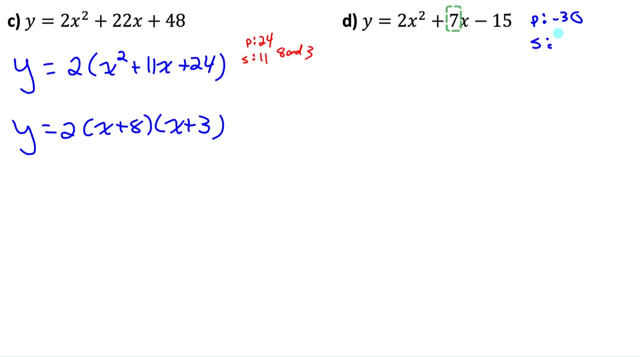 negative 30, and a sum of the b value 7.. So the numbers that work in this case are 10 and negative 3.. And since the leading coefficient is not 1, we can't go right to our factors. What we need to do is split the middle term into 10x minus, 3x, 2x squared plus 10x minus. 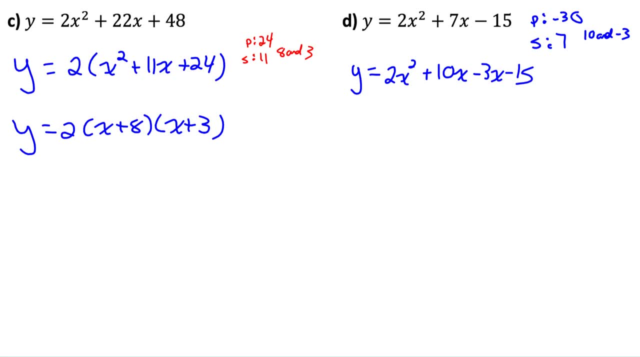 3x minus 3x. So I rewrote the equation, but I rewrote 7x as 10x minus 3x and specifically those two numbers, because those are the numbers that satisfy the product and sum. And now we factor it by grouping. We look at the first two terms and take out a common factor from. 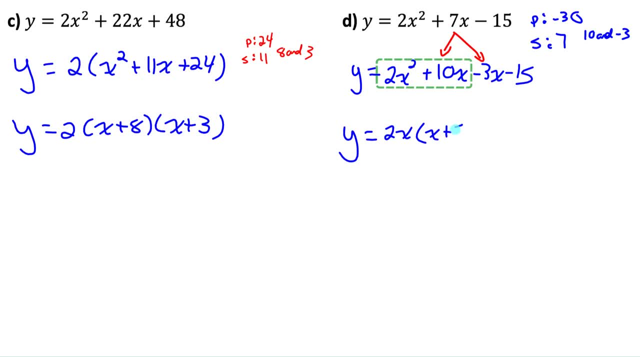 the first two. so I could take out a 2x and that would leave me with x plus 5.. And then I look at the last two terms- negative 3x minus 15, and I take a common factor from those last two terms. I could take a negative 3 from both terms and that would leave me. 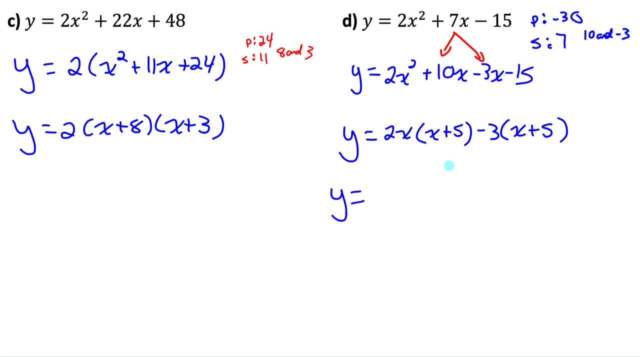 with, once again, x plus 5.. And now that we have a common binomial- they both have that x plus 5, we can factor out that x plus 5, and be left with 2x minus 3e- Once again a quadratic leading coefficient. 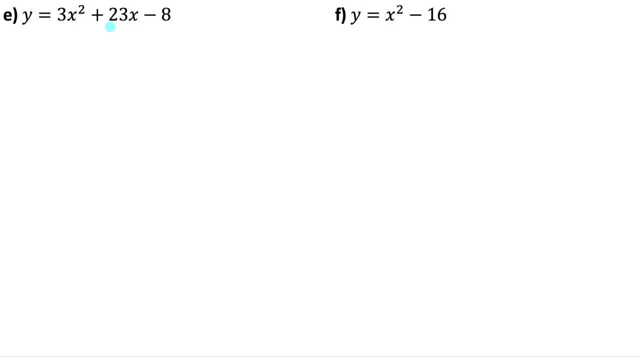 is not 1, and you can't common factor it out. 3 doesn't divide evenly into 23 and negative 8. So we're going to have to factor it the long way by decomposition and grouping. So I want a product of a times c, 3 times negative- 8 is negative 24, and a sum of the b value. 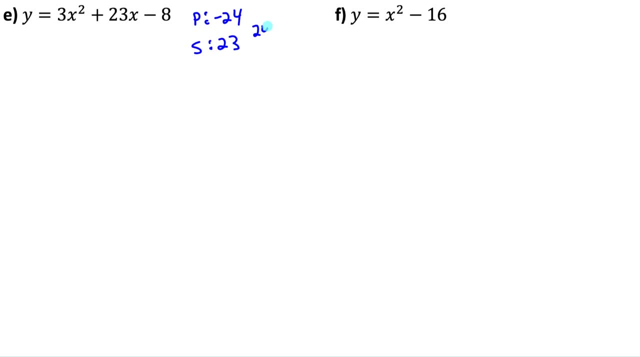 which is 23.. The numbers that satisfy that product and sum are 24 and negative 1.. So I need to split the middle term into 24x minus 1x And now I factor by grouping. If I look at the first two terms and take out a common factor, I 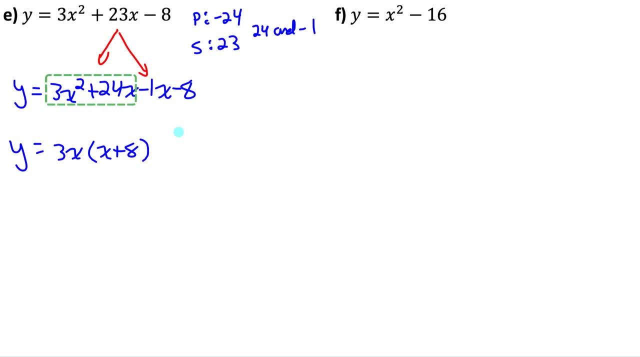 can take out a 3x and be left with x plus 8.. The last two terms: I take out a negative 1, and I'm left with x plus 8.. I see that common binomial. that's how I know I'm doing. 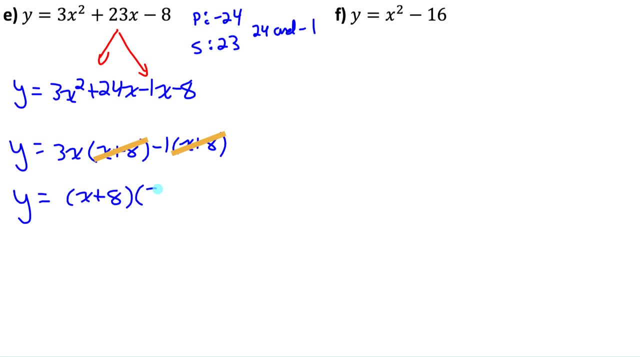 it right. Take out that common binomial and you're left with 3x minus 1 as your second factor, f is a special product. It's a difference of squares. I have an x squared minus a 16. And 16 is a perfect square number: It's a 4 squared. So if you have a difference of 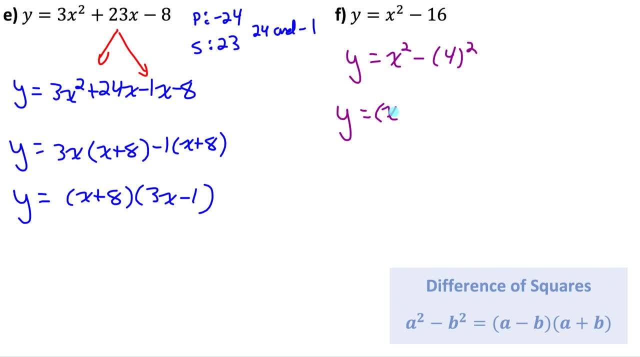 two perfect square numbers. it factors to x minus 4 times x plus 4.. g is another difference of squares. I have 4x squared minus 25.. Well, this one's a little trickier because in order to think of the first term as a perfect square number, we'll think of the first term as a 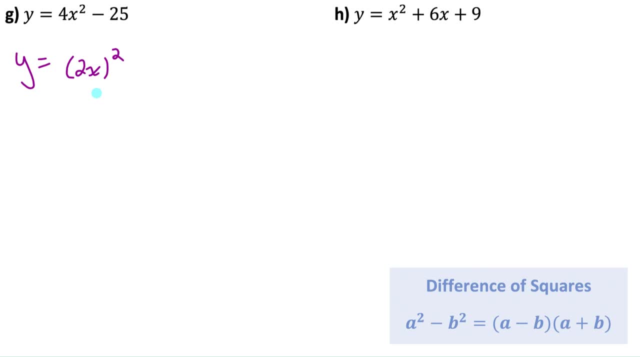 perfect square number. So let's think of it as a 2x that's being squared. If we square the 2 and the x, we get 4x squared, Minus 25 is 5 squared. And now that I see it's a difference of squares. 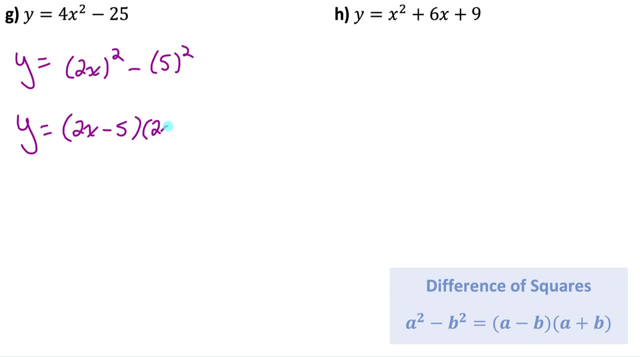 I know it factors to 2x minus 5 times 2x plus 5.. Part h is actually what we call a perfect square trinomial, and that's because it's the same number twice that satisfies the product and sum. The coefficient of this is 1, so I just need to find numbers with a product of c which. 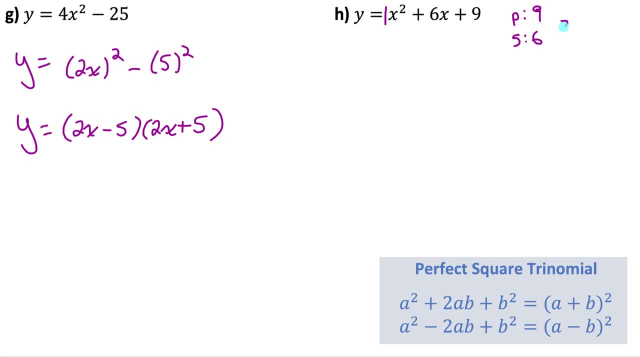 is 9.. And a sum of b which is 6. And the numbers that work are 3 and 3.. So this would factor to x plus 3 times, another x plus 3, which you would never write it twice. 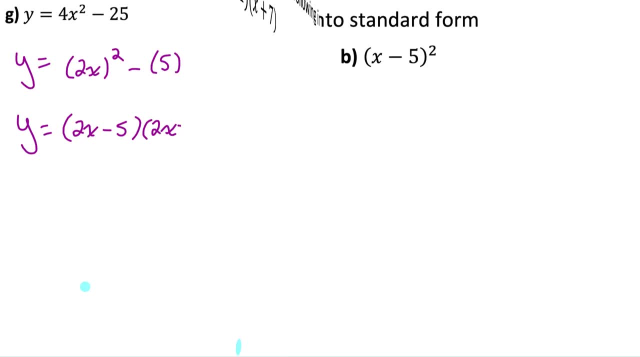 You would just write it as x plus 3 squared. Let's go backwards. now, Instead of factoring, let's expand. Example 17 says: expand each of the following into standard form. So I'm going to have to do my double distributive property, sometimes called FOILing Multiply. 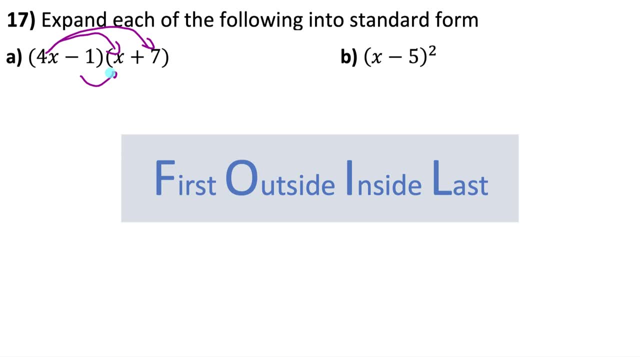 the first terms, The outside terms, the inside terms and the last terms. That's why it's called FOILing. And if I write all four of those products, so 4x times x is 4x squared, And then 4x times 7 is 28x. 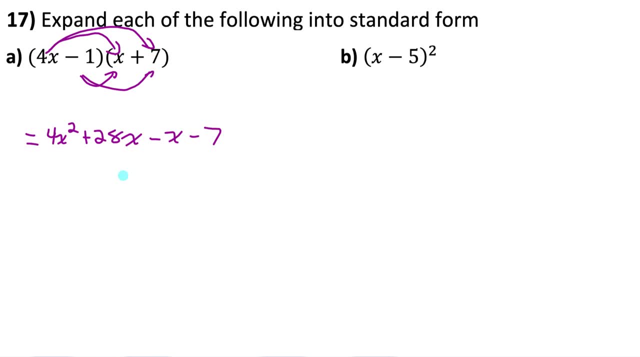 Negative 1 times x is negative x and negative 1 times 7 is negative 7.. Collect my like terms. My only like terms are 28x minus 1x, which is positive 27x. Expanding part b is probably the most common mistake people make in the grade 10 math course. 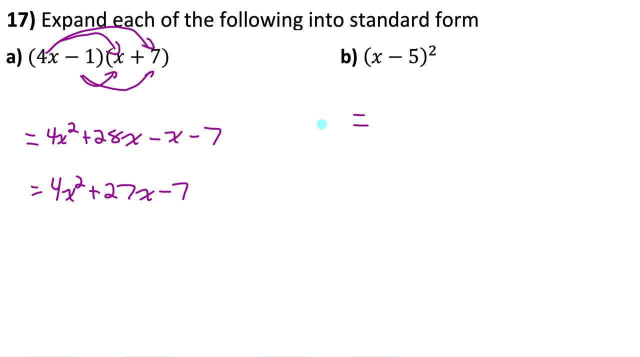 x minus 5, all squared is not just x squared minus 5 squared. You can't put the squared on both terms. You actually have to FOIL it out. You have to do x minus 5 times another x minus 5.. 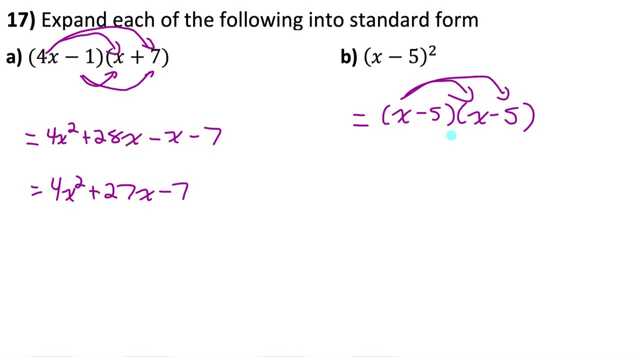 Rewrite it like that and then do your double distributive property and when you do all four products you'll see what you get. x times x is x squared. x times negative 5 is negative 5x, Then negative 5 times x is. 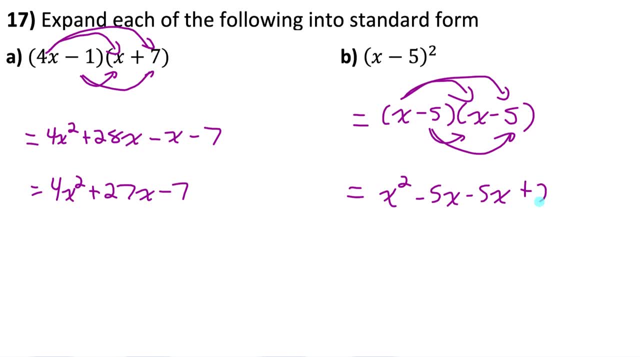 another negative 5x And then negative 5 times negative 5 is positive 25.. If I collect my like terms, the middle two terms, negative 5x minus 5x, is negative 10x, And there it is expanded. 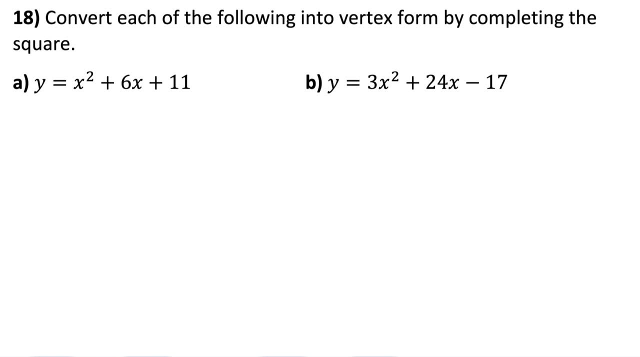 Okay, question 18,. I want to get these standard form quadratic equations into vertex form quadratic equations. The process for doing that is you start by putting the first two terms in brackets and then you common factor out the coefficient of the x squared from. 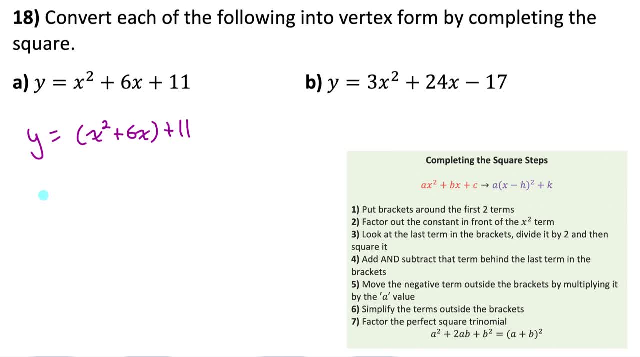 the first two terms, but it's just one in this first example, so I don't have to do anything After that. what we do is we add and subtract a special number inside the brackets. So I need to add and subtract a certain number inside the brackets here. 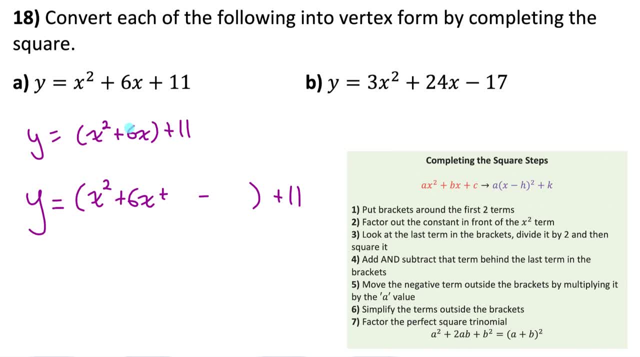 Now what number goes here and here? you always do half of this number and then square it and then put that in these two spots. So half of 6 is 3,, square it and we get 9.. So we add 9, and subtract 9.. 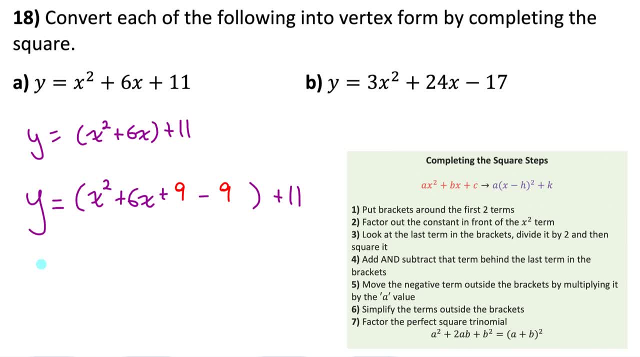 Really, we added 0, right, 9 minus 9 is 0, but that's the step That creates a perfect square trinomial, which is going to help it factor very nicely into vertex form. Before I can factor it, though, I need to get this negative 9 out of the brackets. 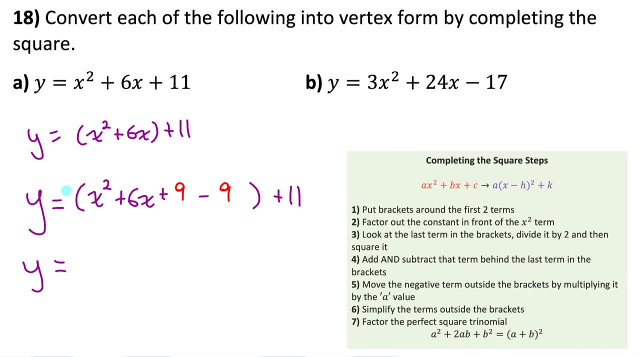 I don't really want it in there. So you have to get it out by multiplying by whatever's in front of the brackets, which in this case is just 1, so really we're just moving the negative 9 out. So I have x squared plus 6x plus 9.. 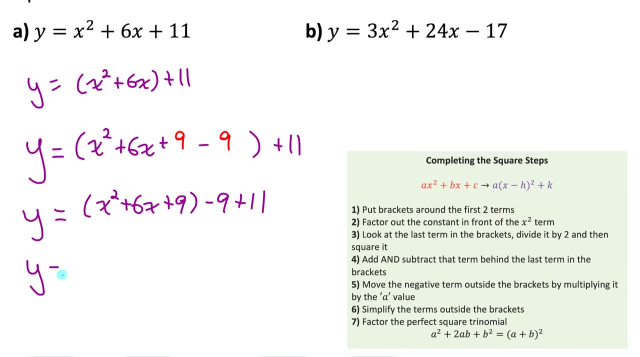 Negative, 9 moves out. Now I just have two things left to do. Factor this quadratic. So what numbers multiply to 9 and add to 6? Are 3 and 3.. So it goes to x plus 3 times another x plus 3, which is x plus 3 squared. 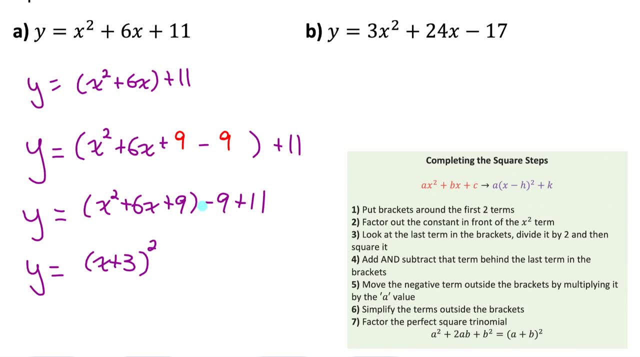 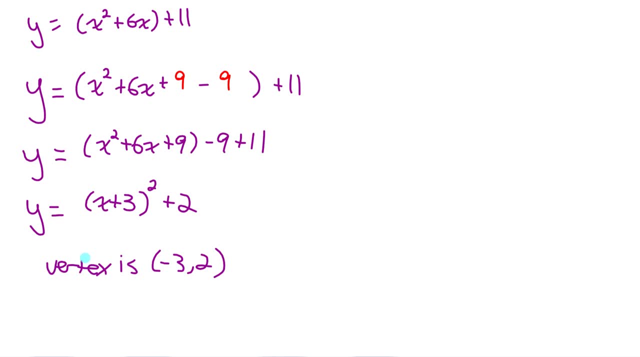 We very intentionally created it so that it would do that. And outside the brackets, negative 9 plus 11 is positive 2.. So my vertex is: negative 3, 2, and since the a value is positive 1,. I know the parabola. 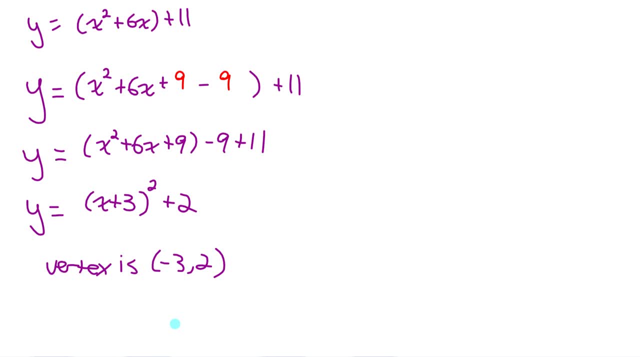 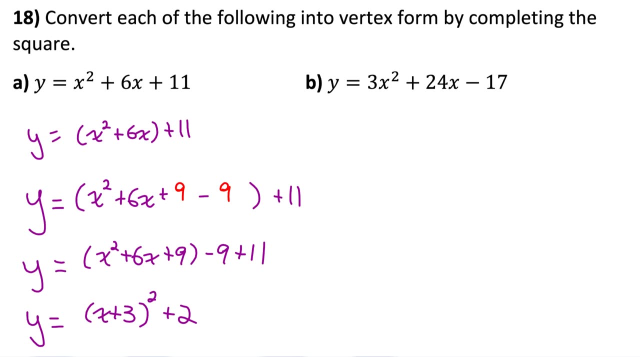 opens up, which means the vertex is at the bottom. so the vertex is a min. So the vertex is a min point. Let's do the question again, but part b, A little more difficult this time. Same steps. Put the first two terms in brackets. 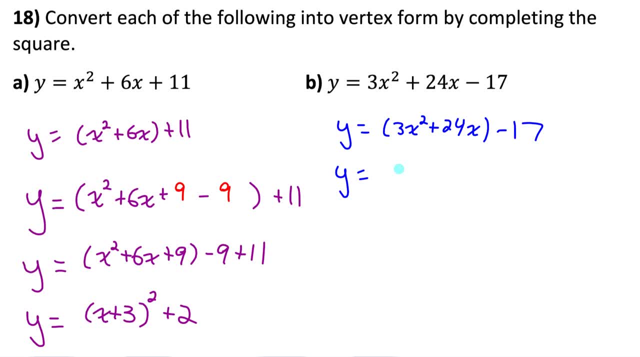 Step 2.. Whatever the coefficient of the x squared is common, factor it out from the first two terms that are in brackets, So I'll put the 3 out front. divide both of the terms in brackets by 3, I get x squared. 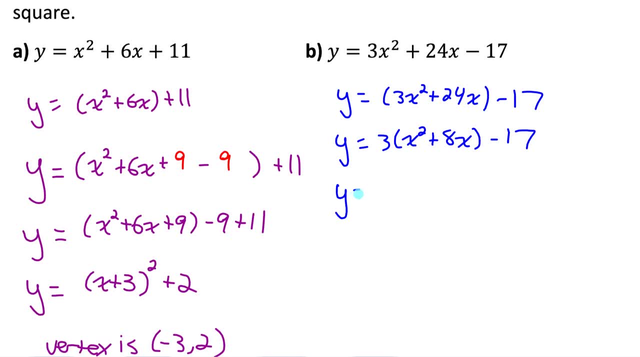 plus 8x. And now what we do is, inside the brackets, same thing. we want to create a perfect square trinomial by adding and subtracting half of this, 8 squared Right. You always look at this number, take half of it and then square it. 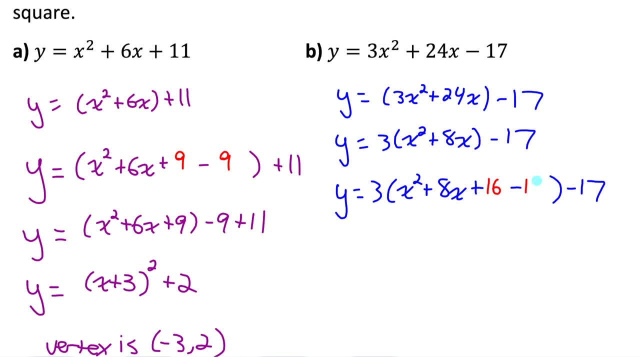 So half of 8 is 4, 4 squared is 16.. So I'm going to add and subtract 16.. We don't want that negative 16 in there, so I take it out of the brackets by multiplying it by whatever's in front. 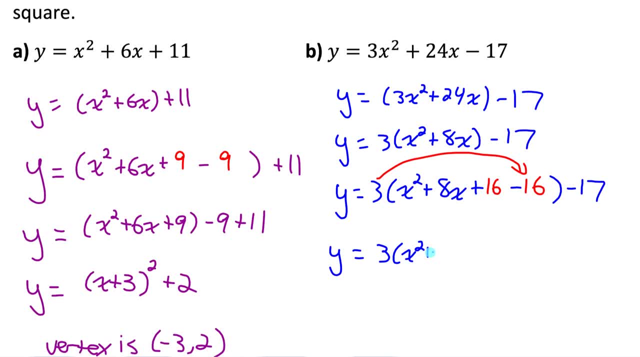 So I have: y equals 3x squared plus 8x plus 16.. Outside of the brackets, this negative 16 is being multiplied by 3, so it's negative 48.. We just have to factor the quadratic. The numbers that multiply to 16 and add to 8 are 4 and 4, so it factors to x plus 4 times. 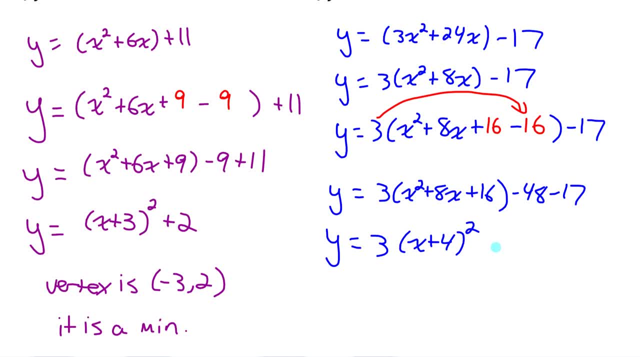 another x plus 4, which we write as x plus 4 squared, And then if I do negative 48 minus 17,, I get negative 65. So my vertex is negative 4,, negative 65, and because the a value is positive, I know the. 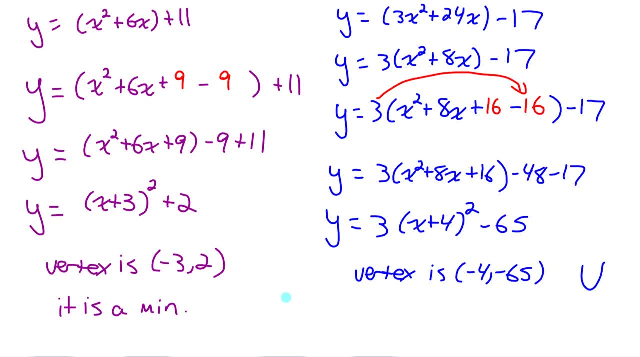 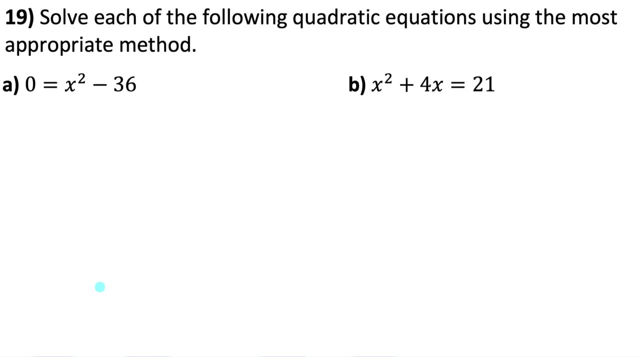 parabola opens up, which means the vertex is at the bottom. so once again it's a min point. Almost done with quadratic, so let's just solve some equations. So when solving quadratic equations you always want to get it into factored form, set each. 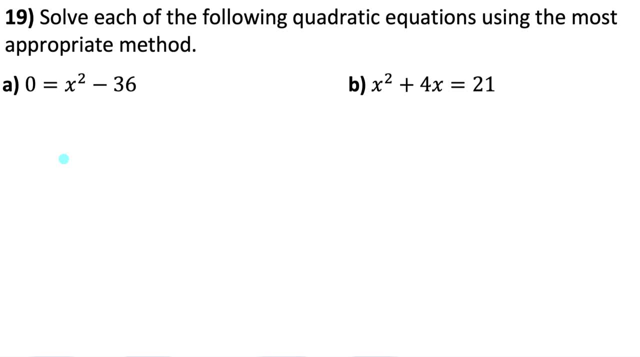 factor to 0, and solve each of those equations you make. So the first one's a difference of squares. It's an x squared minus 6 squared. so I know that factors to x minus 6 times x plus 6.. And how can this equation be true? 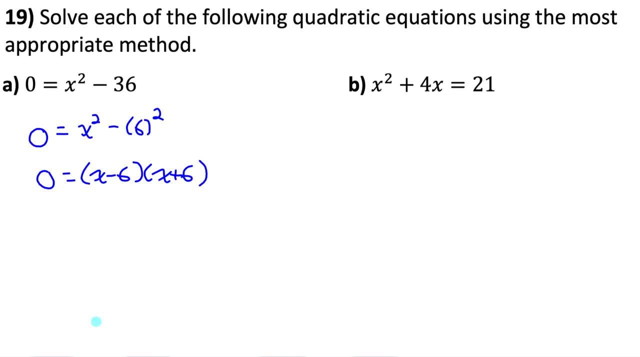 Is, if either of the factors were 0, it would make the whole product be 0,, making the whole equation true. So set each factor to 0,, set x minus 6 equal to 0,, set x plus 6 equal to 0, and solve both. 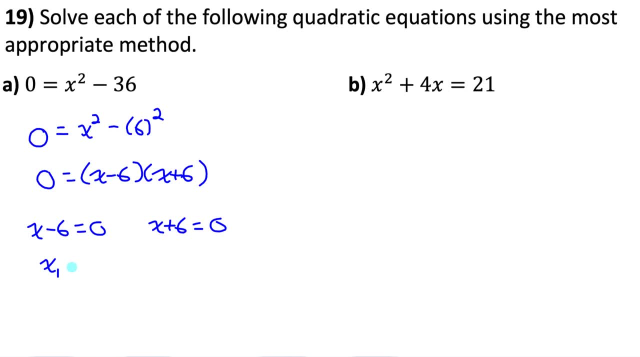 of those equations you made. So I get a first answer: x is 6, and my second answer is x equals negative 6.. These are both answers that satisfy the original equation. This one, this one's not set to 0 to start with, so we should always start by doing that. 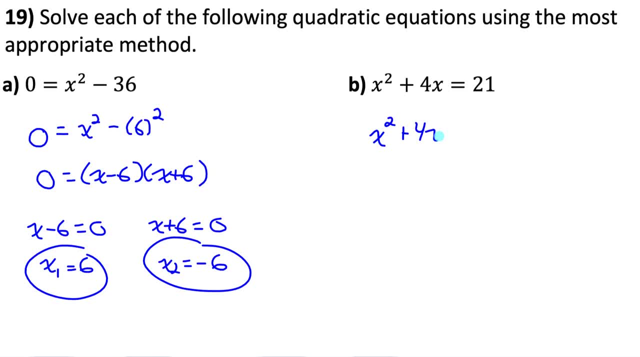 If you have a quadratic, start by setting it to 0.. So x squared plus 4x minus 21 equals 0.. Now we want to factor it, so I'd be looking for numbers that have a product of negative 21 and a sum of 4, and since the coefficient of the x squared is 1,, I'm going to be able. 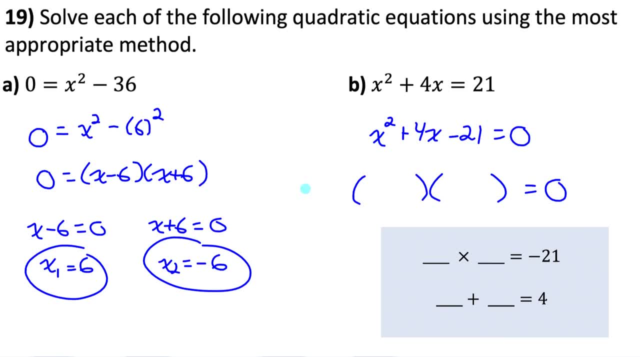 to go right to my factors, once I find the numbers that satisfy that product and sum. So the numbers that satisfy the product and sum are 7 and negative 3, so they go in those two spots. And now to find how the product of these two things could be 0 is if either of those two 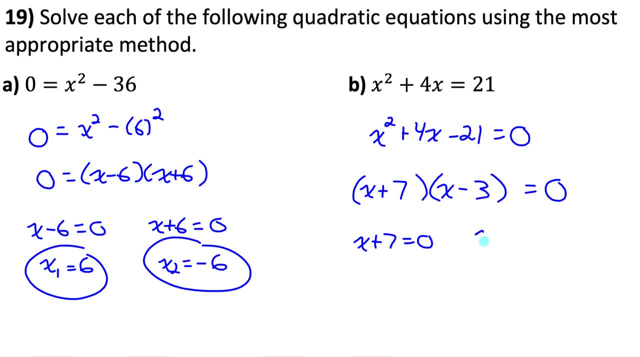 things were equal to 0. So set both the factors equal to 0. And solve both of those equations. My first answer is negative 7, my second answer 3.. See, it's set to 0, the coefficient of the x squared isn't 1, it's negative 1, which? 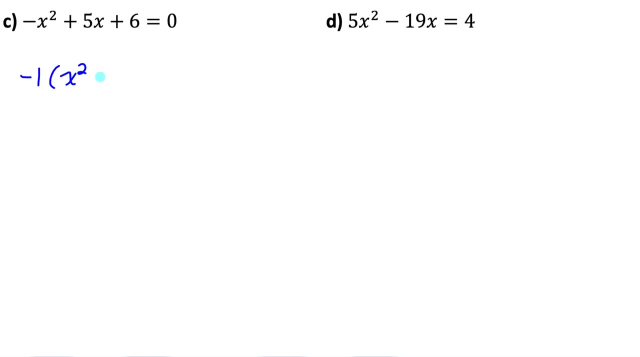 I don't really like, so I'm going to common factor that out. So divide all three terms by negative 1, it just changes the sign of all of them. And now in the brackets is a quadratic with a leading coefficient of 1, so I would just 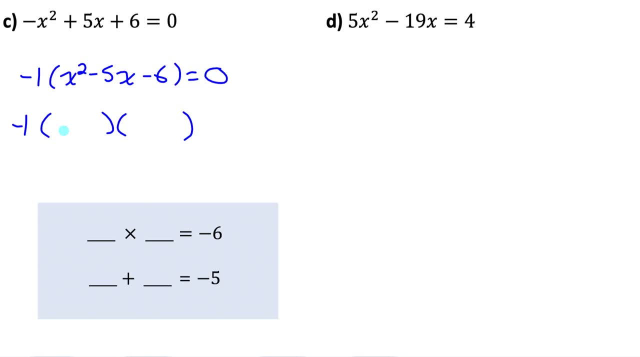 need to find the numbers that have a product of negative 6 and a sum of negative 5, and put those numbers added to x, So those numbers would be negative 3.. And now I'm going to find the numbers that have a product of negative 6 and a sum of. 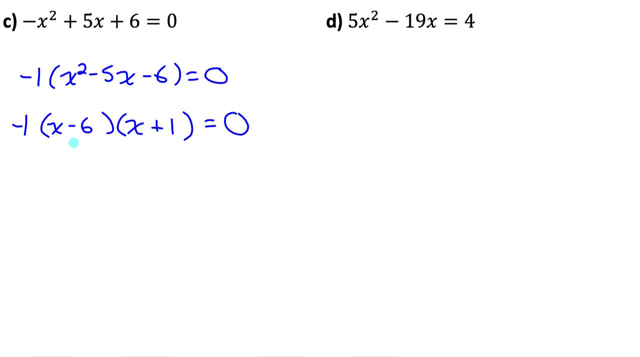 negative 1.. And now this product is 0, if any of the factors are 0. So set the factors that involve an x equal to 0, and solve each of those equations And solve for those two cases. So I get 6 and negative 1 for my two answers. 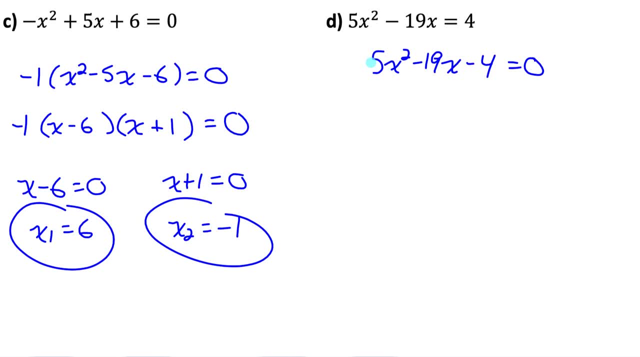 This one. start by setting it equal to 0.. I can't common factor out that 5, so I'm going to have to factor this the long way. The numbers that multiply to 5 times x are equal to 0. The numbers that multiply to 5 times negative 4, so I have a product of negative 20, and 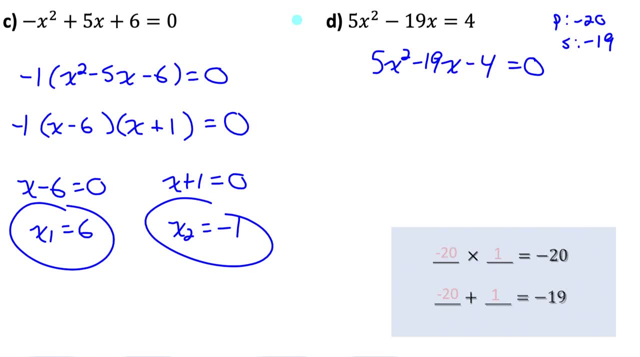 a sum of the b value negative 19,. well, that would be negative 20 and 1.. So I'll split the middle term into negative 20x plus 1x. And now I'll take a common factor from the first two terms. I'd take out a 5x and I'd 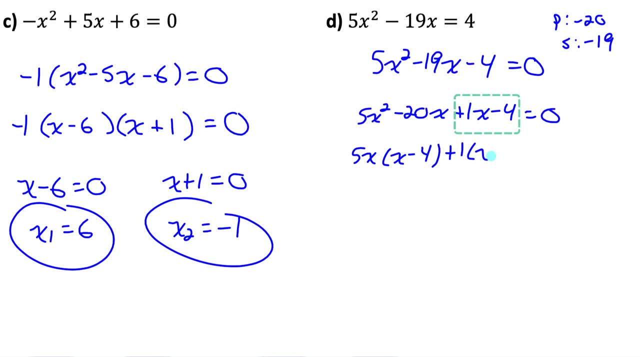 have x minus 4.. From the last two terms I can just take out a 1, which leaves me with x minus 4.. I have that common binomial of x minus 4, when I take that out, I'm left with 5x minus. 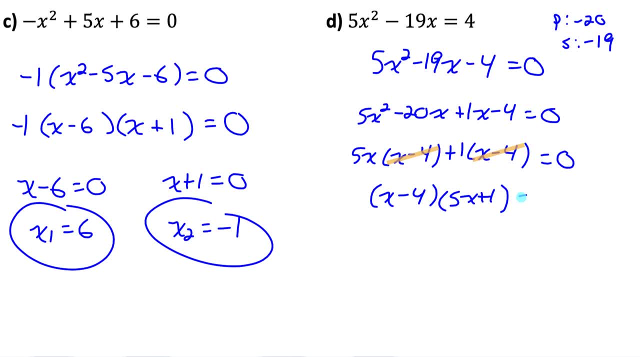 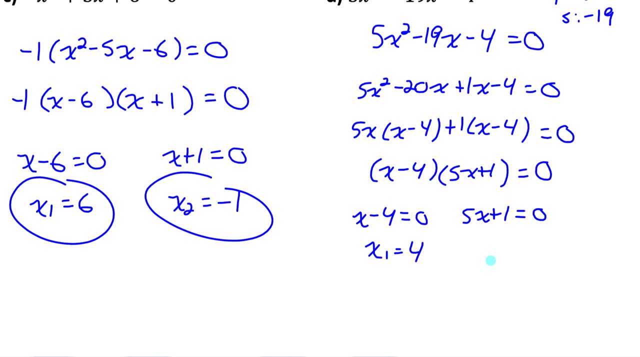 4.. So I'm left with 5x minus 4.. 5x plus 1.. And now I set each factor to 0, and solve each of those equations. I get 4, and this one's a two-step one to solve: subtract the 1 over and then divide. 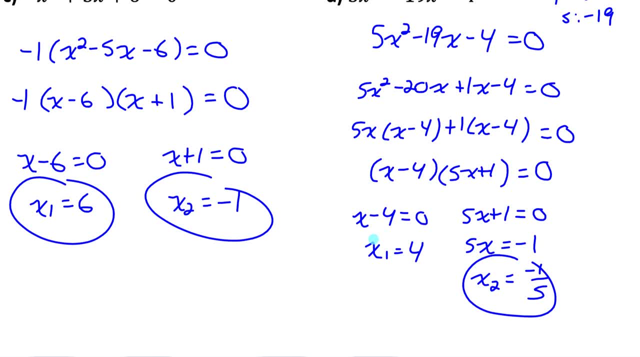 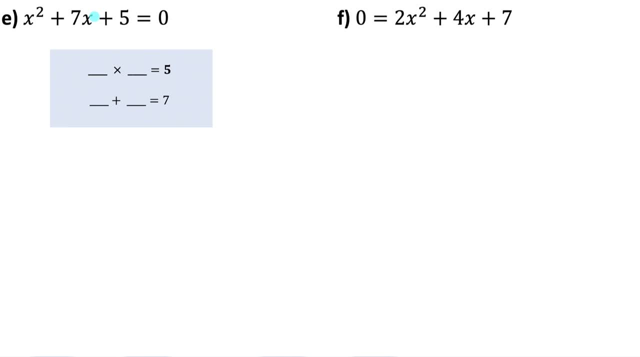 the 5.. My second answer is negative: 1 over 5.. Two more to solve. Notice the first four I solved by factoring. These ones actually aren't factorable. there's nothing that multiplies to 5 and adds to 7.. 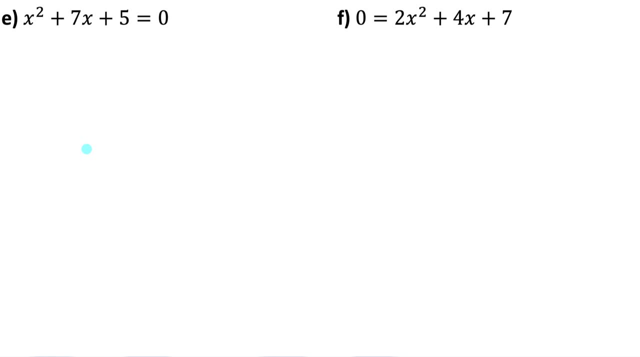 So we can't factor it. but that doesn't mean there's no solutions. it just means there's no rational solutions. There may be some irrational ones. so we need quadratic formula to check. So if I use quadratic formula, x equals negative b, so negative 7, plus or minus the square. 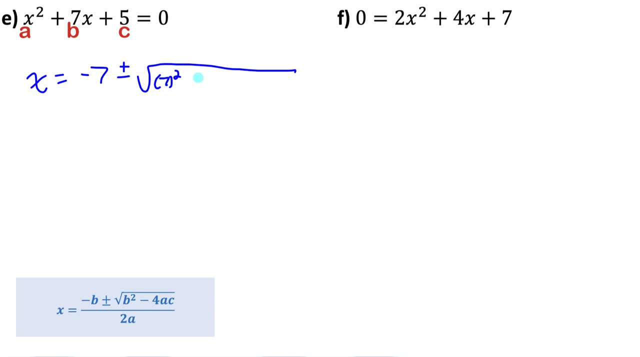 root of b squared, so 7 squared minus 4 times a times c, and this is all over 2 times a. Now I recommend to simplify underneath the square root. first, because we call that the discriminant, And that's going to reveal to us how many answers we're going to get. 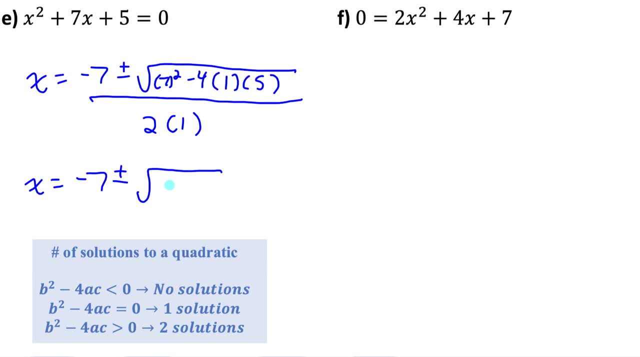 So 7 squared is 49, minus 20,, that's 29.. So I have root 29.. Okay, since I got a positive discriminant, that means I'm going to get two answers here, So I'll split them into my two answers. 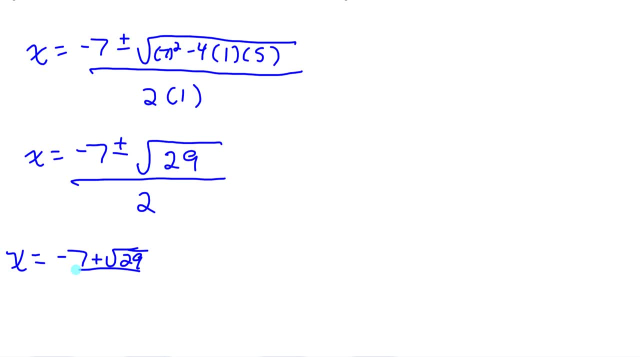 I've got negative 7 plus root 29, over 2.. And I also have x equals negative 7 minus root 29, over 2.. Okay, I've got my two exact answers. So I'm going to get two decimal answers by evaluating on our calculator and rounding. 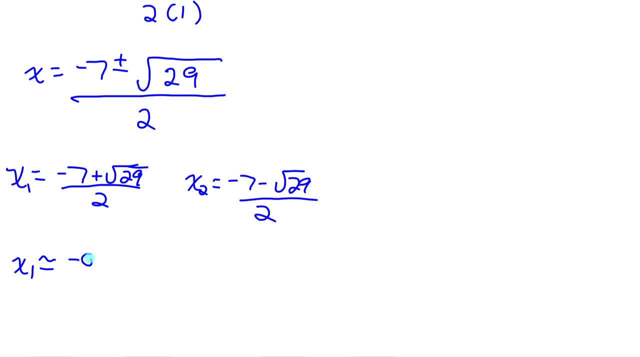 to two decimal places. The first one would give me negative 0.81, and the second one would give me negative 6.19.. If we look at f, I mean sometimes we can't get any answers. You'll see what I mean with this question. 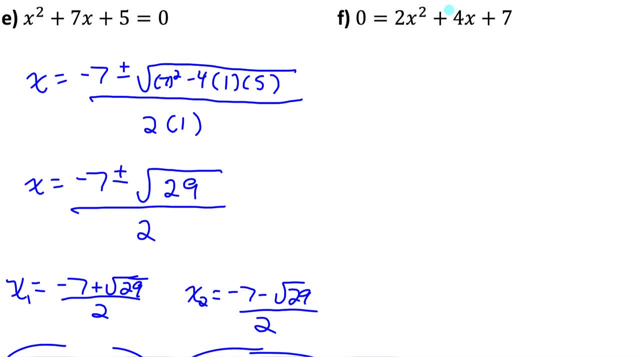 This one not factorable. There's no numbers that have a product of 14 and a sum of 4, so we can't factor it. So we try quadratic formula. x equals negative b, so negative 4.. Plus or minus the square root of b squared minus 4 times, a times c, all over 2 times. 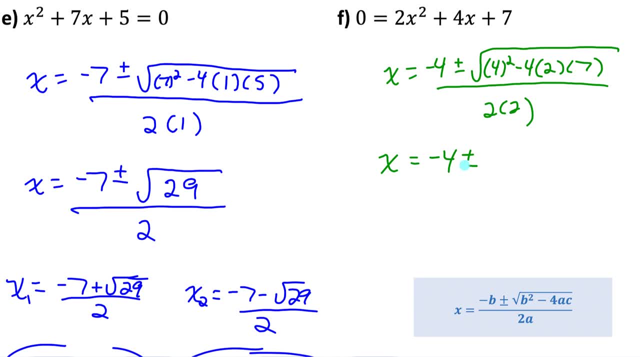 a The discriminant. if we simplify that, 16 minus 56, we actually get a negative answer. We get negative 40. So we've got the square root of negative 40. And you can't square root a negative. so this means we're not going to get any real solutions. 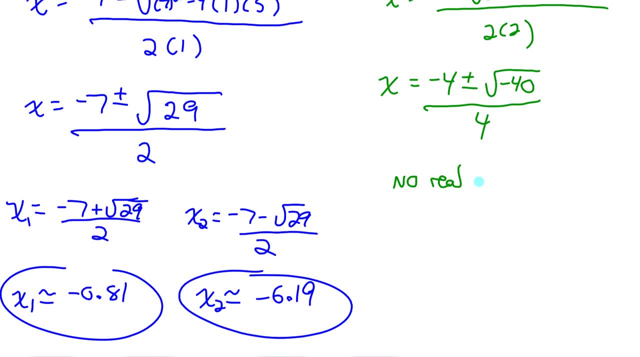 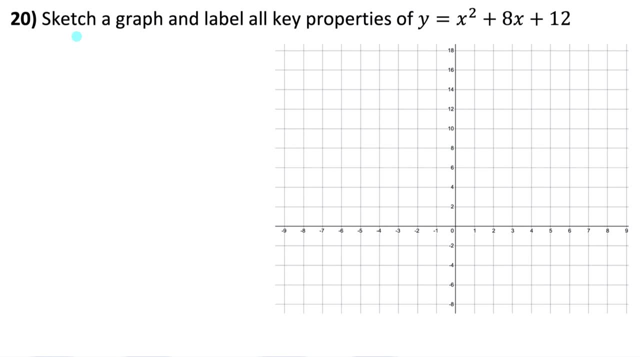 for this We're almost through the whole course 20.. Sketch a graph and label all key properties of x squared plus 8x plus 12.. So key properties would involve x-intercepts, vertex, y-intercepts. Well, from standard form I know the y-intercept: it's the constant value 12.. 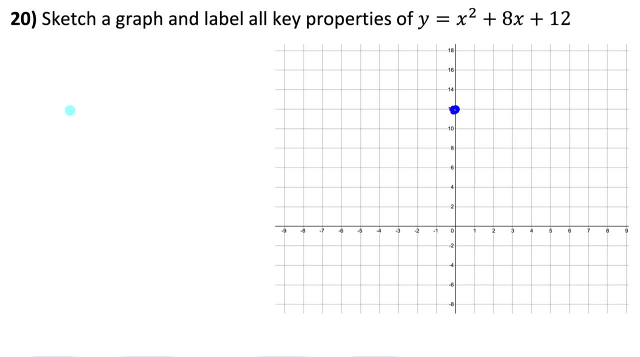 So I'll plot that right now. I know my y-intercept, I'm also going to want the x-intercepts, so I'm going to get this into factored form. The x-intercepts have a y-intercept. The x-intercepts have a y-intercept. 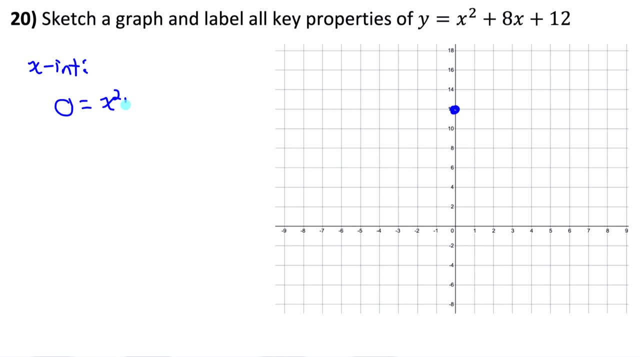 So I'm going to get this into factored form. The x-intercepts have a y-intercept, The x-intercepts have a y-intercept. The x-intercepts have a y-intercept, So I'm going to set y to zero. 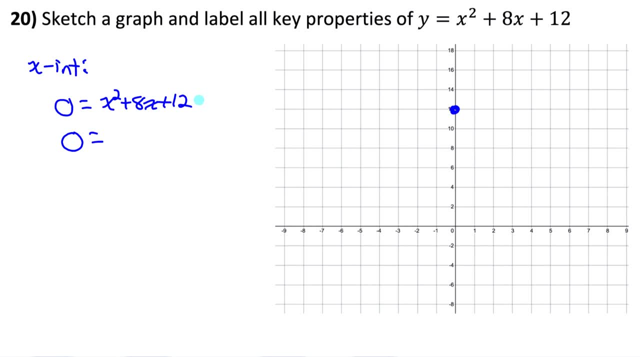 And now I'm going to solve this, and then that will give me the x-intercepts. So to solve it I'll have to factor it: What numbers are a product of 12 and a sum of 8?? Those numbers are 6 and 2.. 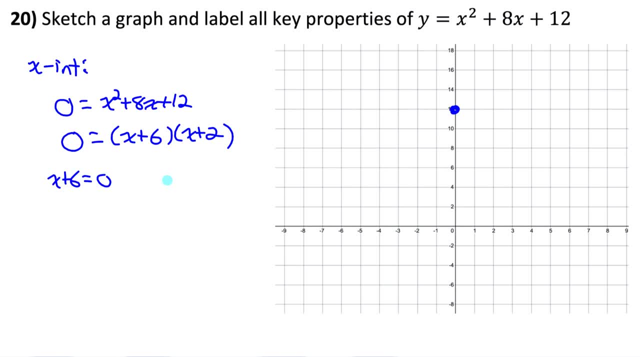 So there's factored form. The product would be 0 if either of the factors were 0. So set each factor to zero and solve, And I get negative 6 and negative 2.. So my x-intercepts are at negative 6 and negative 7.. 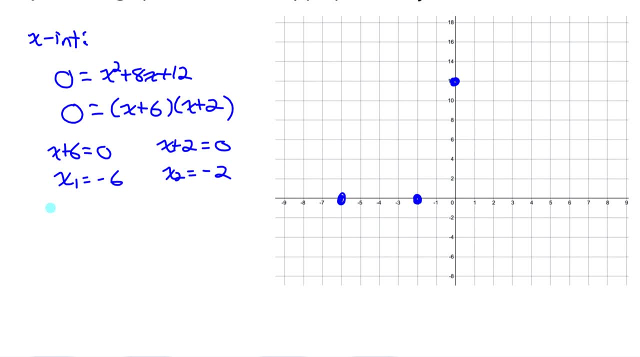 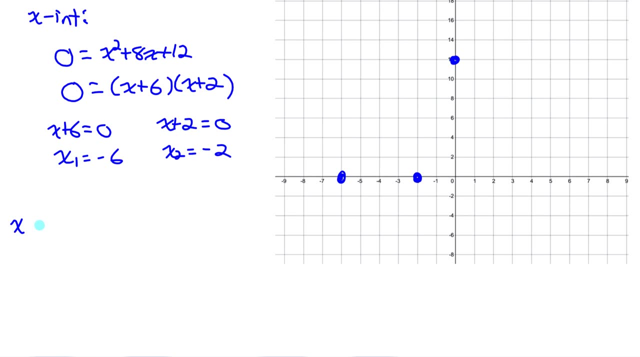 2. let me find the vertex now. well, I don't have to worry about putting this quadratic into vertex form, because I know the vertex is going to be halfway between the x-intercepts, because parabolas are symmetrical, so I can find the x-coordinate of the vertex just by finding the average of the x-intercepts. 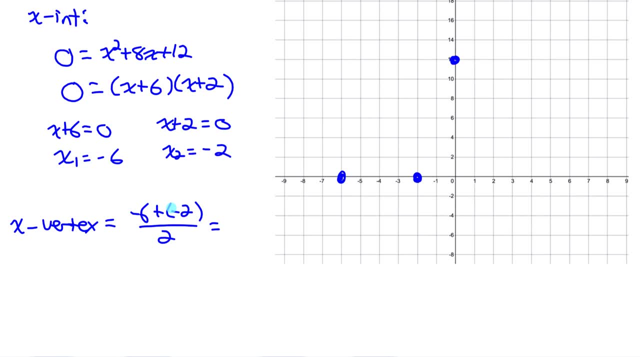 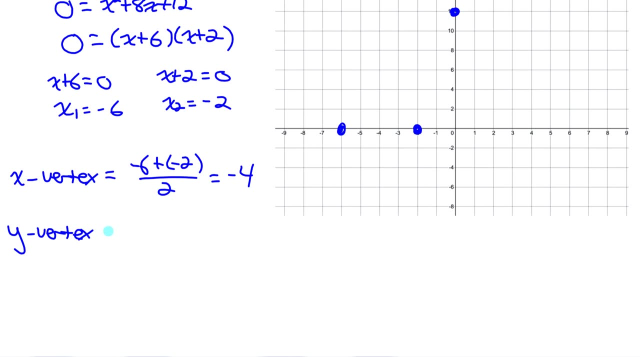 so add them and divide by 2. negative 8 over 2 is negative 4. the vertex is going to have an x-coordinate of negative 4. what's the y-coordinate of the vertex? just plug negative 4 into the original equation, so be negative 4 squared plus. 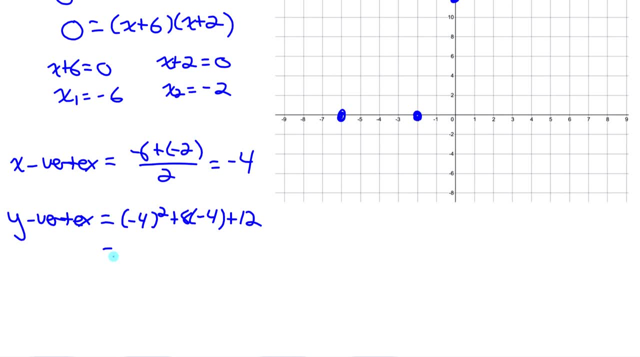 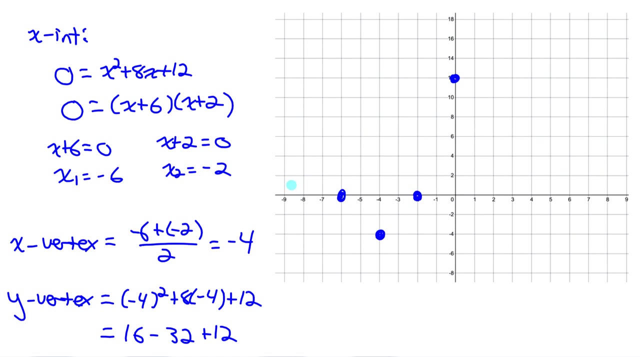 8 times negative. 4 plus 12, 16 minus 32 plus 12. hey, that's negative 4 as well. so my vertex is: at negative 4, negative 4. so that's this point right here. I might as well plot one more point, just because I know problems are symmetrical. if 4. 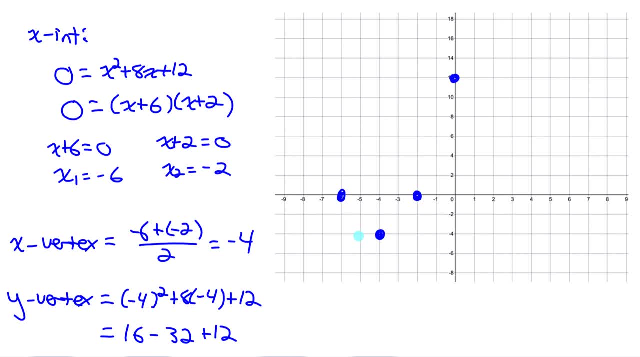 units to the right of the vertex right over here, and then I'm going to add y-coordinate of 12 for units to the left- 1, 2, 3, 4- we would also be at a y-coordinate of 12. so now I should be able to draw a fairly accurate sketch of. 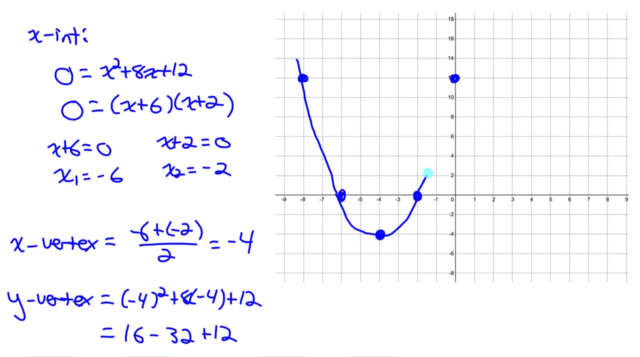 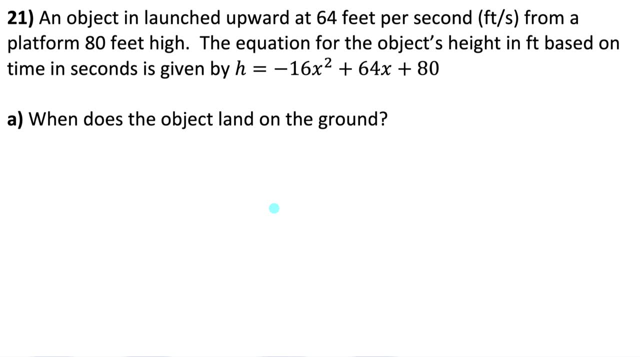 this parabola, making sure I go through all of these key points here and have that good U shape. and there we go. last quadratus question is an application question. an object is launched upward at 64 feet per second from a platform 80 feet high. the equation for the objects height and feet is based on time in. 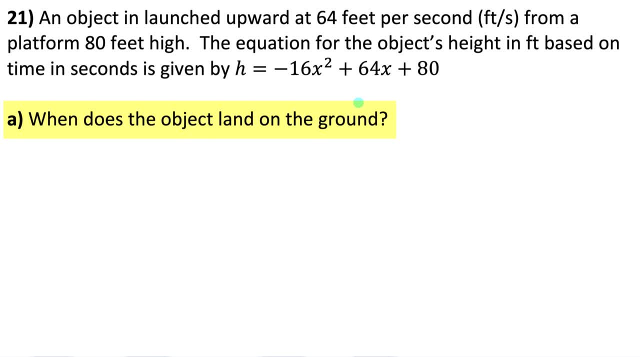 seconds given by this equation. when does the object land on the ground? anything. that time you see anything with the ground. that's the x intercepts, that's when the height is zero. so set the height to zero and solve. and to solve a quadratic that's set to zero, we factor it. so i'm actually going to 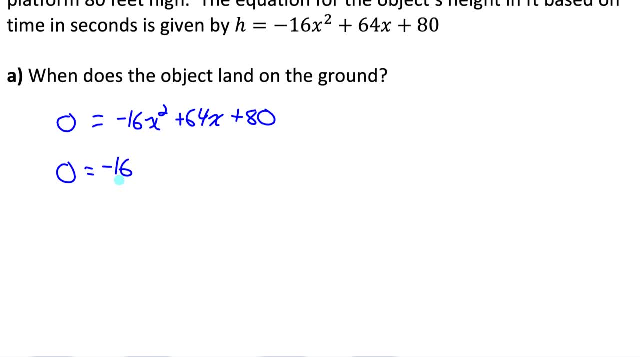 common factor out this negative 16 first, because i think it divides evenly into 64 and 80.. so let's divide all three terms by negative 16 and i would get x squared minus 4x minus 5.. and now this quadratic has a leading coefficient of 1, so i just have to find numbers that multiply to negative 5. 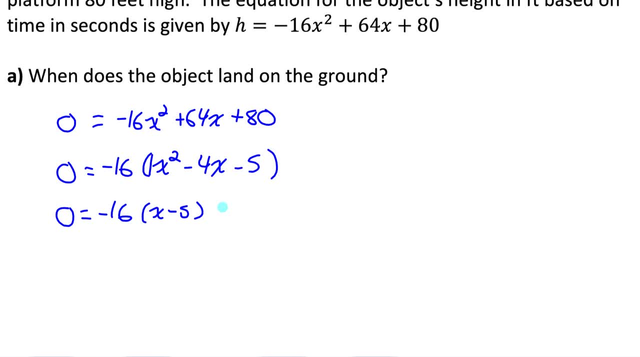 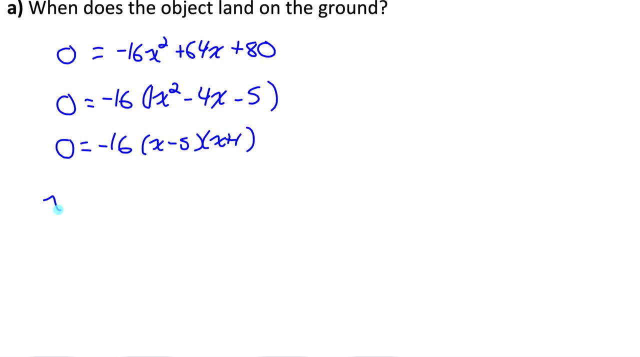 and add to negative 4, and those numbers are negative 5 and positive 1. so there's my factored form version of it. and now this whole product would be 0 if any of the factors containing an x was 0. so set each factor with an x to 0. 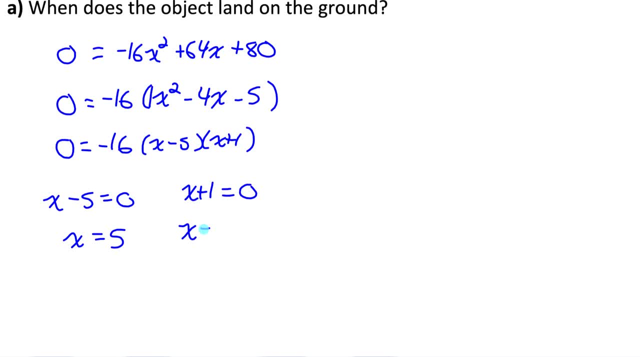 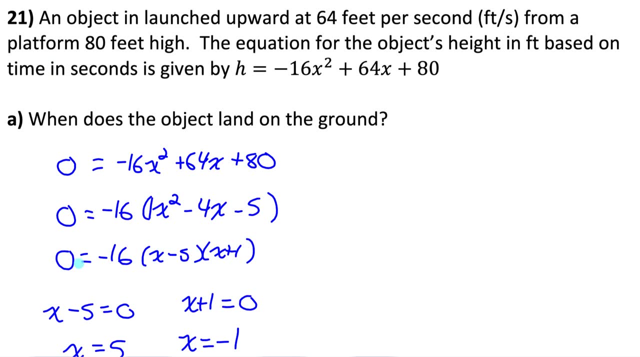 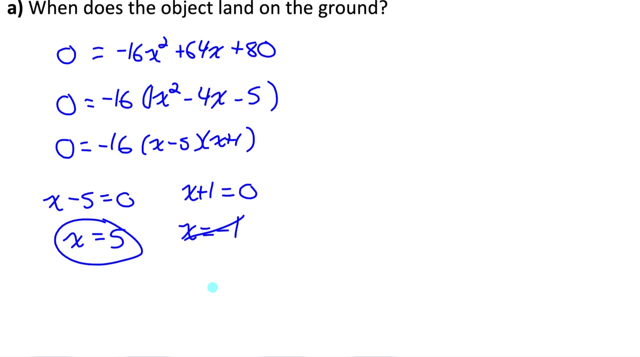 and solve, i would get 5 and negative 1.. now keep in mind: x in this equation actually stands for time in seconds. so we can't have negative time. so we can reject that answer and our only answer here is five seconds. so it'll hit the ground after five seconds. 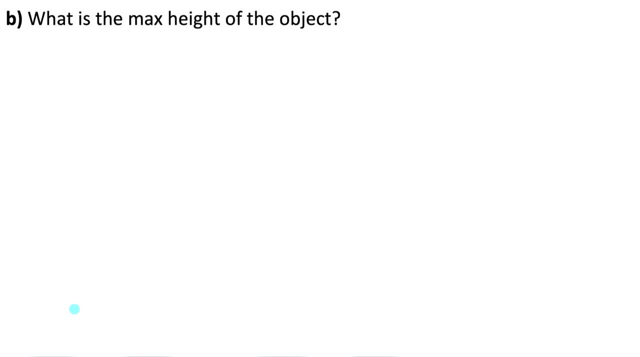 part b says: what is the max height of the object? well, the max. anytime you say anything about max or man, it's talking about the vertex. and what is the max height? it wants to know the y coordinate of the vertex. that's what we're looking for here. 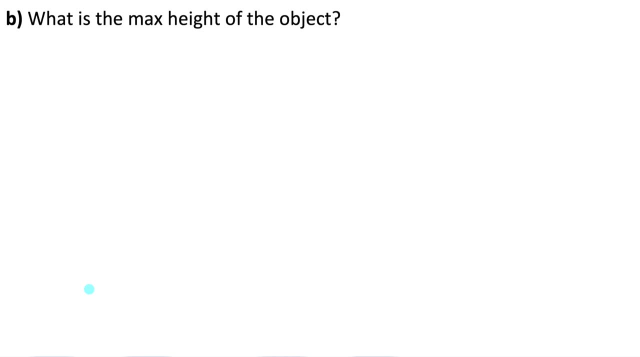 it's going to be easier for us to find the x coordinate first and then use that to find the max height. so i can find the x coordinate of the vertex by finding the average of the x intercepts. so the x coordinate of the vertex, i know it's going to be halfway between. 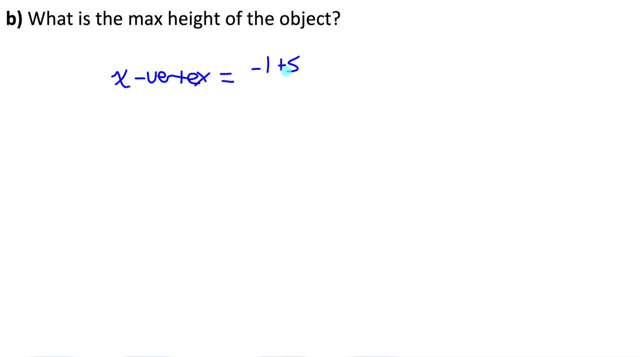 the x intercepts. so i just have to add them negative 1 and 5 and divide by 2.. that gives me 4 over 2, which is 2.. so the x coordinate of the vertex is 2 seconds and it's going to be at a max at 2 seconds. but what is the max height? let's find the y coordinate. 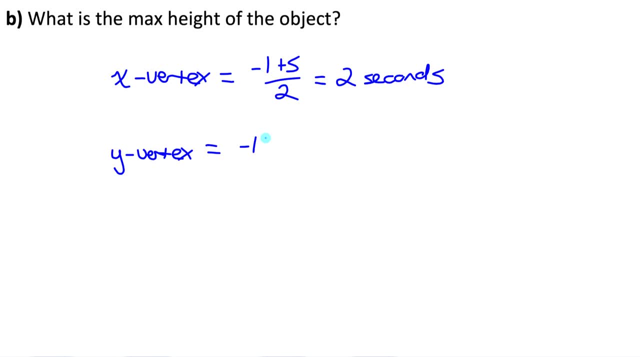 of the vertex by plugging 2 into the original equation. if i plug it into the original, negative 16 times 2 squared plus 64 times 2 plus 80. and if i evaluate this, i would get 144 feet. so my vertex is, at the point 2, 144.. the x coordinate is the time. the y coordinate is the. 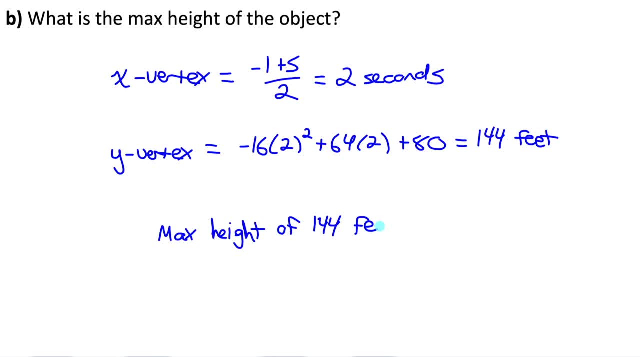 height. so the max height is 144 feet feet. Part C says: when is the object? 100 feet off the ground. So this one, we set the original equation, we set the height to 100. And then we need to solve this equation. So, in order to solve, 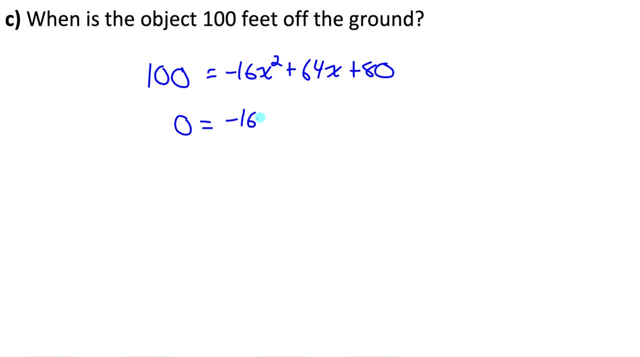 a quadratic, we have to set it to zero. So let's move that 100 to the other side. 80 minus 100 is negative 20.. And now to solve this, I can't common factor out that entire negative 16.. Because that. 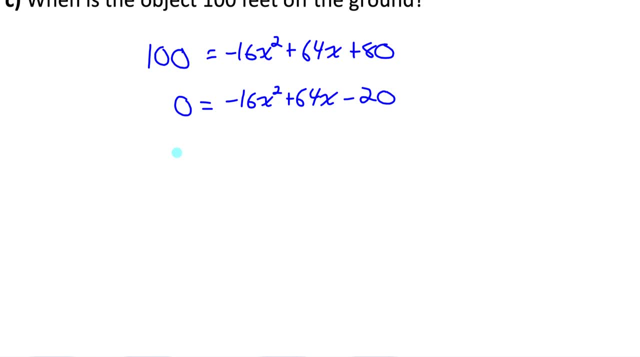 doesn't divide evenly into 20. But I can common factor out part of it. So zero equals. I can take out, let's say, a negative four from all three terms. I'll take our negative four, And that would give me four x squared minus 16 x plus five. And now are there any numbers that have? 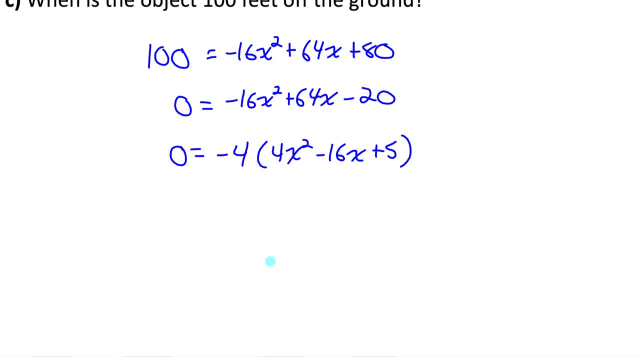 a product of four times five, so a product of 20 and a sum of negative 16?? I don't think so. So we'd have to use quadratic formula to see how this factor can be zero. So quadratic formula with that factor I would do. 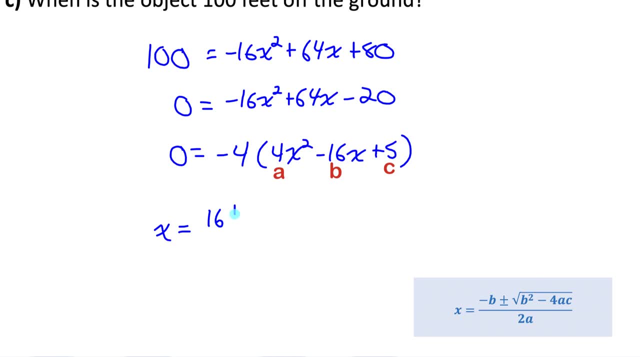 x equals negative b, so 16 plus or minus the square root of negative 16 squared minus, four times a times c, all over two times a. notice: this negative four is not part of the quadratic equation at all. all we're doing is trying to figure out how can this be zero, because that will make the whole 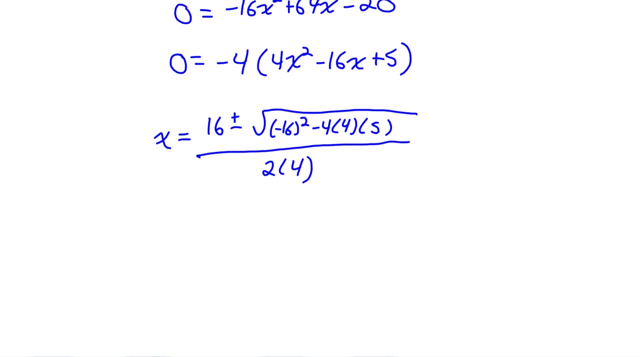 product be zero, which is what we want. And then if we simplify the discriminant underneath the square root, I would get 160 plus root 176.. And if I split this into my two answers, if I do 16 plus root 176 over eight. 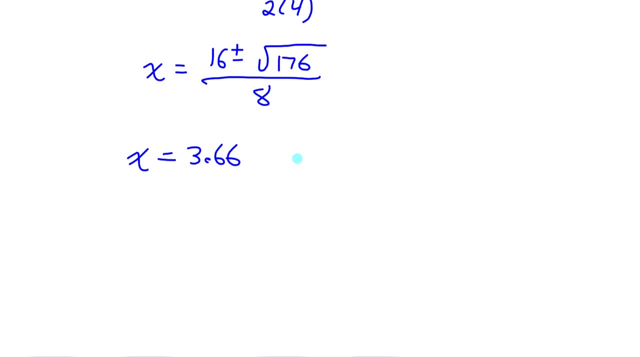 I get 3.66.. And if I do 16 minus root, 176, over eight, I get 0.34, I get two positive answers. So I get two times when it's at 100 feet. And if we think about, if we think about what it looks like, 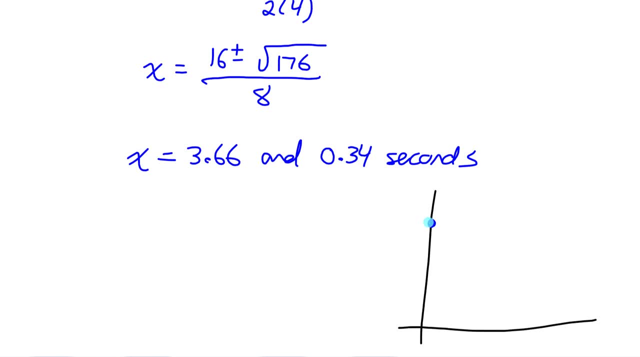 we know it has a y intercept of 80. That's the platform is, and then of course, it's going to go up and come back down. the highest it gets, we figured out, was 144.. this was at 2: 144 and this is at 0: 80, so it must be at a height of 100. 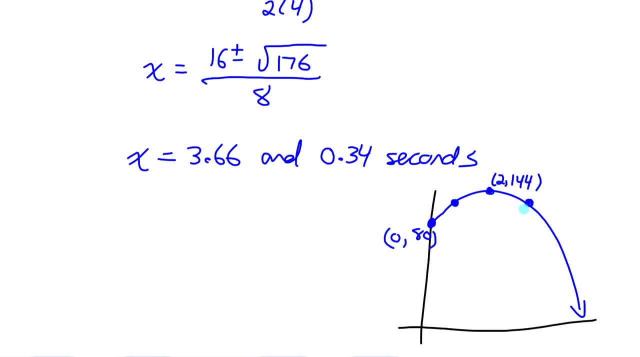 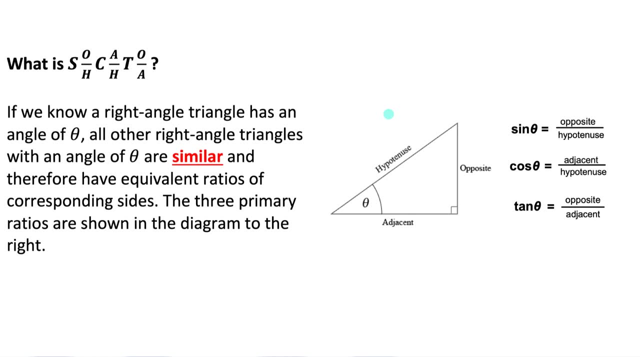 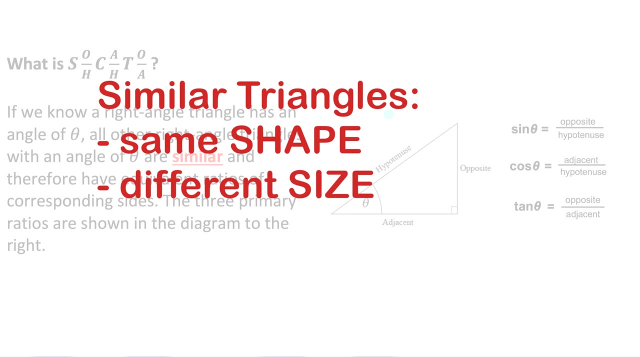 at two other times, at 0.34 and at 3.66, and that's what we found in this unit. you start off by looking at similar triangles, which are triangles that have the same shape but are different sizes. we know similar triangles have equivalent ratios of sides. 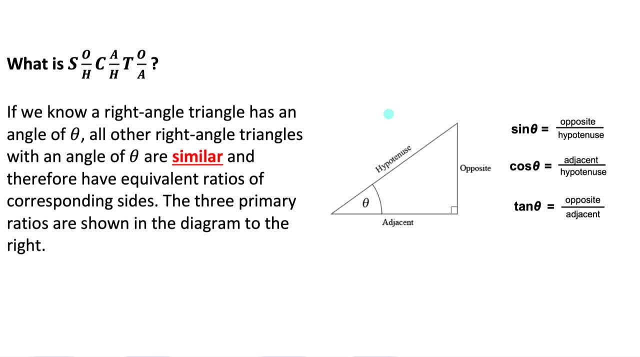 that naturally extends to right angle trigonometry and the acronym SOHCAHTOA, which tells us about ratios of sides in similar right angle triangles. we look at this right angle triangle here. we know that if a right angle triangle has a reference angle 0.01 from the right-angle triangle, we know that if a right-angle triangle has a reference angle, 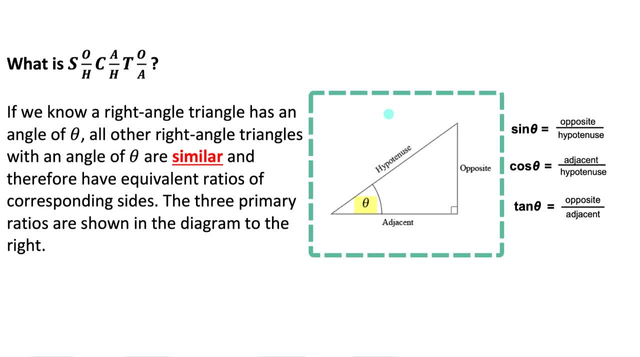 of theta. all other right angle triangles with that same angle theta are similar. they're the same shape but they may be different sizes. but because they're similar we know they have equivalent ratios of corresponding sides. since a triangle has three sides, there's three different pairs we could make from those three sides. we could pair up opposite and hypotenuse to get a. 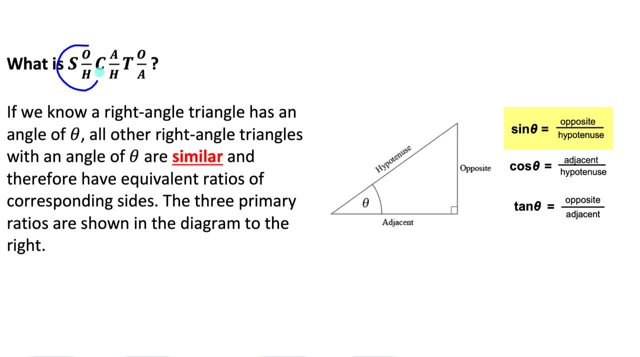 ratio and we call that ratio sine. that's where so comes from. sine of an angle equals opposite over hypotenuse. if we pair up the adjacent and hypotenuse, we call that ratio cosine. cosine of angle is adjacent over hypotenuse and tan of an angle is opposite over adjacent and the sides. 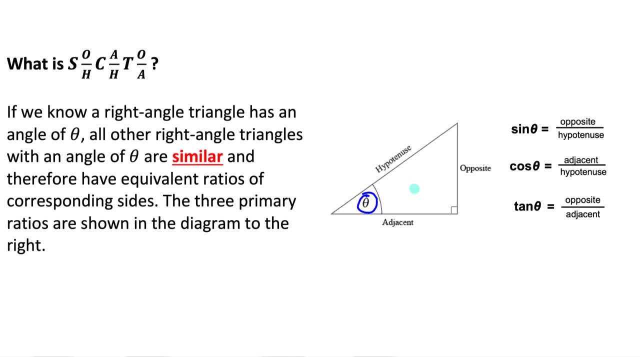 are being labeled from this reference angle, theta. so of course, opposite from that would be that side adjacent means right beside it, which is right there, and the hypotenuse is always across from the right angle. so here's a diagram just illustrating that. notice this right angle. 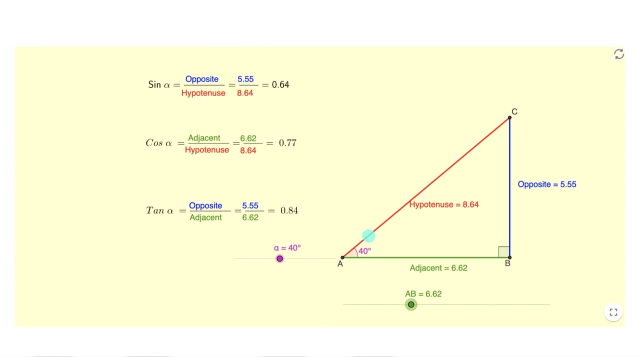 triangle. i have the sine, cos and tan ratios being calculated for this 40 degree angle. notice if i keep the shape of this the same. so keep that 90 degree angle and that 40 degree reference angle, but change the size of this triangle. notice that these three ratios are all going to stay exactly the same. so, even though the size of 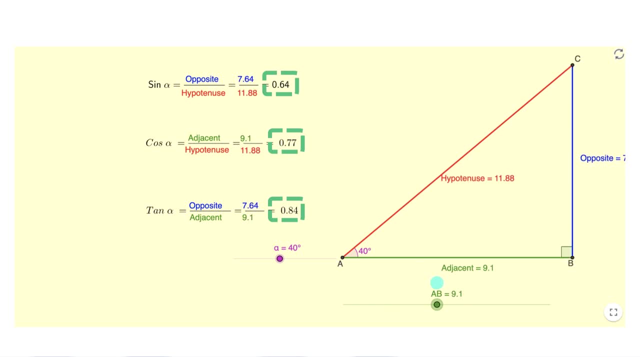 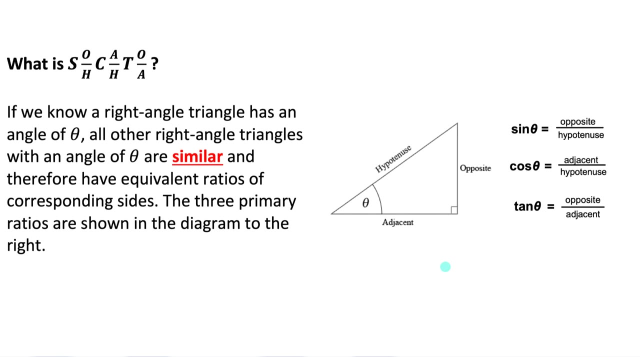 the triangle changes because all of these triangles are similar, their ratios stay the same and your calculator has the ratios programmed in. so sohcahtoa is used for right angle triangles. so let's do a couple questions where we're going to have to solve for angles or sides in right angle. 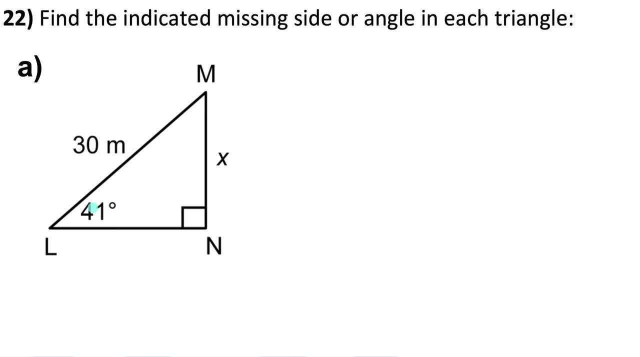 triangles. so i've got this right angle triangle. here i see a reference angle of 41 degrees and it's asking me to solve for the indicated side, indicated by x. so i need the length of side x and i know this side here. so from the 41 degree angle i want the side that is opposite to it. 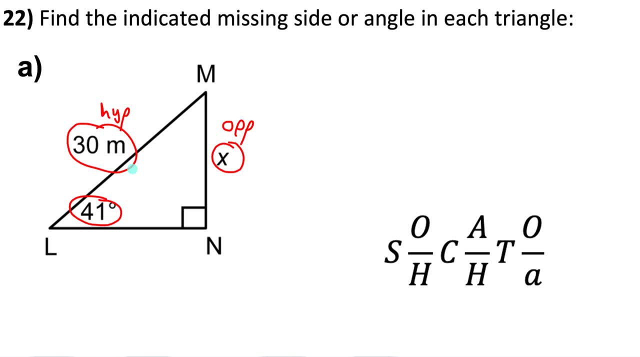 and i know the hypotenuse. so what ratio has opposite and hypotenuse, that's sine. so i know sine of the 41 degree angle would equal the opposite side, which we have called x, over the hypotenuse, which is 30. and then we'll just isolate x to solve for it by multiplying the 30. 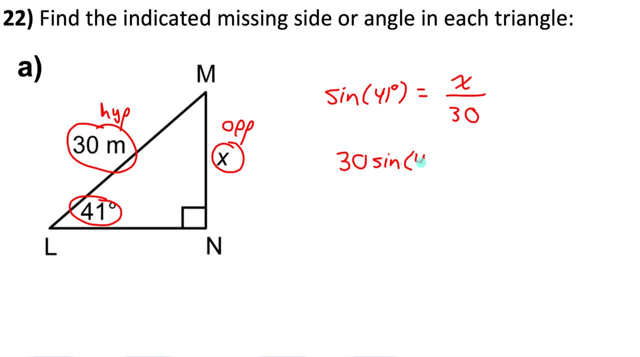 over. so 30 multiplied by sine of 41 degrees equals x, and if we evaluate that 30 times sine 41- making sure your calculator is in degree mode- we'll get an approximate answer for the length of side x, and it's about 19.68, and our units for this are meters. part b: once again we have a right angle triangle. where we're looking for a side length, so we can use sohcahtoa. so we're going to use a side length for the right angle triangle, where we're looking for a side length, so we can use sohcahtoa. so we can use sohcahtoa. 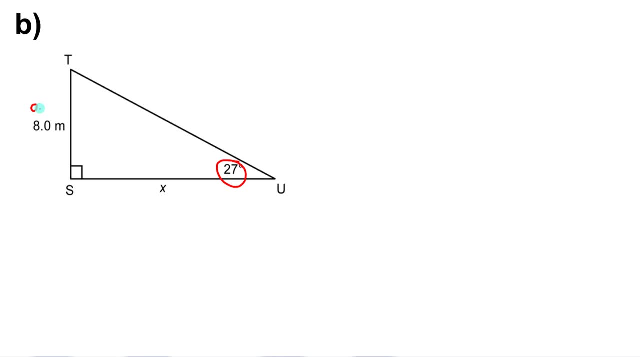 here's our reference angle. from that reference angle we know the opposite side and we are looking for the adjacent side. the ratio that has opposite and adjacent is tan. so i know tan from the reference angle would equal opposite, which is 8, over adjacent, which is x. now when? 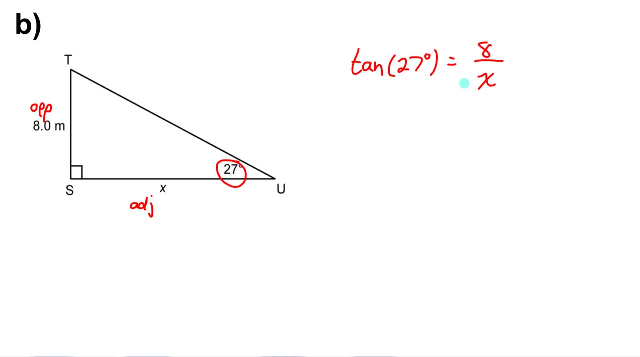 the variable is in the denominator of the ratio. when you do the algebra to isolate it, really what happens is the x and the tan 27 just switch spots. so i get x equals 8 divided by tan of 27 degrees and i can get my approximate value for that by typing in on my calculator and: 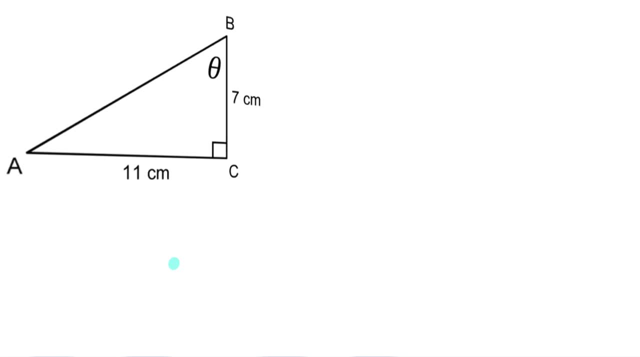 i get 15.7 meters, this one. we're looking for an angle. when we have a right triangle and we know two sides and we want an angle, we actually end up using inverse trig ratios. let me show you so: from the angle we want, we know the opposite side and we know the adjacent side. 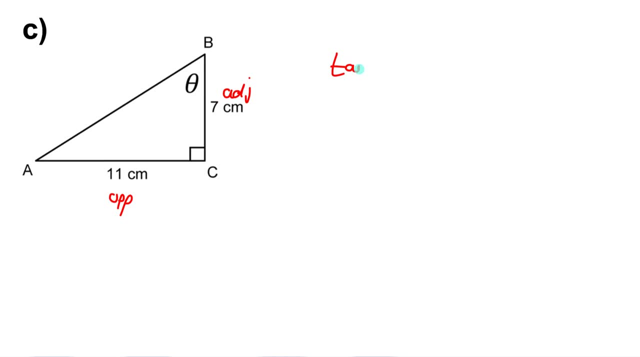 so the ratio that has opposite and adjacent is tan. so i know tan of that angle would equal opposite 11 over adjacent 7. to get the angle i actually have to do inverse tan. so theta is equal to inverse tan, which we denote as tan with that negative 1 looking exponent thing. but it's not. 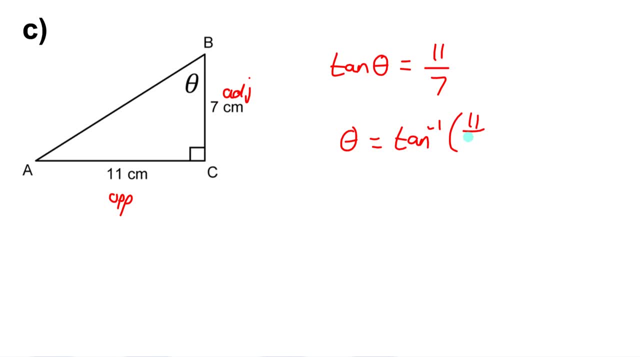 actually an exponent just means inverse tan of the ratio 11 over 7, and so if we evaluate this inverse tan of 11 over 7, when you use inverse tan, the calculator knows your input is the ratio and it's going to output the angle. we do that, we'll get an angle of about 57.53 degrees if we round. 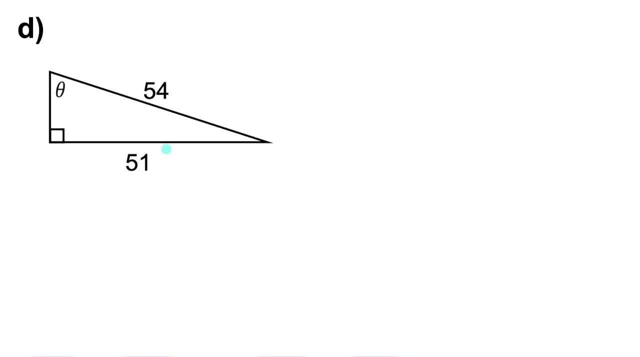 it to two decimal places. let's try another one like that once again, a right angle triangle. we know two sides. we're looking for an angle. so from the angle we want, we know the opposite side and the hypotenuse. the ratio that has opposite and hypotenuse is sine. so i know sine from that. 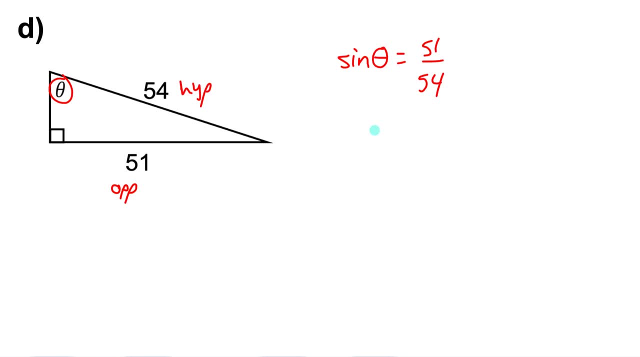 angle would equal 51 over 54 and when we want the angle and we know the ratio, we do F point 1 to the left first, we do F 2 to the right and if they う is equal to F 3 to the right. 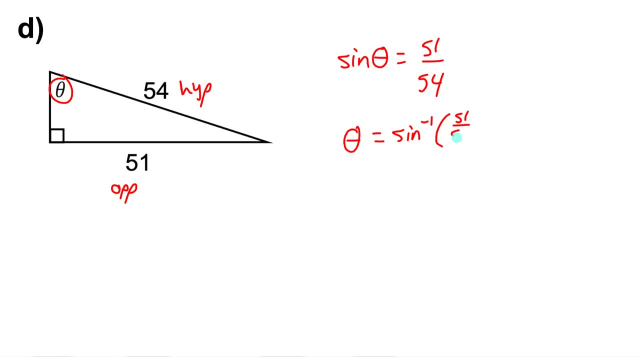 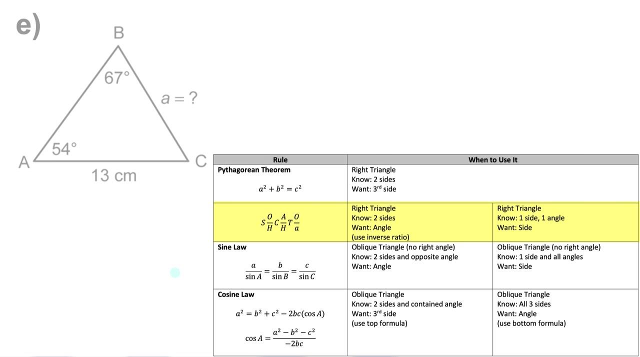 inverse sine of the ratio, and the calculator will output to us the angle that has that ratio, and it'll be about 70.81 degrees. Let's move on to non-right angle trigonometry. So after you learned about SOHCAHTOA, you would have then learned about two laws that work for calculating. 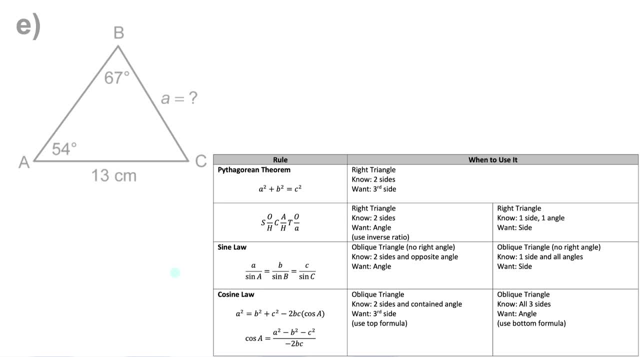 sides and angles of non-right angle triangles, called oblique triangles, and you would have learned about sine law and cosine law. Now, sine law and cosine law also would have worked for these first four, but SOHCAHTOA is so much quicker that if you have a right triangle, you do SOHCAHTOA. 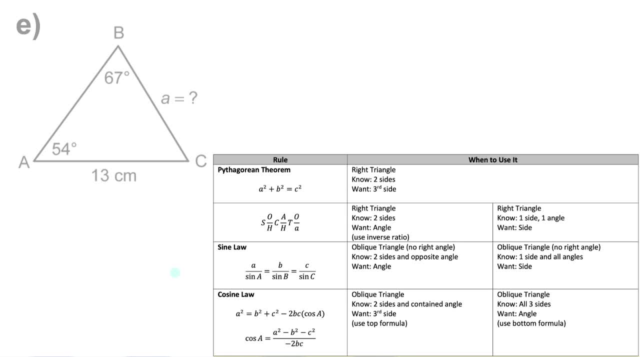 If you have a non-right triangle, SOHCAHTOA does not work. You have to use sine law and cosine law. So depending on what you're given and what you're looking for, you decide what to use. So for this question, we know two angles and one side of the triangle, which means we're going to use sine law. 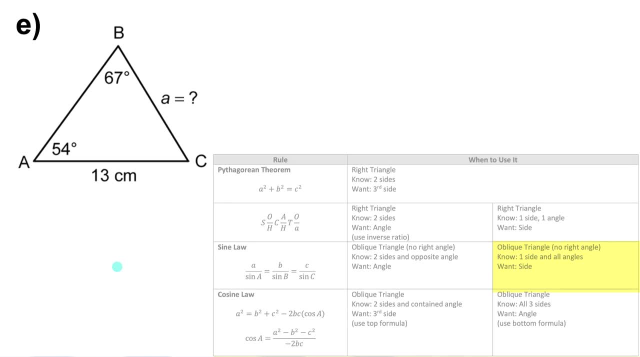 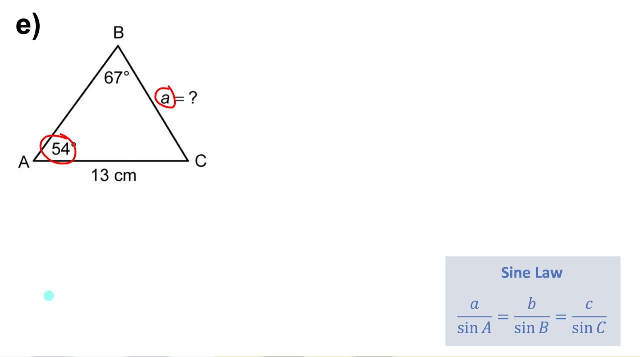 to find the other side. We're looking for side a, which is of course a cross from angle. a Sine law tells us that the ratio of a side to the sine of its opposite angle is equal for each of the sides in its corresponding opposite angle. So I know that a over sine of its opposite angle 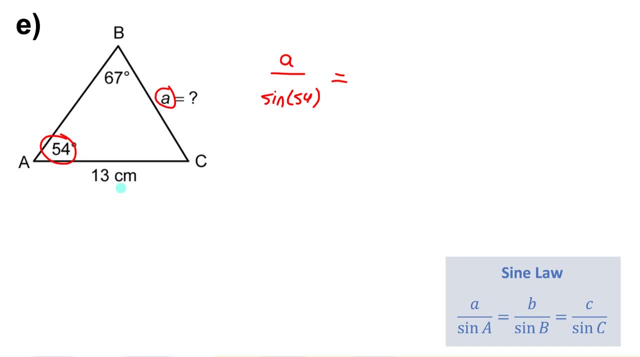 54 would be equal to 13 divided by sine of its opposite angle, 67. So based on this, I can now- I now have an equation with one variable. I can just multiply this sine 54 to the other side and I then have a isolated, So 13 times. 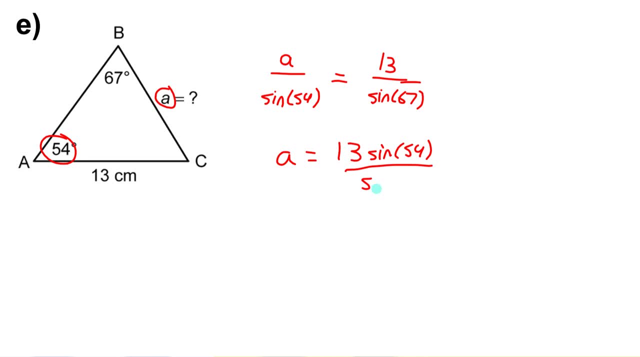 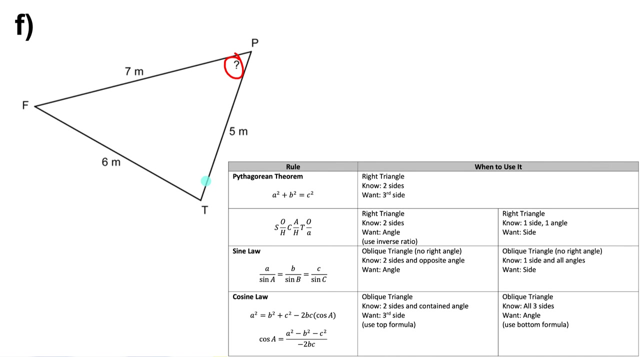 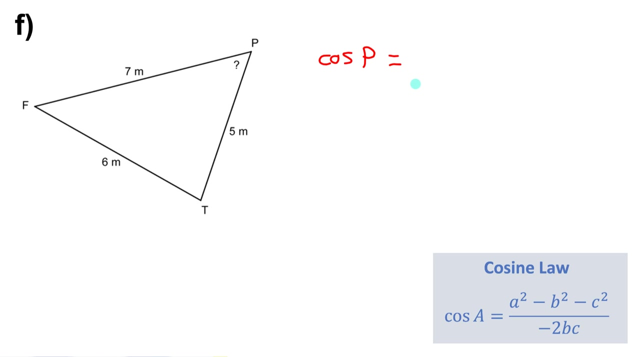 sine 54 over sine 67. if I evaluate this, I'll get an approximate length for side a which is 11.43 centimeters. Part f: if we're looking for an angle and we know all three sides, we can actually use cosine law for this. So if I want cosine of angle p, it's equal to we do the square of the side. 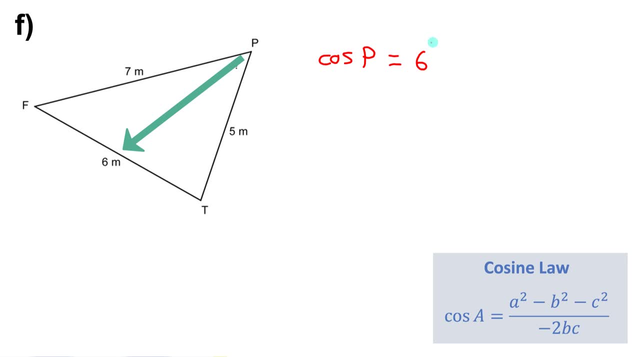 opposite from the angle we want. so 6 squared Minus the squares of the other two sides. so minus 7 squared minus 5 squared. The order of the 7 and the 5 doesn't matter, but the 6 definitely has to be first. The first one is the one across. 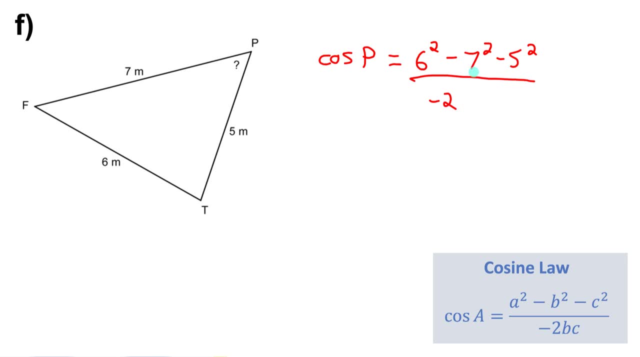 from the angle we want, Divided by negative, 2 times the second two sides, the 7 and the 5.. Ok, so we have the ratio. maybe we want to simplify this ratio. so 6 squared minus 7 squared minus 5 squared is: 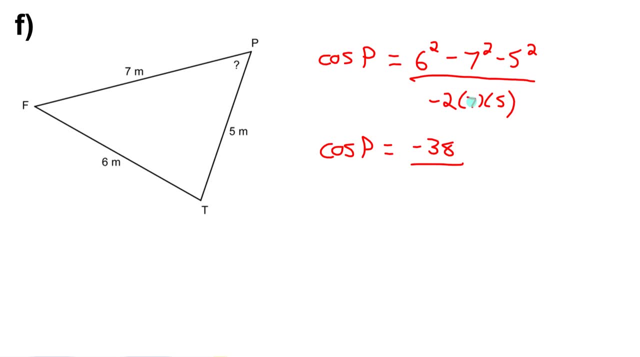 negative 38. And then negative 2 times 7 times 5 is negative 70. so I have the ratio and I want the angle. I know to get the angle. if I want angle P, I can do inverse cosine of the ratio and I'll just cancel out those two negatives and 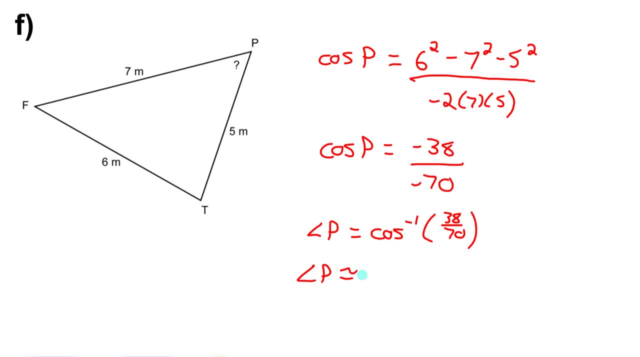 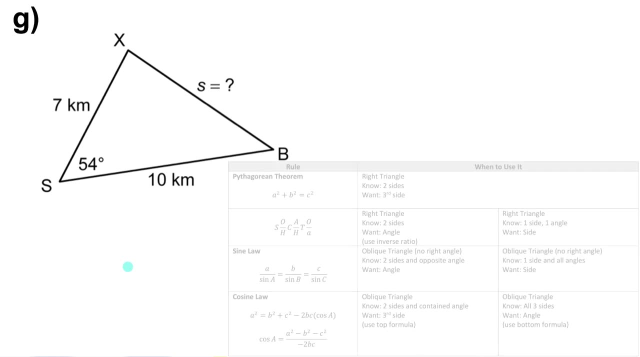 just write 38 over 70, so angle P. if I do inverse cos of that ratio, I get 57.12 degrees. and the last scenario you'll have is if you know two sides and the angle contained by those two sides, which means between the two sides you can find the side opposite from the contained angle. 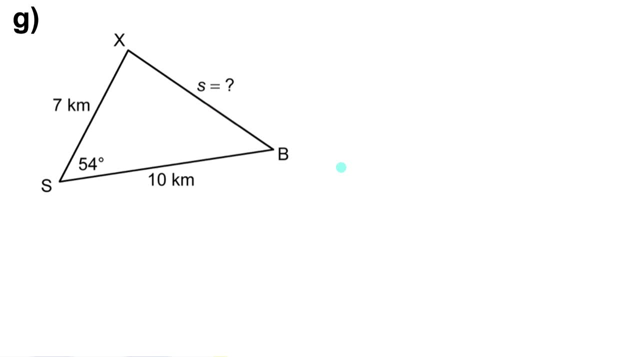 by doing cosine law, a rearranged version of cosine law compared to this one. we did to find the angle, but it's the same equation. so if I want this side s equation based on cosine law is: s squared equals the sum of the squares of the other two sides: 7 squared plus 10 squared.